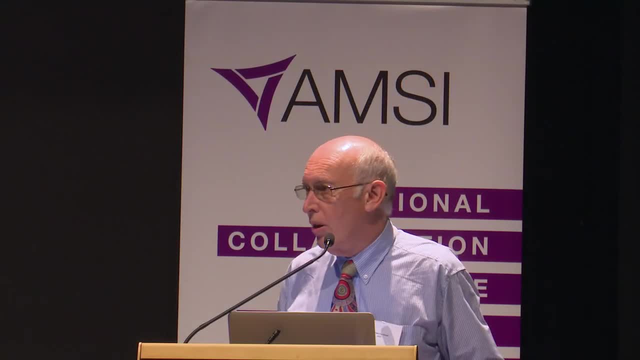 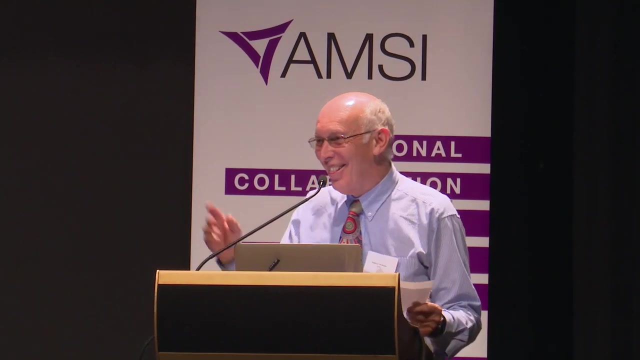 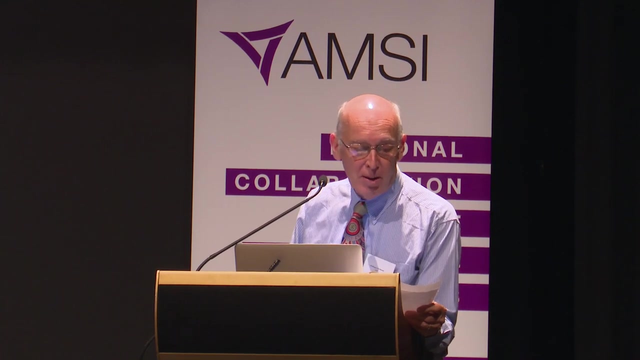 Good evening everyone. My name's Tim Brown and for the grand total of 13 working days I've been director of the Australian Mathematical Sciences Institute. Oh, thank you. Save your applause for something worthwhile, please. I would like to acknowledge the Bedigal people that are the traditional custodians of the land on which this meeting takes place. 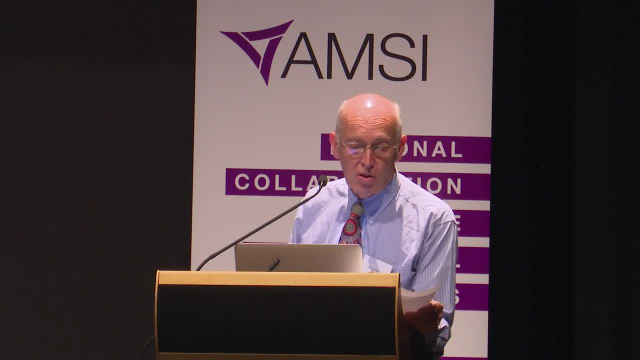 and I would also like to pay my respects to their elders, both past and present. AMSE has a very proud tradition of running a summer school, and this year we, I understand, have approximately 170 student participants and they're studying a very wide range of subjects. 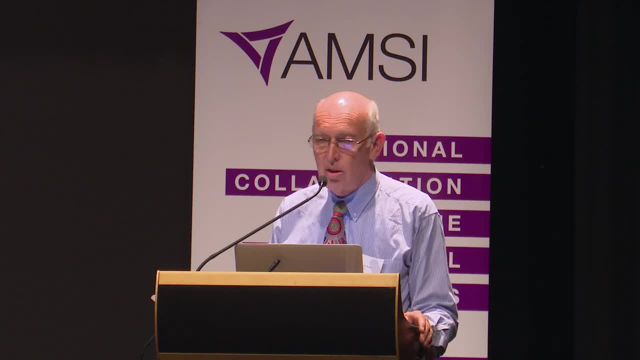 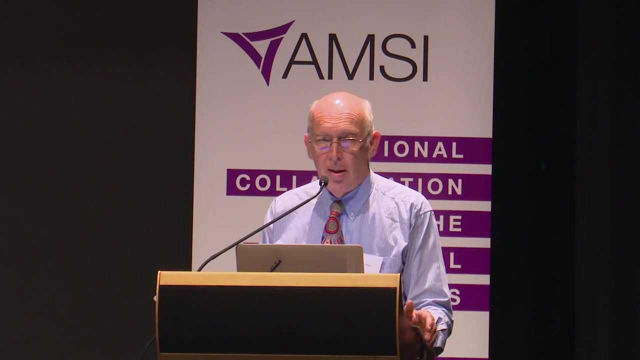 And I think that's really greatly to the credit of the mathematical sciences community that we're able to do this. It provides all of those students with a much richer mathematical education than they would otherwise get, and it's also a great opportunity for staff from the Australian Mathematical Sciences Institute. 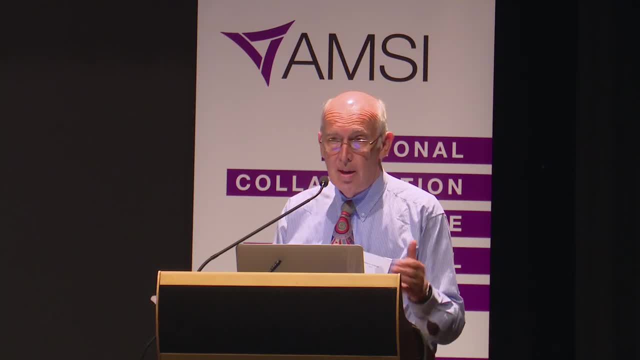 from the summer school host to be exposed to a much wider group of students than would otherwise be the case. Nevertheless, it is a bit tough both for the lecturers and the students to be giving up some of the time that perhaps would traditionally be a break for them. 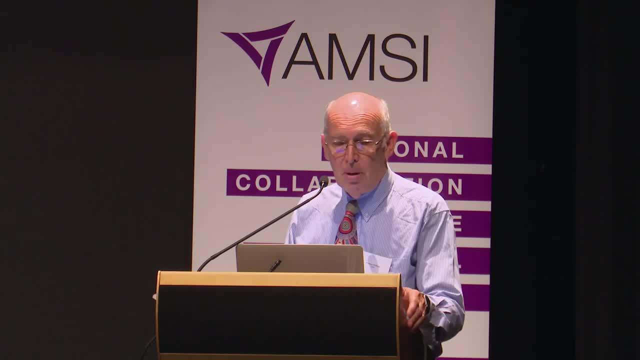 So I really wanted to give a very big thank you to all of you for this great summer school. Thank you, And I think the public lecture has been a wonderful tradition and, without any further ado, it gives me great pleasure to introduce one of the summer school lecturers who's been teaching mathematics of planet Earth. 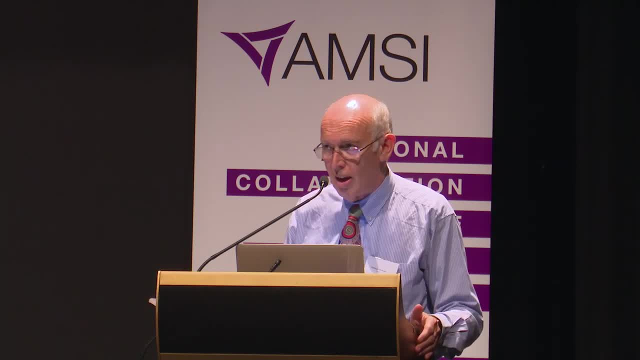 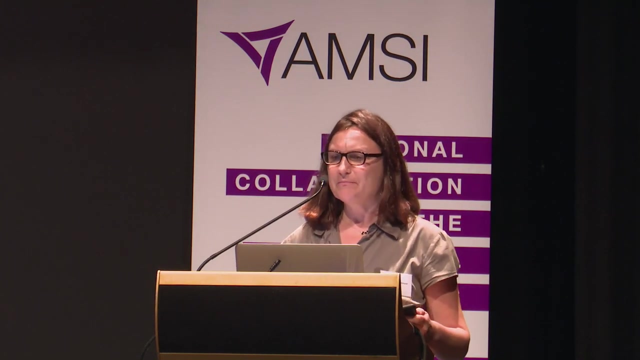 Associate Professor Lisa Alexander, who's going to introduce our speaker tonight. Thank you, Okay, thank you very much, Tim. As Tim said, I've had the pleasure of teaching on the AMSI summer school this year and UNSW has had the privilege of hosting it. 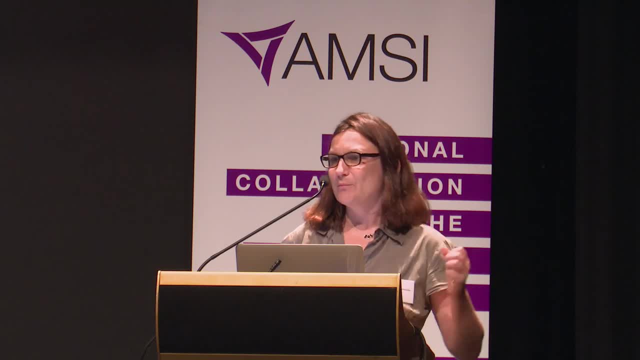 I'm always impressed by the number of students who come and their enthusiasm and how impressive they are, So thank you. I can see some of you in the audience, so that's really good. So before I introduce our invited speaker, I have an announcement to make. 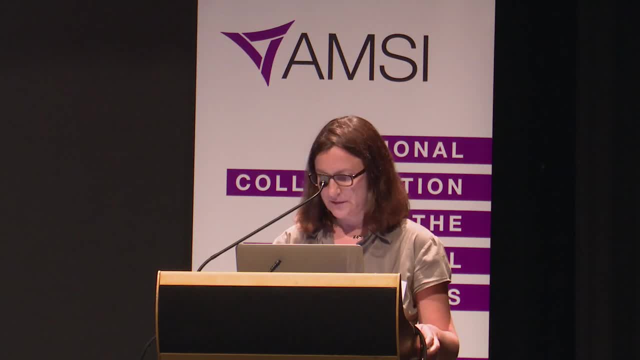 I've been asked to let you know that tonight's lecture will be filmed. We're going to try and minimise the footage of the audience, but if you have a problem with that, please let our event organisers know. Anna, are you here? 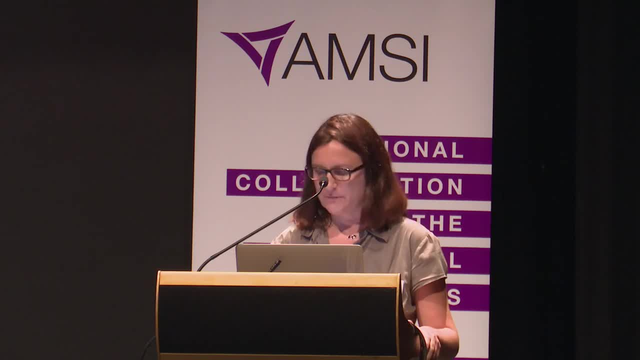 Over there if you have any issues with being filmed. So now it's my great pleasure to introduce our speaker, Dr Stephen Griffiths, who will be presenting the public lecture this evening. I hadn't actually met Steve- maybe somewhat surprisingly- until today. 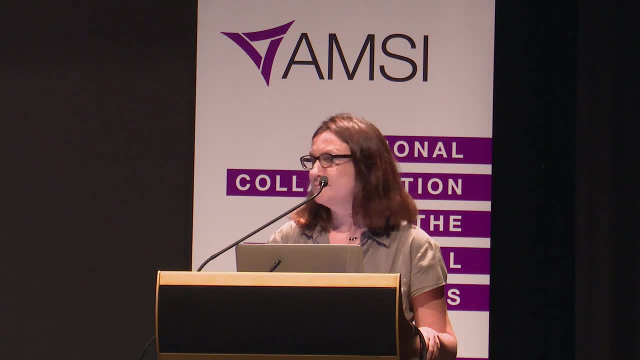 But I've- actually- not unsurprisingly- heard a lot about him, not just for the fact that he's academically excellent, but also because he's well known for being very down to earth, being very collegial and being a good mentor, particularly to students. 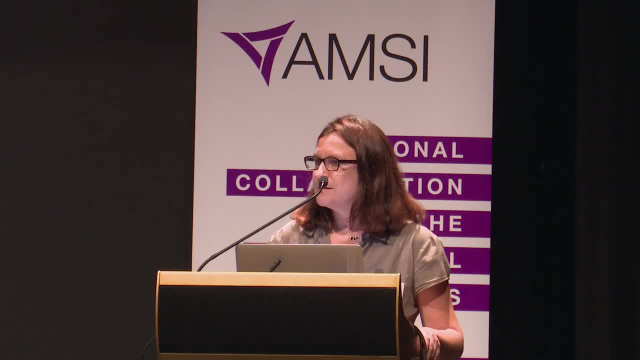 Dr Griffiths got his PhD in 1993 in theoretical physics. He's currently a lecturer at the Atmospheric and Oceanic Sciences Programme at Princeton University, in addition to holding previous and current positions at NOAA's Geophysical Fluid Dynamics Laboratory, And that's also included visiting scientist positions to places such as the National Centre for Atmospheric Research in Boulder. 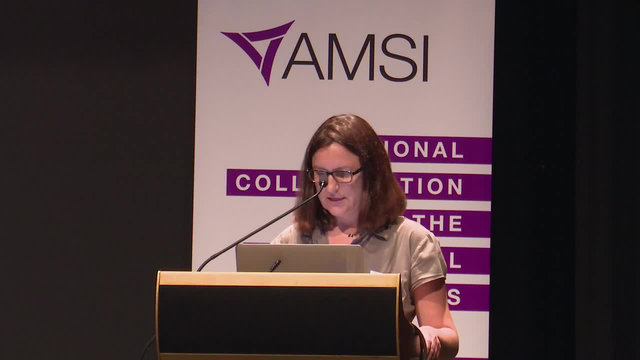 and also at CSIRO in Hobart, So he's very well travelled and he has a very good network of colleagues. So Stephen's research is concerned with elements of ocean fluid mechanics and the role of ocean in the earth climate system. Examples of his particular research topic in recent years have been on Atlantic and Southern Ocean dynamics. 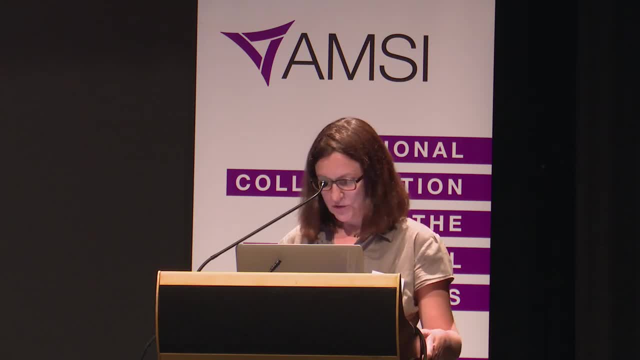 global and regional sea level, variability and change, transport of matter and energy by transient mesoscale and submesoscale eddies, and algorithms for ocean circulation models. So he has a wide range of research that he's interested in. He also aims, as I said, to foster fundamental understanding of physical concepts and their creative use in describing observed and simulated ocean phenomenon. 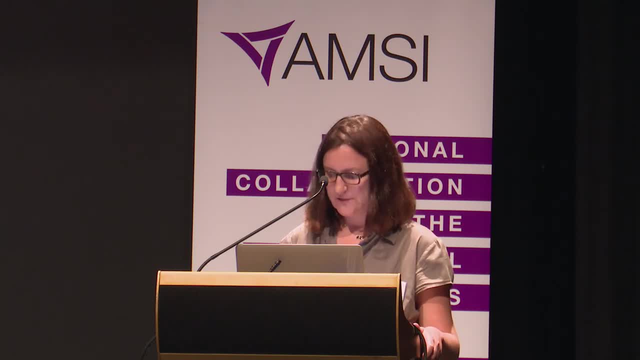 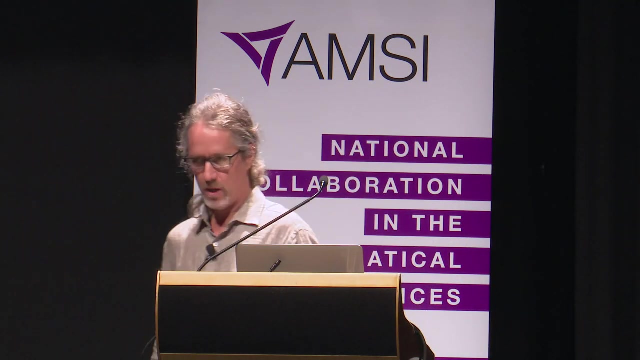 So tonight he's going to be talking to us on a maths physics view of ocean circulation. So, without further ado, please welcome Dr Stephen Griffiths to the stage. Thank you, So thank you. Thank you, Lisa. Thanks for the organisers. 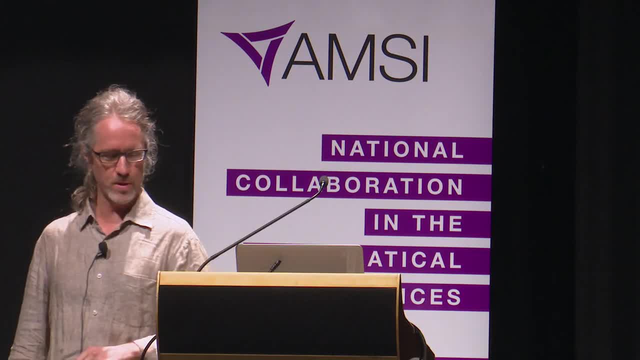 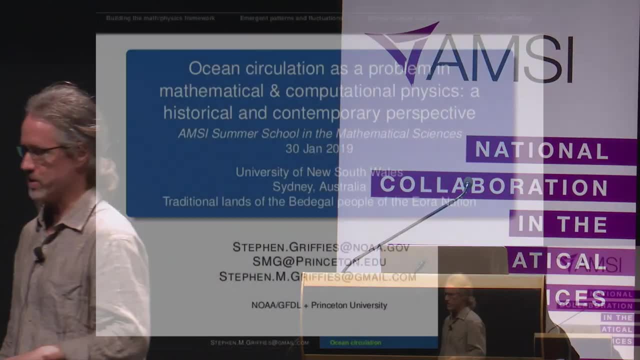 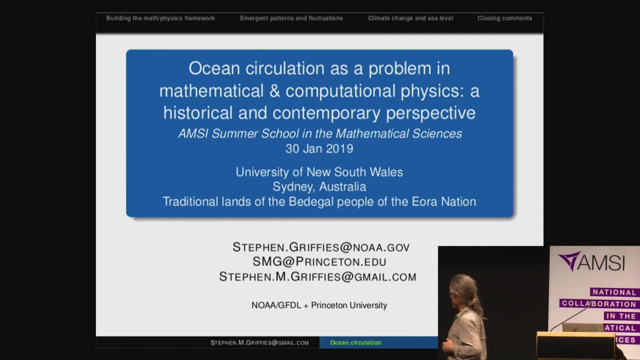 Thanks for especially the students for showing up in this summertime, Hot summertime here in Sydney. I left five degree Fahrenheit in Princeton before I came here, So it's a nice break. So I changed the title a little bit, but it's still very similar. 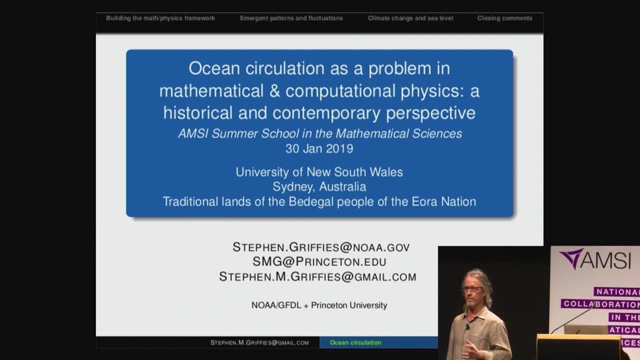 Ocean circulation is a problem in mathematical and computational physics. That's kind of my focus and it's going to be historical, very selective overview with a contemporary perspective And again acknowledging the traditional owners of this land And acknowledging that I have three email addresses because of certain things that have been going on in the last 35 days or so in the US. 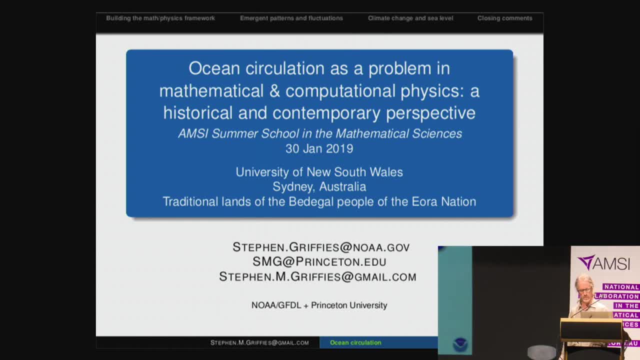 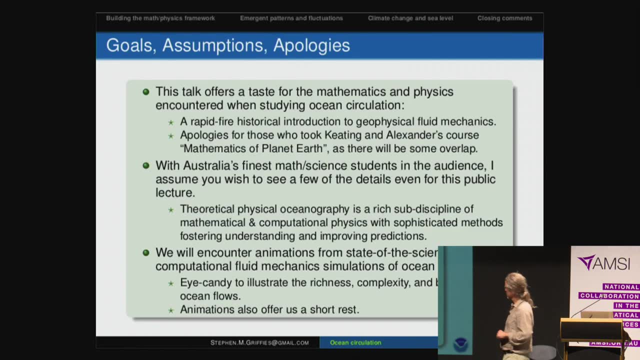 which made it impossible for me to be official, But now I'm official again. So for those that know what I'm talking about, that's it. That's the extent of the politics. This talk offers a taste of the mathematics and physics encountered in what we do for ocean circulation modelling. 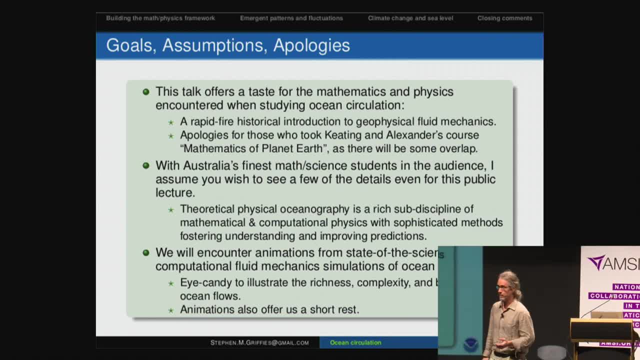 And ocean circulation, physics and oceanography in general. I'll give a rapid-fire historical overview of geophysical fluid mechanics, which is the science, the fundamental science of what we do, And apologies for those who took the mathematics of the Earth, planet, Earth course, because there's going to be some overlap. 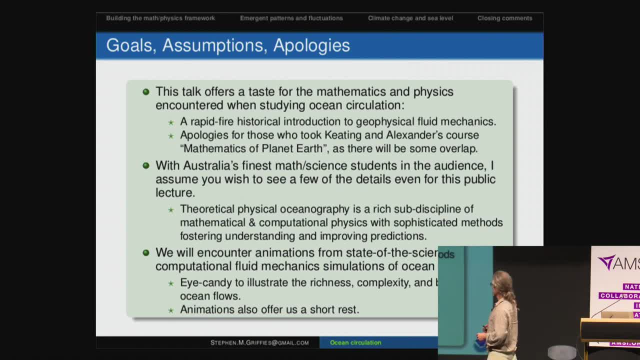 But you'll probably hear it in a different way With some of the finest students in Australia's math and science. I hope that you will not be bothered by some mathematical symbols. Theoretical physical oceanography is a rich sub-discipline of physics. 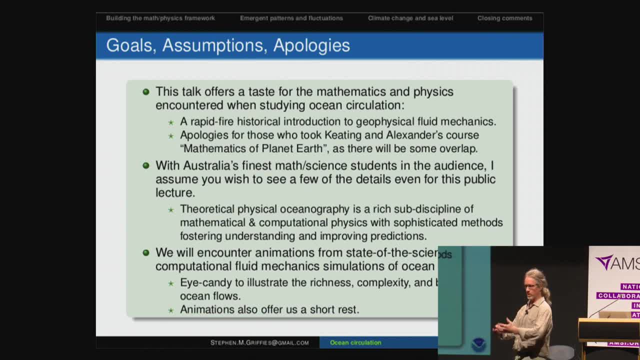 Mathematical and computational physics in particular. There's observational elements to what we do in oceanography as well, but I'm going to focus more on the theoretical and computational side. We will also encounter, for breaks and also for stimulus, and hopefully some whetting of appetite, some animations from high-tech computer simulations. 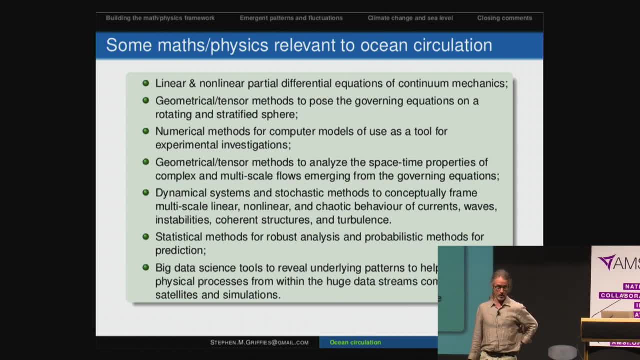 So what are the physical and Well, what are the mathematical areas That we deal with in this subject? So there's just a very incomplete list here, Going from linear and nonlinear partial differential equations, Geometrical and tensor methods to formulate those equations on a rotating sphere. 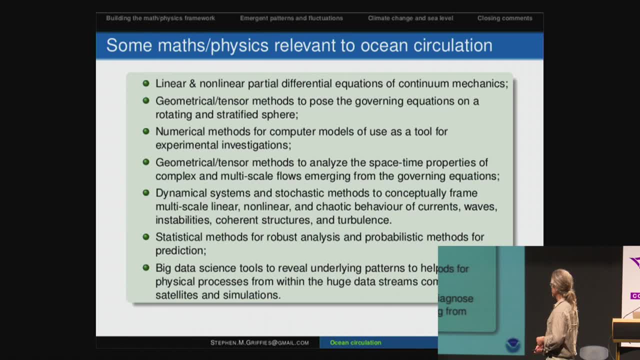 Also to do some numerical methods You need For computer models. you need numerical methods, numerical analysis, And again you need the geometrical and tensor methods to analyze the structure of the flow. This is complicated fluid dynamics that we're dealing with. 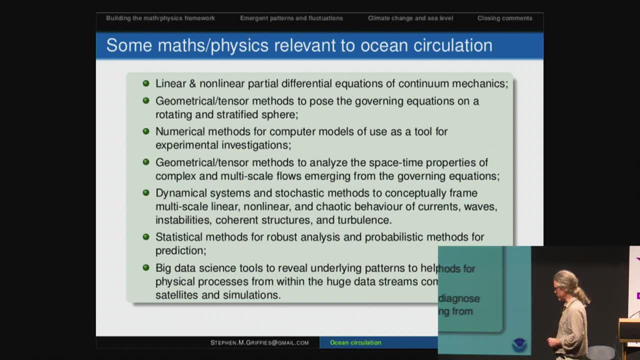 And you have some in a stratified flow, And so there's lots of different features, geometrical features, that having some fundamental math tools in your hands will help you a lot. Dynamical systems and stochastic methods are very useful for understanding lots of the fluctuating variability that we see. 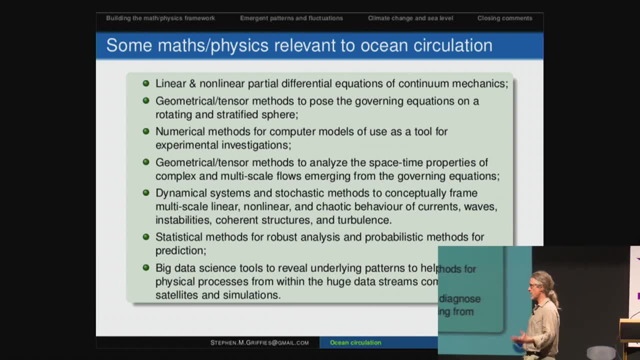 And statistical methods for robust analysis And probabilistic methods for prediction. A lot of what we do at my laboratory deals with models that we use to predict hurricanes Or tropical cyclones, The weather and different fluctuations in the ocean, And big data science tools to reveal the underlying patterns. 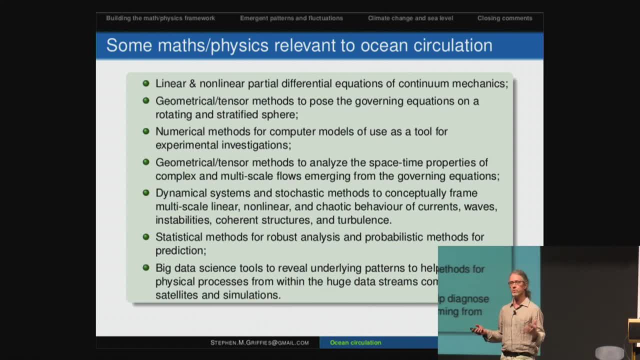 And to help diagnose physical processes within huge data streams. We're talking petabytes of data that we're starting to put out with computer simulations And archives of data And satellites as well. So those of you who have interest in some math and the use of that math will find a rich home in the earth sciences. 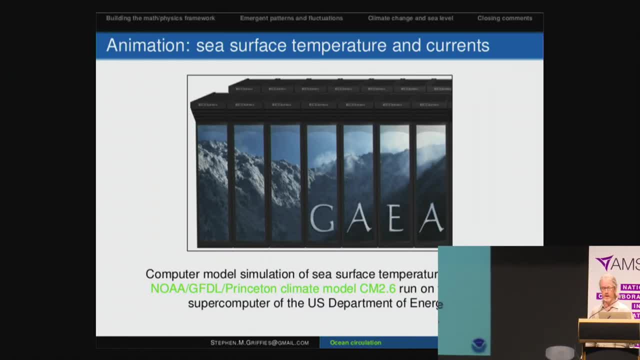 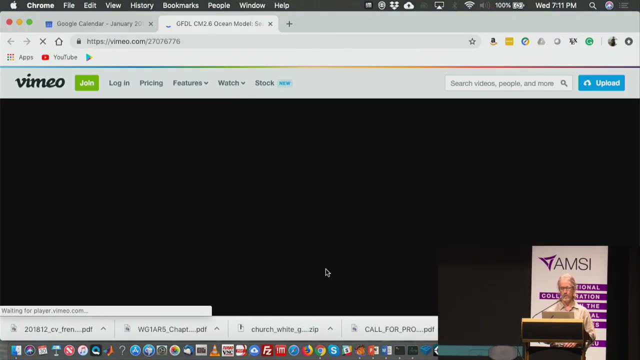 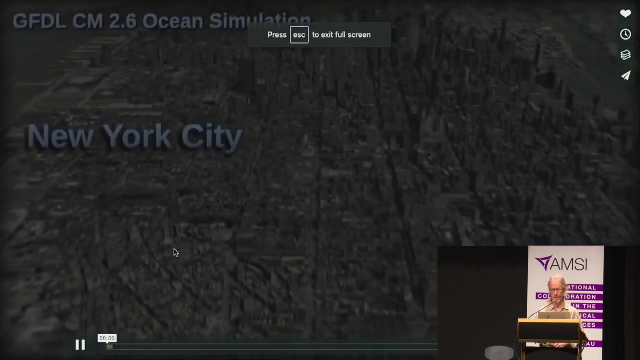 And, in particular, oceanography. So to give you an early wetting of your appetite, I'm going to jump between. Going through the internet, You can find these. This is a Vimeo video Of a computer simulation that was created at GFDL a few years ago. 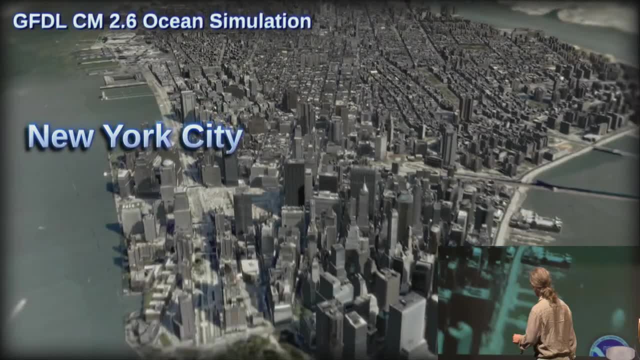 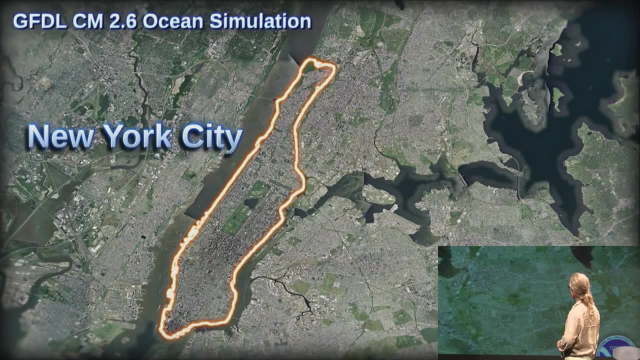 Starting from giving you a sense for the grid size, I have a view of New York City Which is very close to where I live. I was there just a few days ago: Manhattan Island, And this is a grid box, A tenth by a tenth degree. 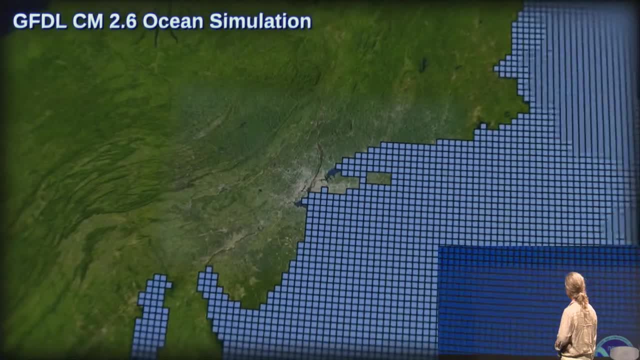 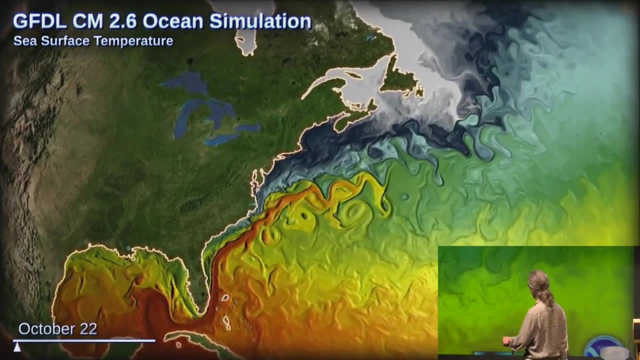 And now we're going to pan out and see a bunch of those grid boxes And then we're going to start to see some ocean circulation features And this is one of my favorite features off the east coast of the US. Is this jet of water coming up? 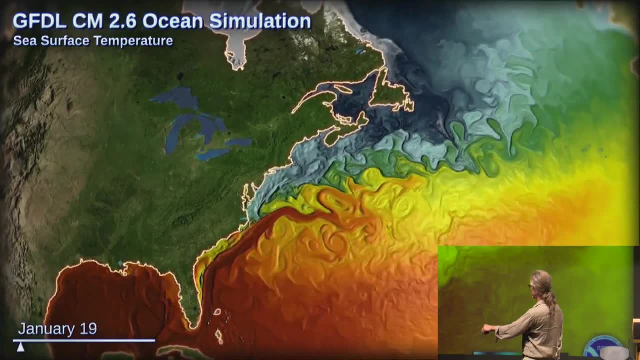 It's the Gulf Stream. You can't see down here, but the days There's a clock down here, So we're moving pretty fast. You can't go out in the ocean and see this by eye right away. This is We're going. 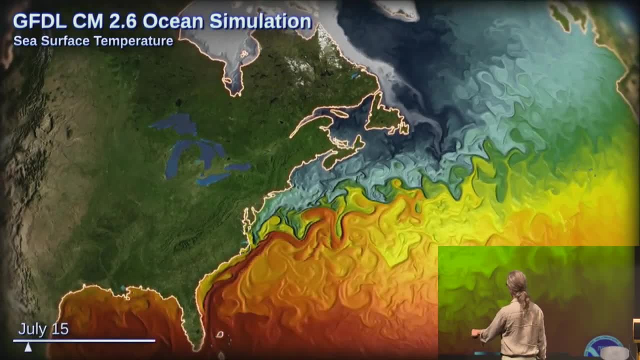 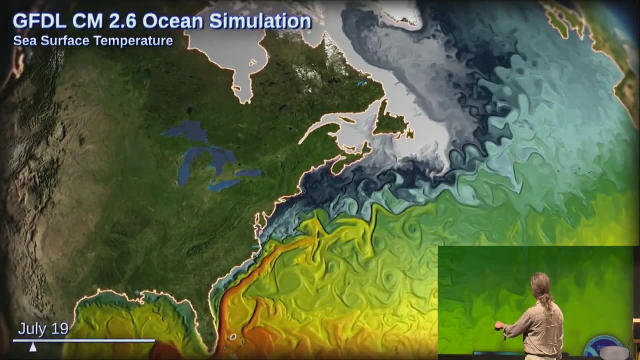 These are fast moving along here. So the warm temperatures, So the red is warm And, as you see the seasonal cycle, It starts to cool a little bit And the jets go unstable In a type of instability known as baroclinic. 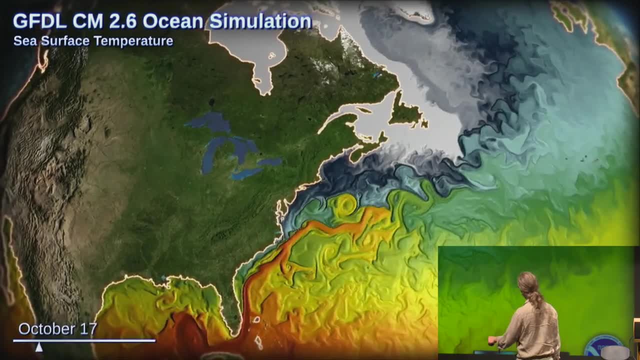 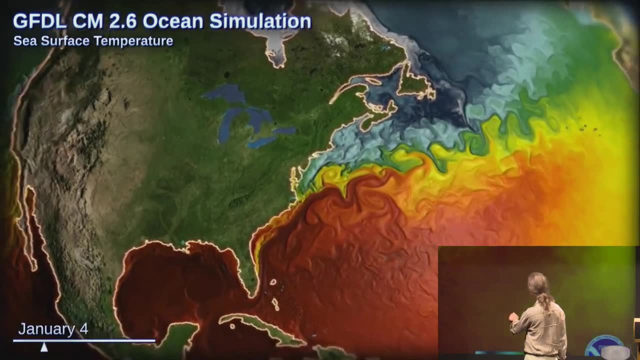 And barotropic instability, And that warm water moves northward, Into the North Atlantic, Bring in lots of warmth, Especially over to the east side of the Atlantic, Into the Atlantic, Into northern Europe, And now we're going to move to the tropics. 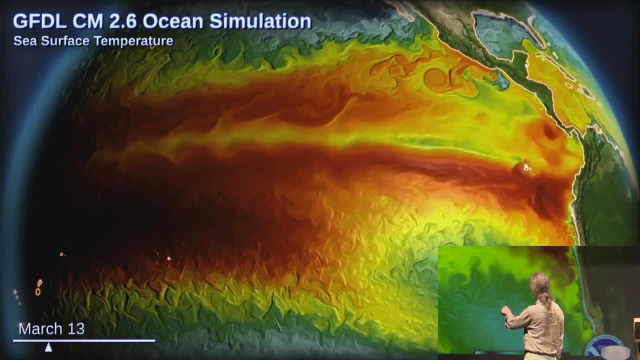 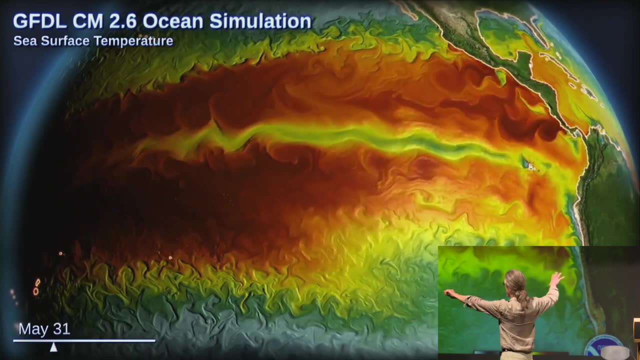 And see a very different looking dynamics here With these tropical instability waves And large amplitude, Large wave number Or large features As you go lower into the tropics. This feature right here is a Galapagos island Which is really fascinating. 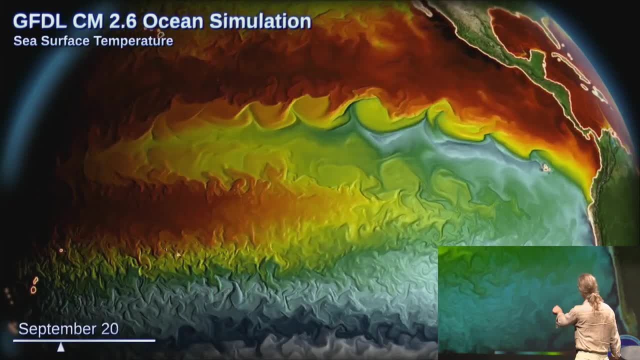 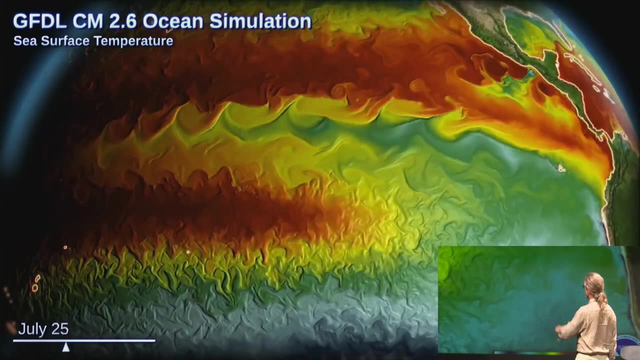 This little speck on the Right near the equator Creates a huge wake That you can see And it's a nice image that you see the smaller scales When you go to the higher latitudes Away from the equator. 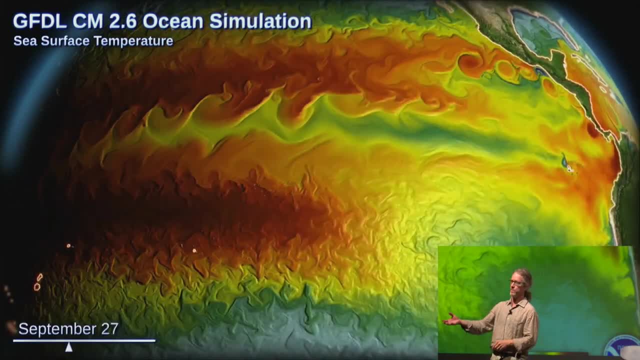 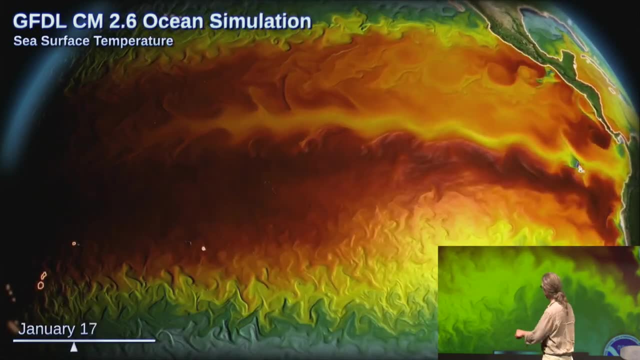 That's due to the rotation of the planet And the fact that with a rotating planet On a sphere, The Coriolis parameter, The Coriolis acceleration, Has a variation That's a function of the latitude And the scales of the motion, gets smaller. 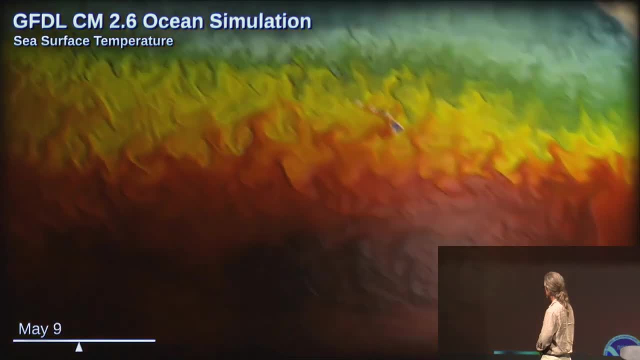 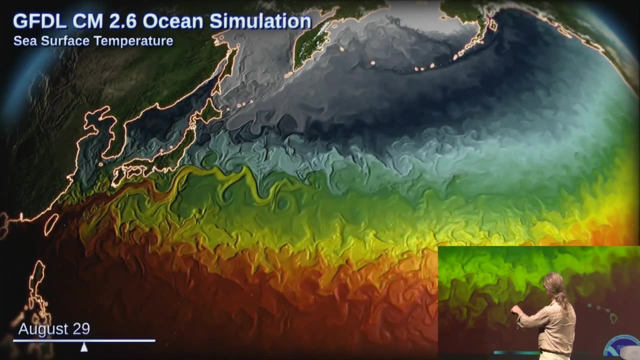 As you go to the higher latitudes Due to some basic geophysical fluid mechanics features. This is the Kirishio current Off the east coast of Japan, Moving out into the north Pacific. Very similar dynamics That what we saw over in the Gulf Stream. 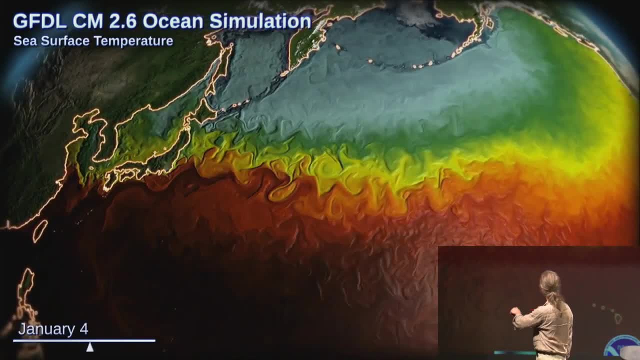 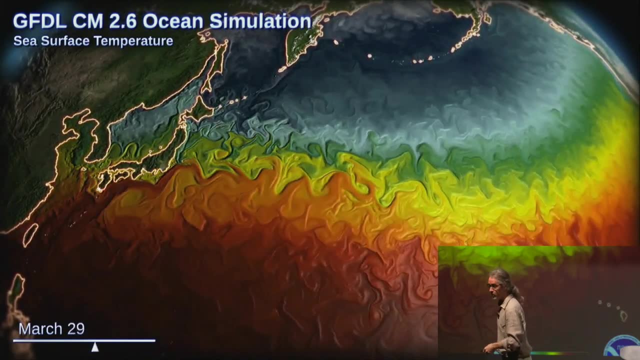 Just a few seconds ago And we're changing the temperature. I'm sorry, the temperature scale is down here. One other thing to note: You see some large fluctuations And that's because this is a coupled model. It's coupled to an atmosphere. 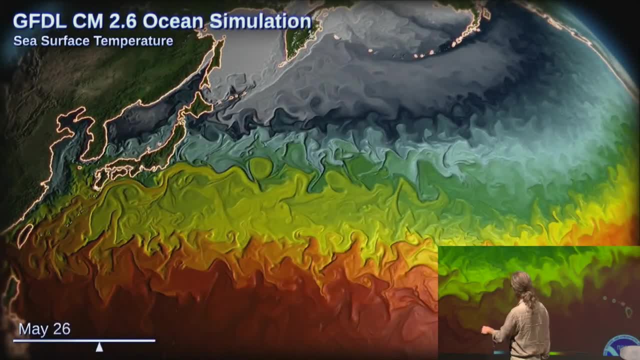 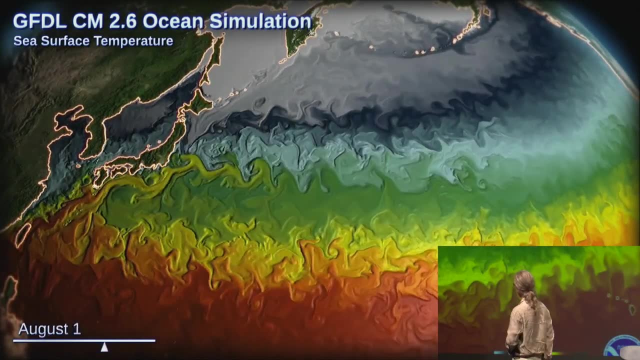 And so you have big seasonal patterns here, And every so often, If you're really good with your eyes, You'll see a tropical cyclone go through, And tropical cyclones suck up cold water from beneath And leave a wake of cold water in its path. 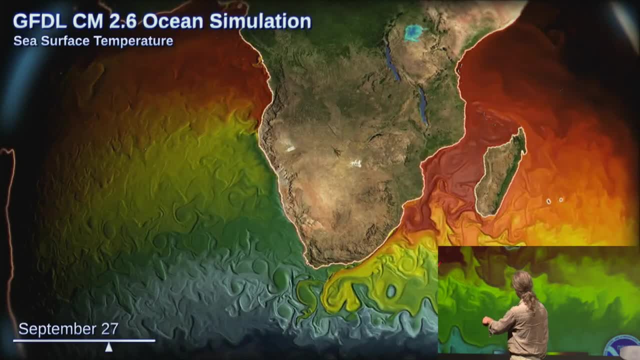 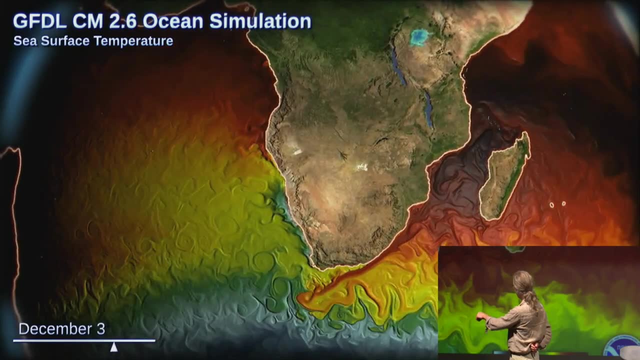 Now we go to South Africa And you see this current here Around the south of Cape Good Hope And that's the Agulhas current here And it breaks into these eddies And these whirling eddies that move into the South Atlantic. 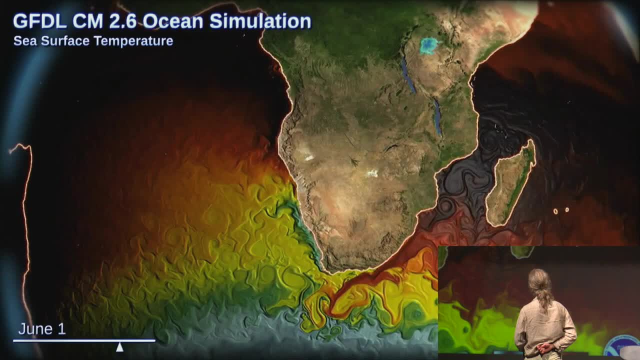 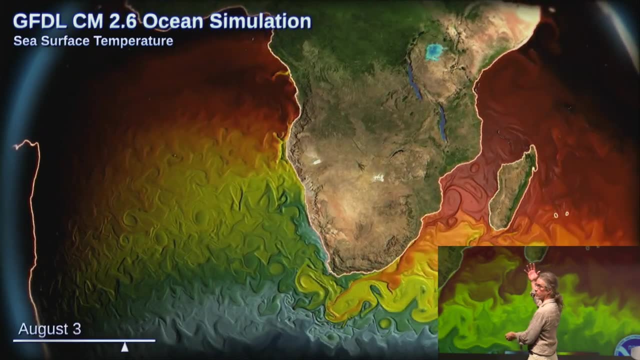 And these are called Agulhas eddies For good reason. That's part of the geography of where we're at And you see this cold water here That's driven by winds That are blowing along the coast And sucking up cold water. 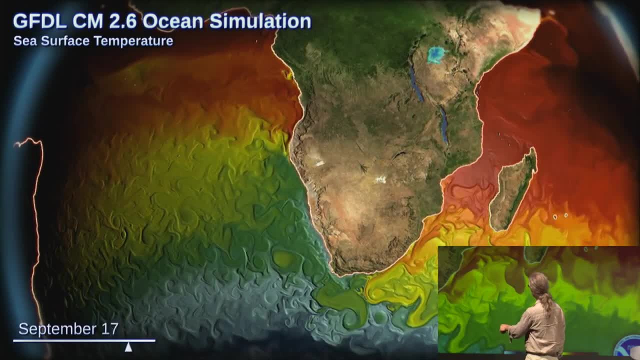 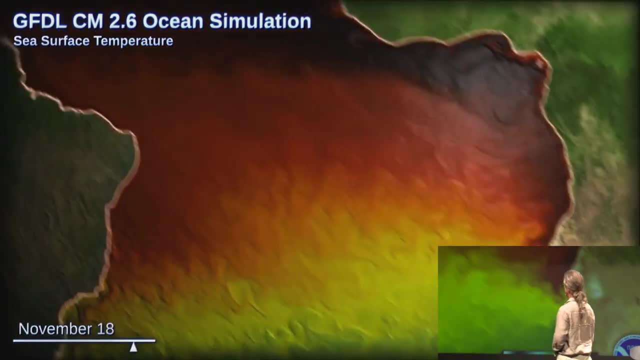 Due to a process known as Ekman suction. It's a very rich fishing zone down here. They have the nutrients that are sucked up by the winds. And now where are we going to go Back to the tropical Atlantic, Changing the color scale a little bit. 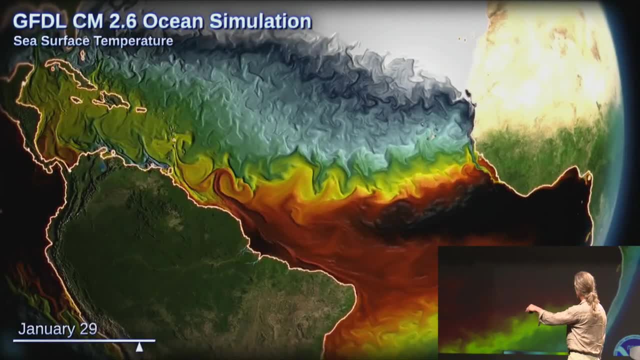 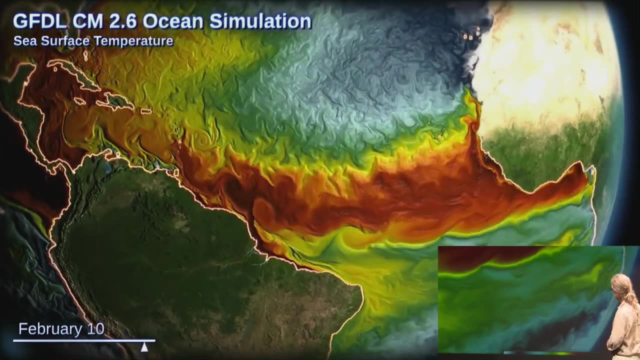 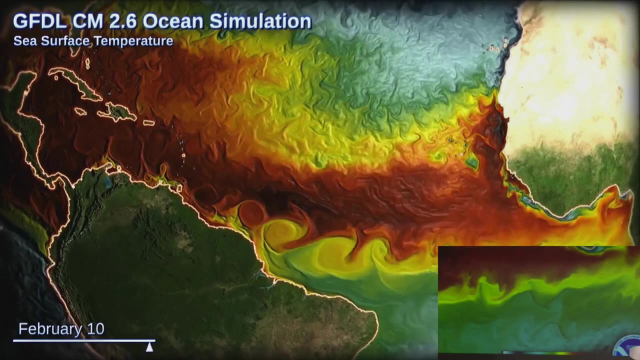 And seeing the Caribbean, The Brazil current moving up water Into the Caribbean islands here, And I think that's it. That was a big eddy there That might have been created by some local windburst. Anyway, This is a simulation in a climate model. 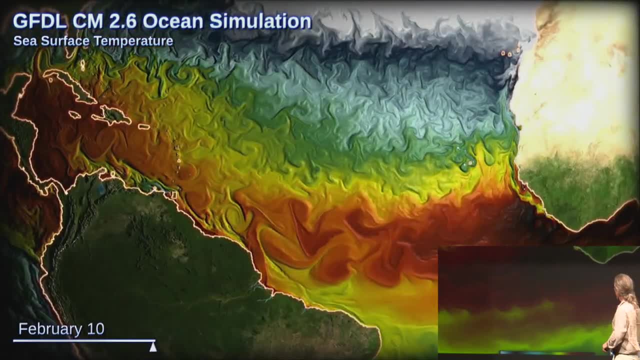 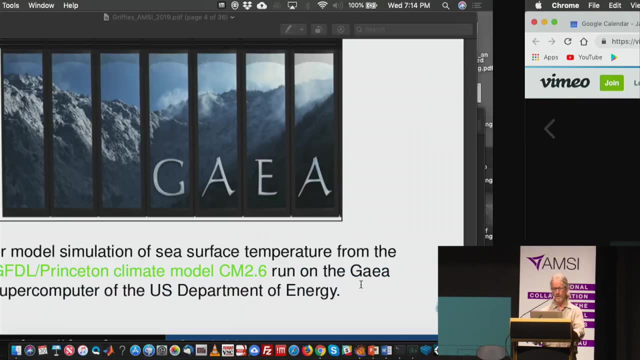 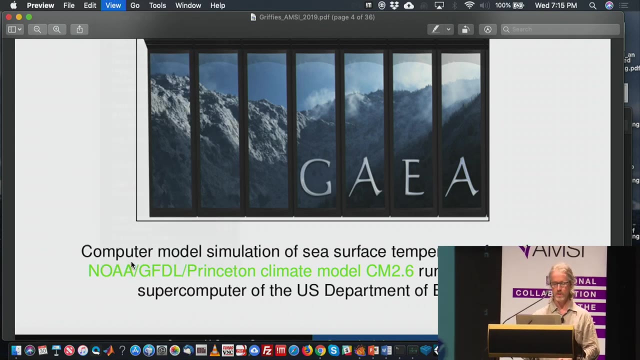 That is dear to my heart. It was a model that I helped build And it is still very much state of the science In climate modeling And it's something that I cannot get enough of Seeing those kind of images And those animations. 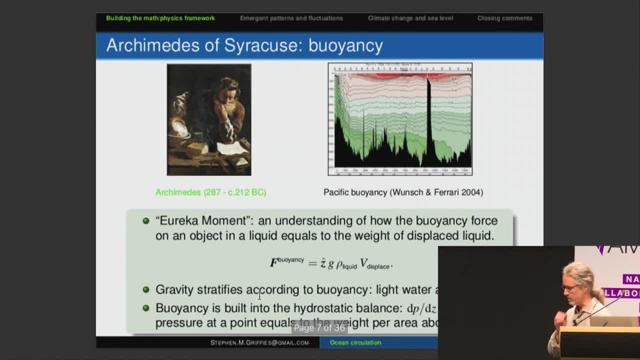 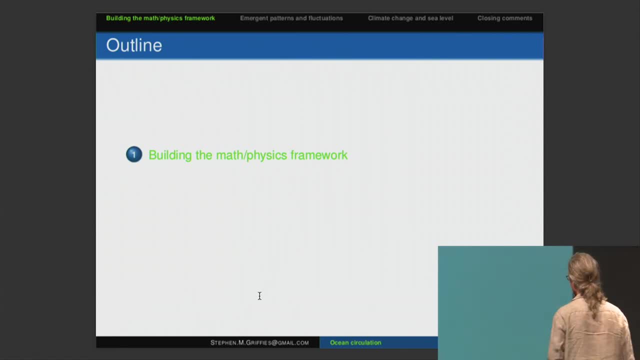 Because they are very inspiring And very useful scientifically As well as sort of a gee whiz, Eye candy sort of thing. So now I would like to step back a little bit And try to help you get a sense For some of the mathematical and physical ideas. 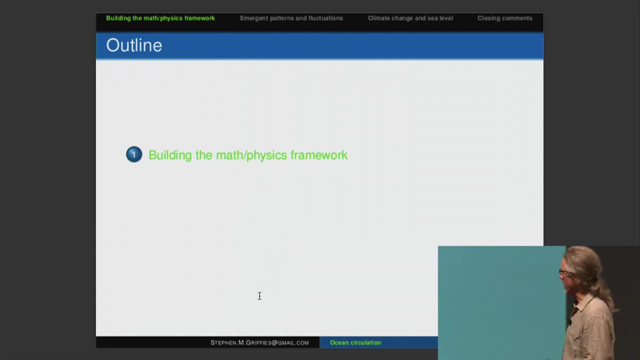 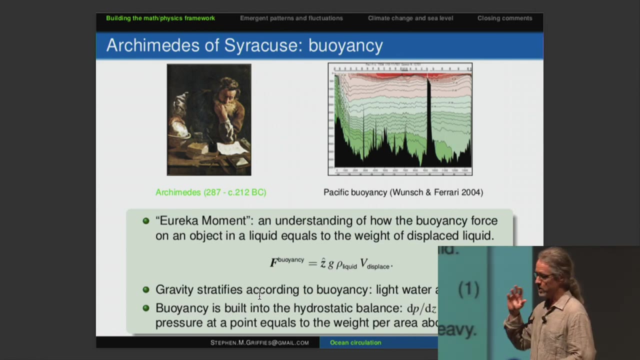 That go into building these models. And I'm going to step way back, Starting here with Archimedes. So the ocean and the atmosphere Are rotating fluids on a gravitating sphere, So gravity sorts the water In so far as you have dense water. 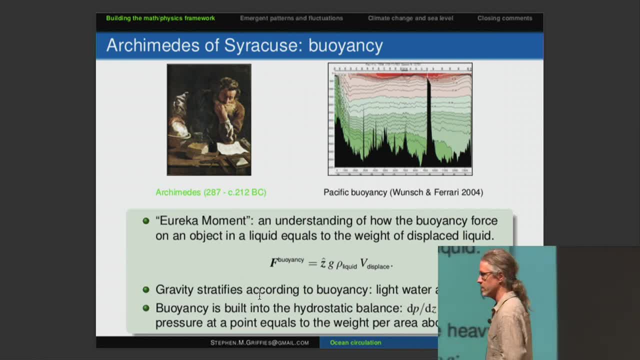 Heavy water beneath light water, And that concept is so intuitive That we just forget that it started really By this guy sitting in a bathtub Figuring out how do you weigh this crown And determine whether it was gold or not. So you have this idea of buoyancy. 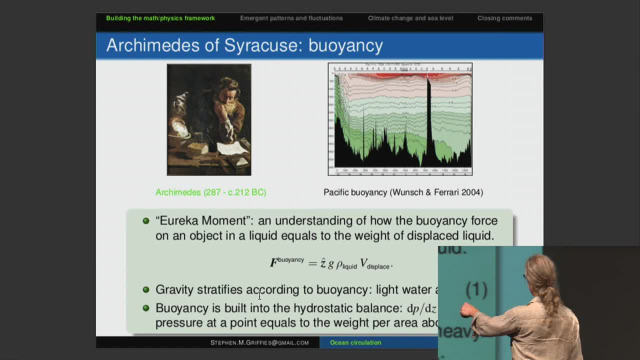 And this is an image here of the ocean, Sorted according to density, And it's a slice through the Pacific Ocean With depth going up. This is the surface of the ocean And this is the bottom. The black is the topography. 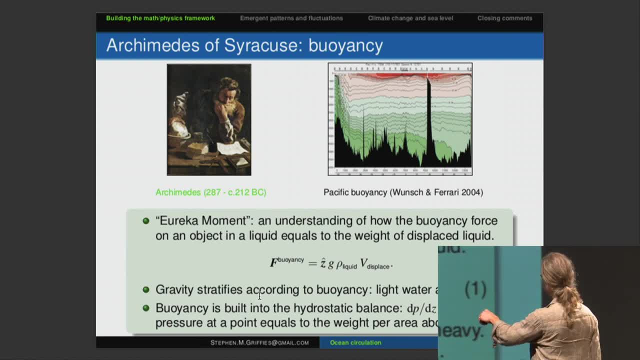 The earth going up and down In the bottom of the ocean, Very interesting geography there And creating these seamounts And these features. And you see, in the south, here to the left, This green water is dense water That spills into the deep ocean. 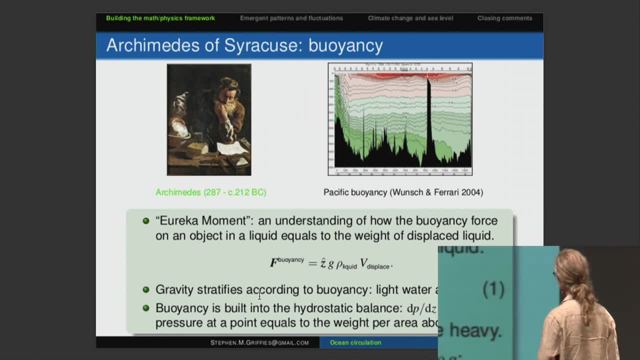 That's the densest water on the planet, Created off the coast of Antarctica, And you have warmer and lighter water that sits above it And as you go up into a region called the thermocline, You get very warm water, But this is a very basic property of the ocean. 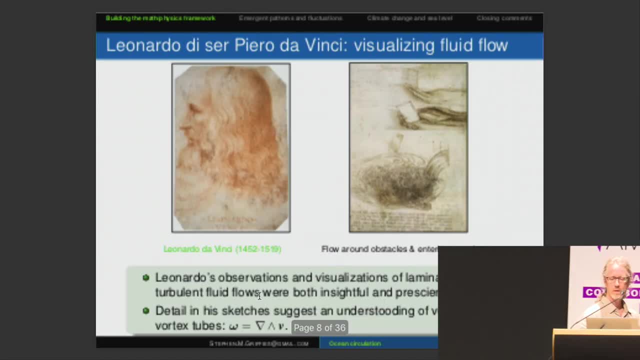 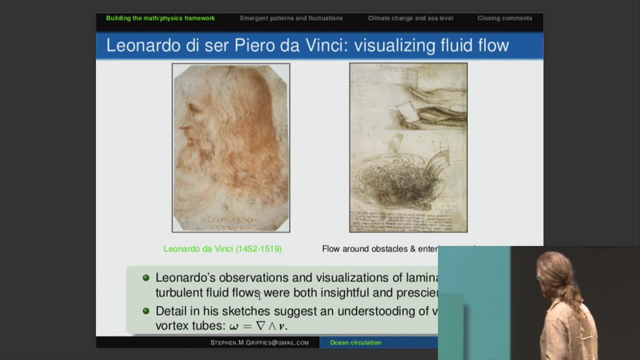 It's stratified. Another basic concept that I think is building up in time here. historically, This is Leonardo, And if you look at some of the images that Leonardo created, Just by observation, He didn't have computers, He didn't even have mathematics that Newton and Leibniz and Laplace figured out later. 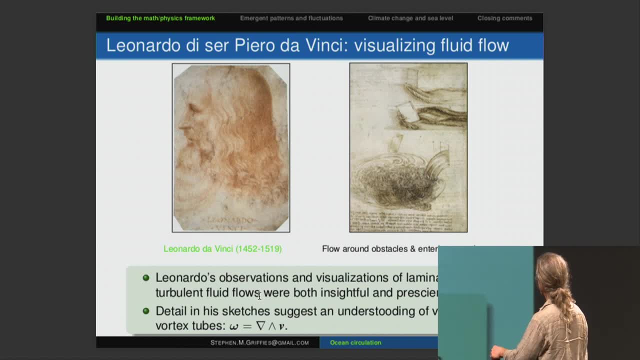 He was. He intuited, And just through observations, The whole idea of vorticity and vortex tubes. You can see that in his images He was drawing vortex tubes And looking at flow, going around obstacles And water moving into a pool here. 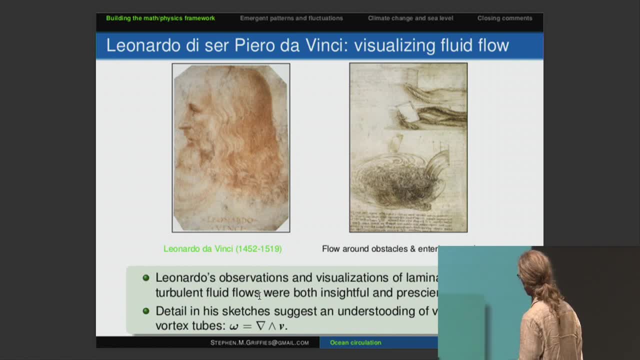 And you see these eddy features that he drew here. It's a fascinating, amazing fact that Leonardo was just able to see all of that Just by looking at it. And so visualization in general. The point of this image here is that visualization is a powerful tool. 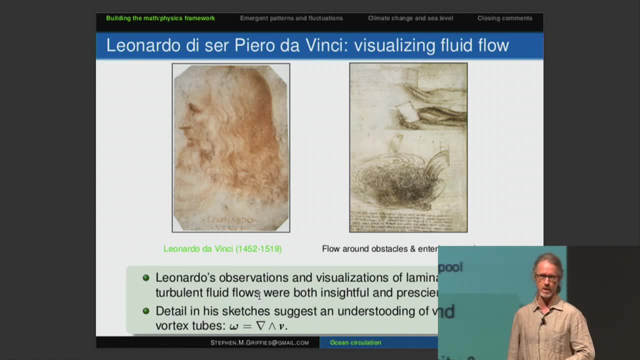 And it's becoming more and more sophisticated with the computer simulations that we're generating. Now That computer animations, Computer simulation, Visualization tools, There's some people talking about three dimensional holographic kind of ideas. Can you imagine walking through a holographic? 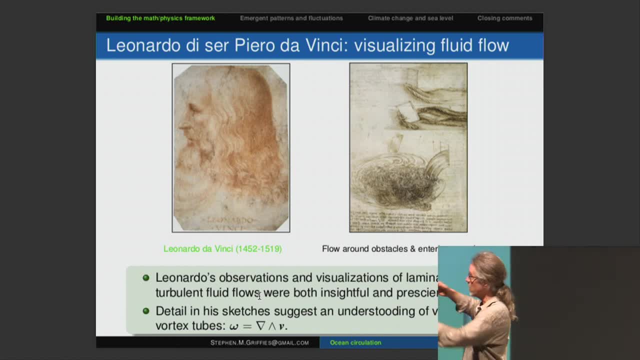 You know, Sort of like the holographic place in Star Trek, Where you're in the middle of the ocean with circulation patterns flowing around you. The ability to absorb the mathematics and the two dimensional structures Just opens you up to a whole new area of being able to see the understanding. 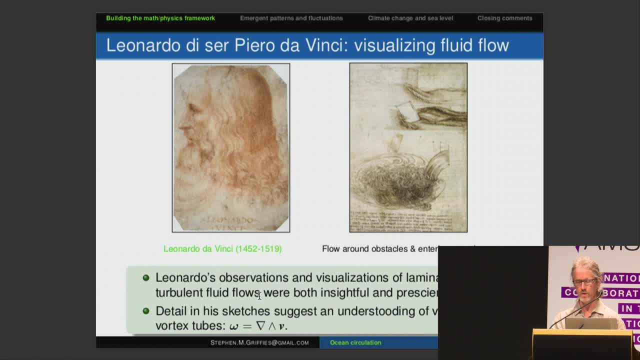 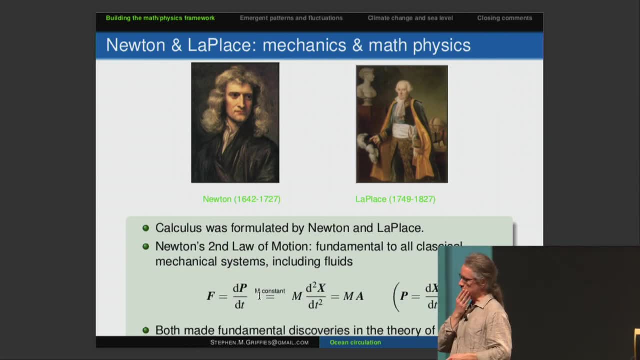 Understand what you're getting mathematically, And I can imagine in 10 or 20 years people are going to be looking back at us today And thinking we're in the stone age. So Newton and Laplace did a lot, of course. 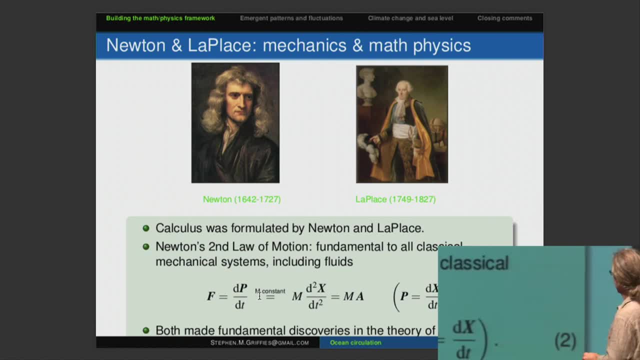 To develop mathematical physics and mechanics. And F equals MA is just so. Oh shoot, It's off the bottom here. It's so intuited that you forget that three or four hundred years ago, The fact that you had Newton's first law, 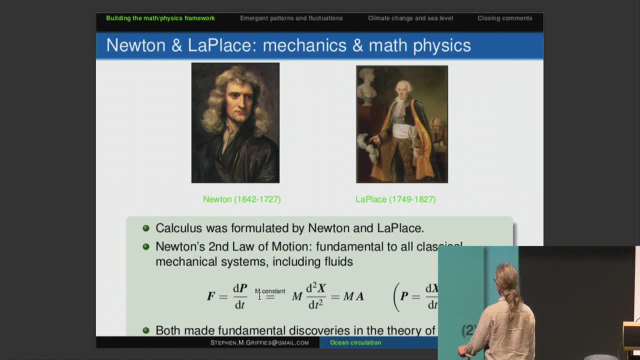 Or second law of motion, Was revolutionary. I mean, he was able to describe with this equation The motion of the planets As well as He didn't realize it himself, But as well as the motion of fluids, And Laplace did a lot as well. 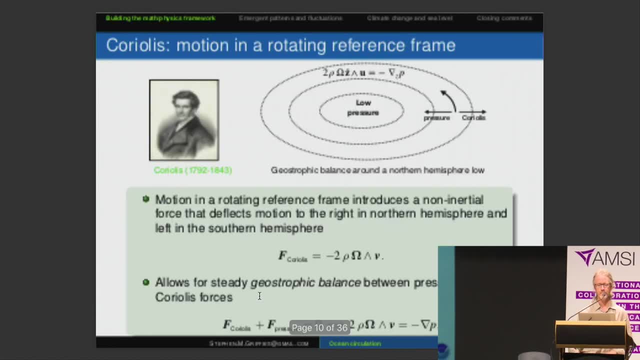 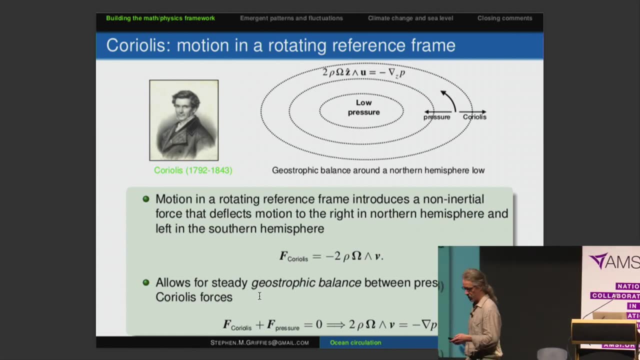 They both made fundamental discoveries in tides, by the way. So now the other point. We have a rotating planet. We may not realize it, But we're actually in a rapidly rotating planet Relative to other planets, And that rapid rotation is a very important feature. 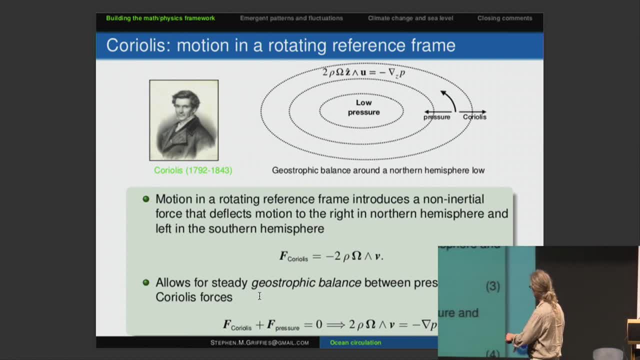 Of the fluid dynamics of the circulation. So Coriolis is the guy who studied. He was an engineer studying rotating engines And the fluid mechanics And just rotating physics in general And his Coriolis force Is a very first leading order term. 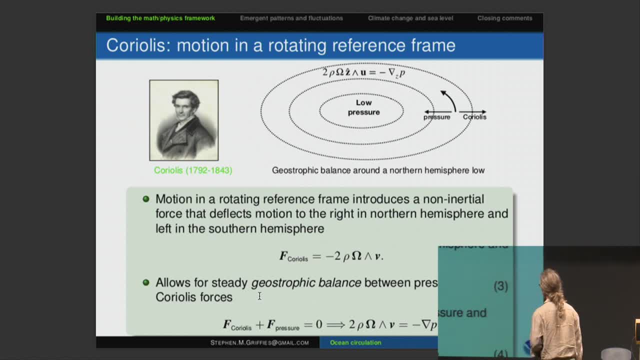 In the large scale circulation of the atmosphere in the ocean And you have what's called the geostrophic balance. And so geostrophic balance is a balance between pressure And Coriolis, And if you have a low pressure system in the northern hemisphere, 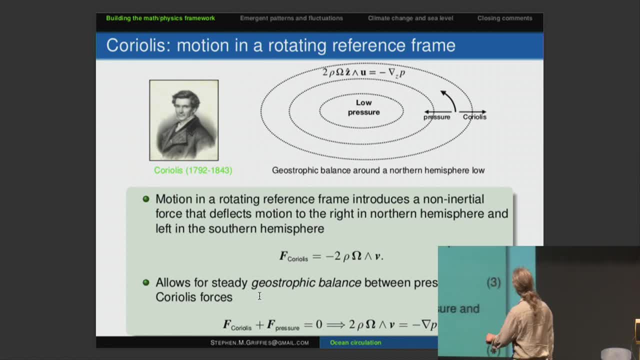 Apologies for being a northern hemisphere centric. The geostrophic balance is a balance between pressure Pulling you in toward the low pressure And the Coriolis pulling you outside, And it leads you to a circulation that goes around pressure contours. 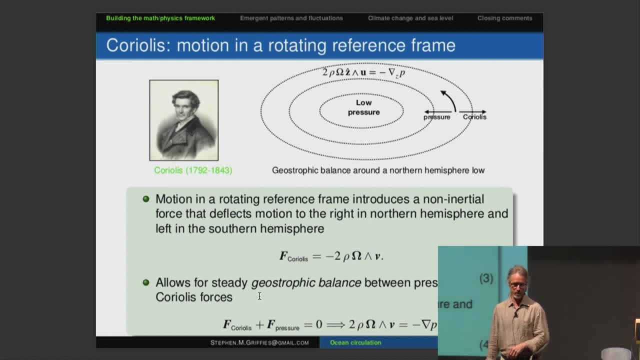 Parallel to pressure contours, Not perpendicular to it, Like you would have without rotation. So geostrophic balance. For the most part, Leading order circulation In oceans and atmosphere Is geostrophically balanced. So yeah, By the way, 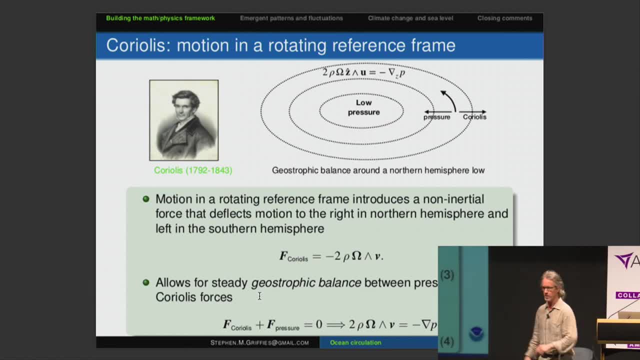 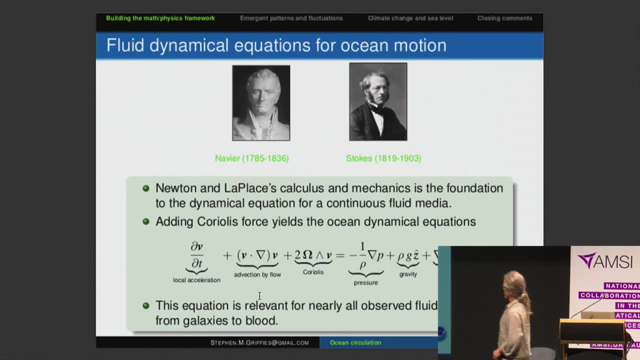 Is everything all right. Logistically, You guys are okay seeing. If there's any issues, Raise your hand. I can't see you, So you're probably not going to get anything changed. But So the fluid mechanical equations, That really 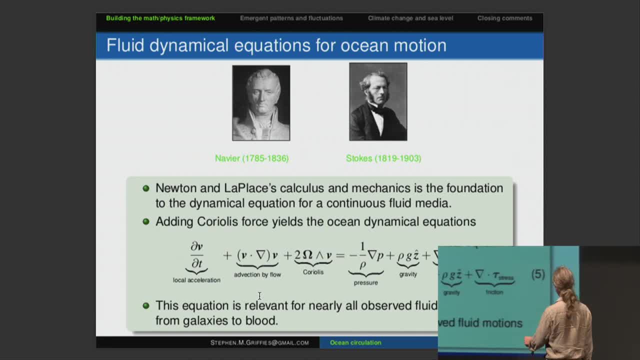 It's amazing. Okay, Newton Stokes. So the two guys- And we're not The equations of fluid mechanics That we all Start from, Basically Called the Navier-Stokes equations, And so here they are. Here's a bit of math. 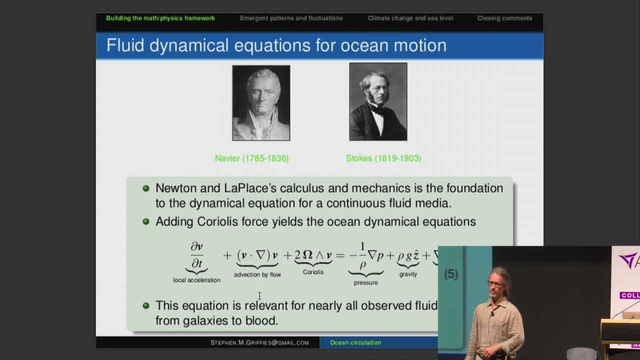 Again You have velocity field V. The local time derivative of that Is a local acceleration Plus an advection. So advection is a Fact, that fluid is moving And that can change the properties Through a process known as advection. 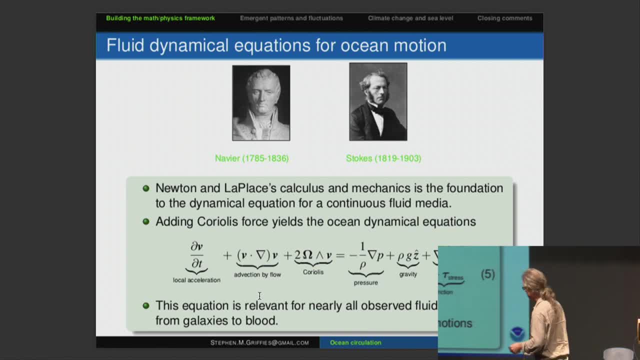 Or some In the engineering community That's called convection. But convection Has a particular meaning In the atmosphere And ocean science, And so You know, You know, In the atmosphere And ocean science Is that. 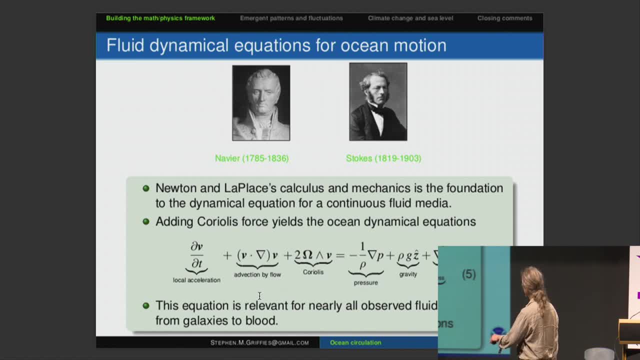 Is distinct. The Coriolis Acceleration Is here, It's. It's a cross product Here Of the Rotation Of the planet Times, the Cross product Into the velocity field. Here's your pressure force. 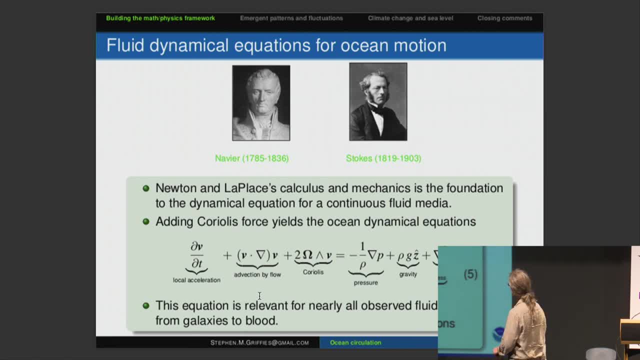 Pressure, gradient force. Here is a gravitational term. Gravity moves vertically, Z hat Is in the vertical In our notation, And there's a frictional term, The fact that you have Fluid parcels Rubbing against each other, Exchanging. 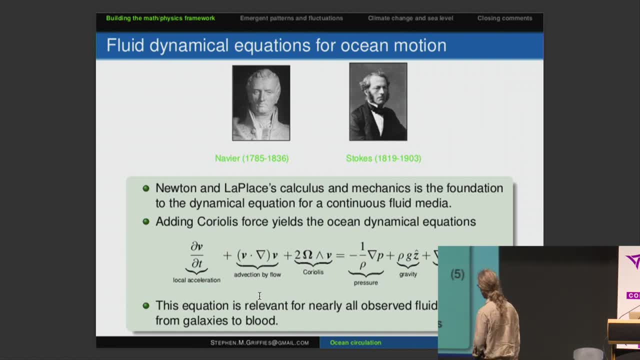 Momentum Between each other Creates Stress And friction. Also, When you interact With the atmosphere Or the topography, The bottom Of the earth Below, There's a frictional Interaction Between that. It's amazing. 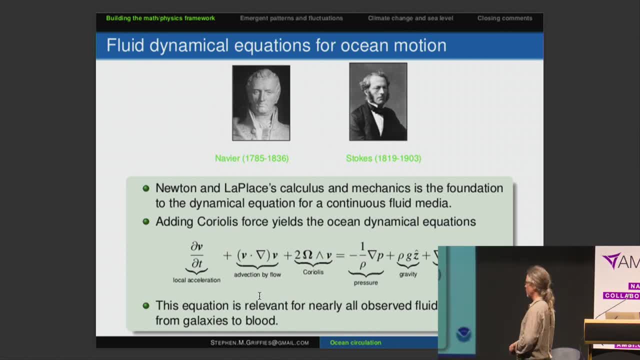 That this Equation Is relevant For Is, For the most part, Most observed Fluid mechanical motion, All the way From galaxies To blood flow. It's an amazingly Rich System Here That You To make use of. 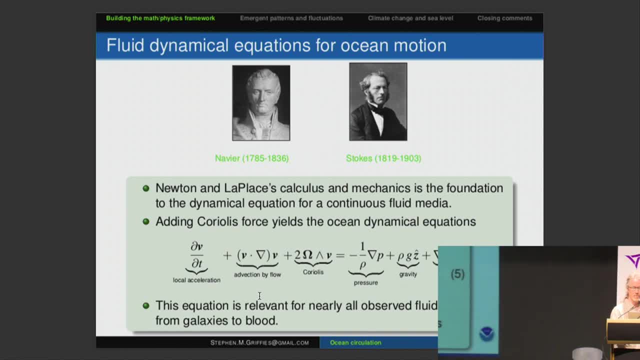 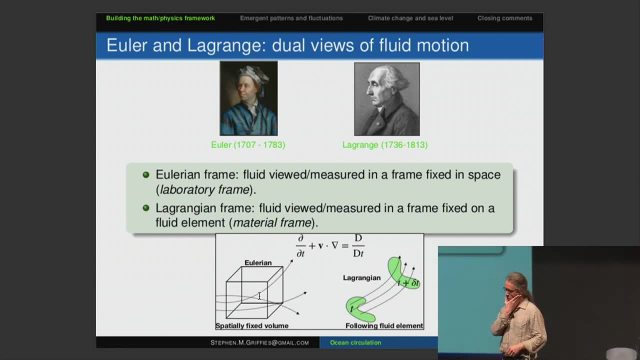 But nonetheless It is the grand Unified Equations For Fluid mechanics, Environmental fluid mechanics And fluid mechanics In general. So Another piece That I'd like to To Raise To you. It's Probably 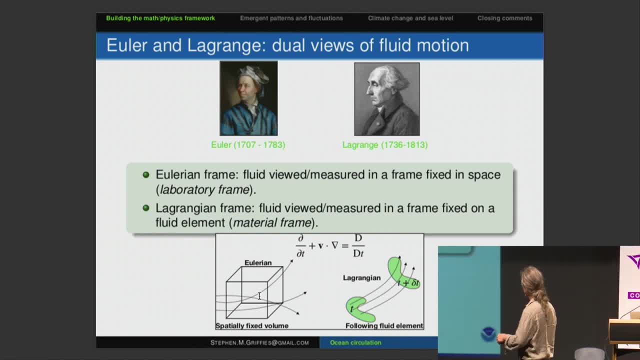 Something That's Going To be A little Subtle For Some Of The World. So The Idea Of What You Think About, What You Observe When, 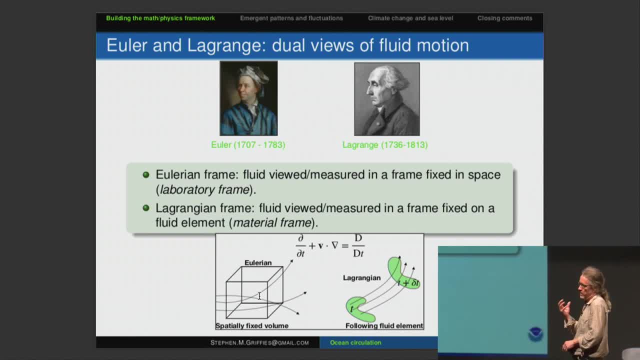 You're Looking At Fluid Motion Here. How Do You Describe That? I Mean These Guys Were, And So You Can Take Many Different Perspectives In. 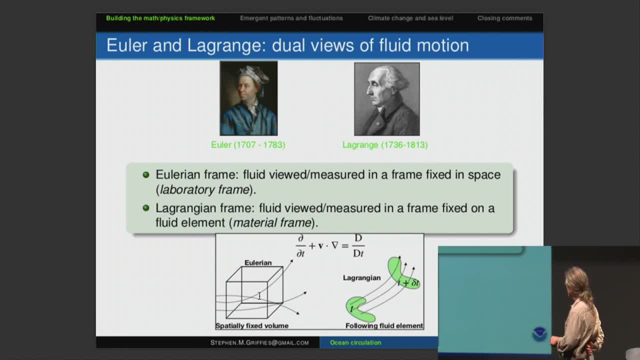 Orler And Lagrange. Really My Understanding Historically Is Orler Did Both Of These. Lagrange's Name Is Attached To Lagrange's Lagrangian Is. 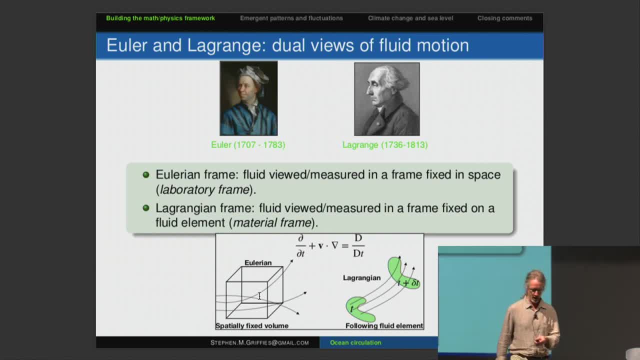 A Particle Of Fluid You're Moving With It. It's A Moving Reference Frame, And So The Kinematic Description Requires A Transformation Between The Two. 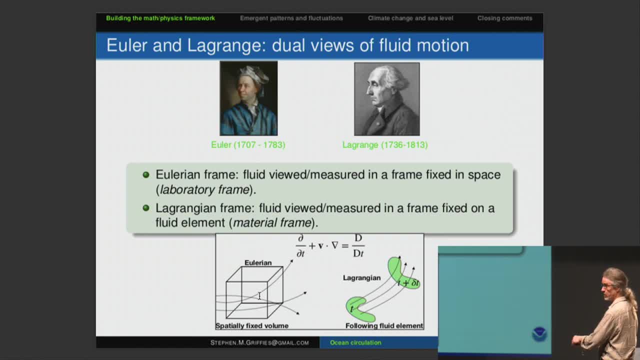 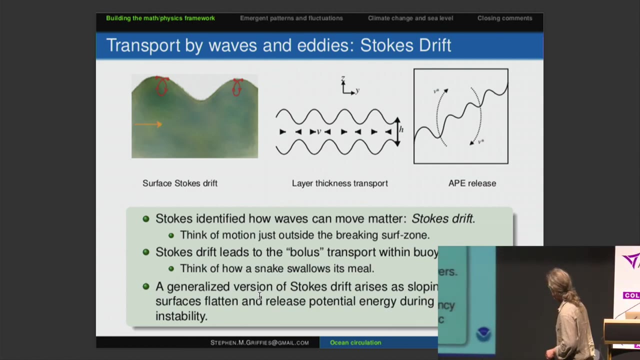 The Left Hand Side. Okay, Lagrangian Frame, Your Fall, You Move In With The Fluid Patch. So This Is Even More Subtle, I'm Expecting. 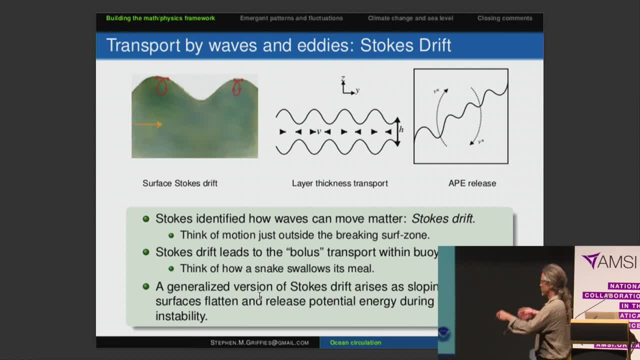 That That Many Of You Will Will Find This- That The Motion Of The Wave At Your, Your Head, Is Bigger Than The Motion Down. 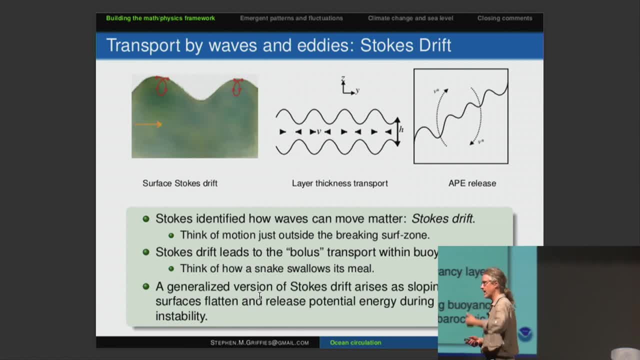 Below. Okay, So As The Wave Is Moving By, It's Moving And The And You Get A Net Mass Transport And That's A Net Matter. 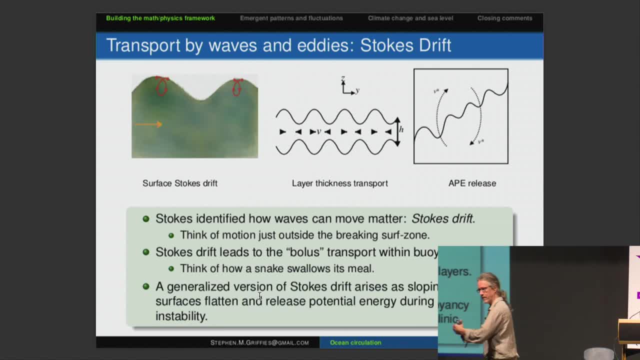 Transport Due To Stokes Flow In The Ocean. Where You Have These Density Layers? You Have These, So You Have A Density Surface That Is Upward. 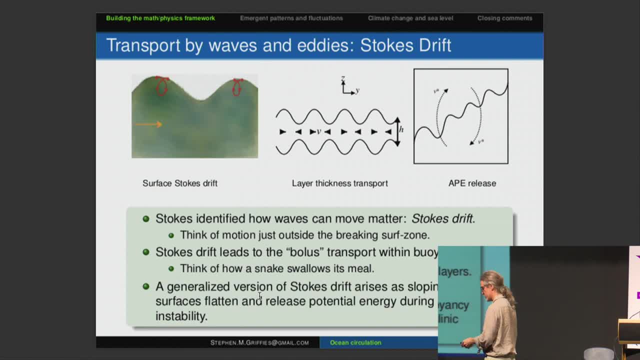 Like This And It Has Some Energy That Needs To Do To Rise That That, To Get That Density Service. I Hope That Some Of You 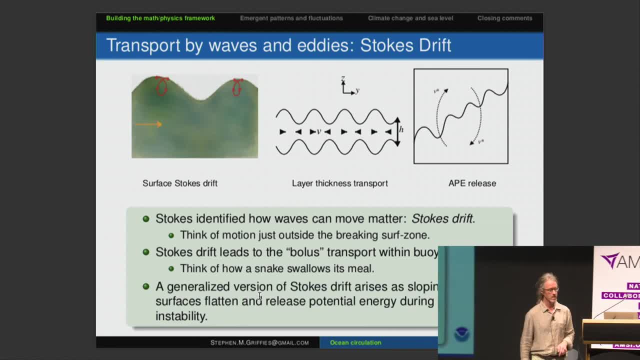 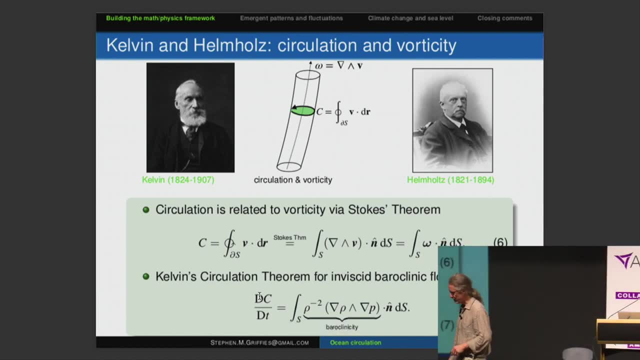 Will Appreciate. It Is If You, If You Do Any Fluid Mechanics, You Will Probably, And You Do Wave Mechanics, You Will See If You. 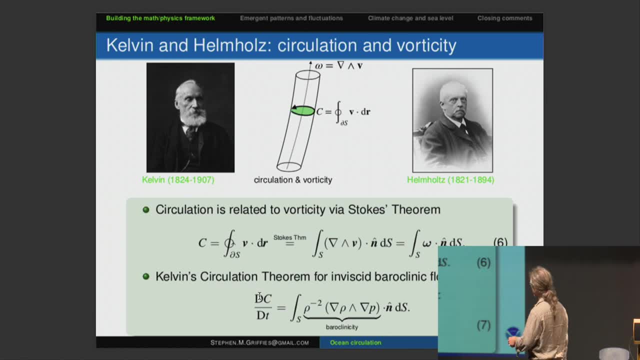 Think About Fluid Mechanics. They Thought A Lot But They Argued A Lot, And The Arguments Back Then Were An Englishman Or Not An Englishman. 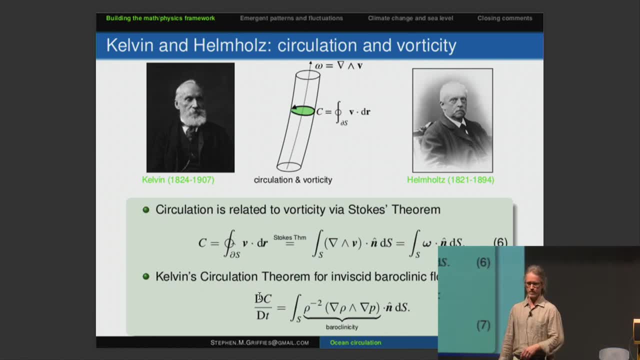 He Was Felt The Book Of The 断 dizer And Result Of The Enquiry From The History To The History Of Things And Of 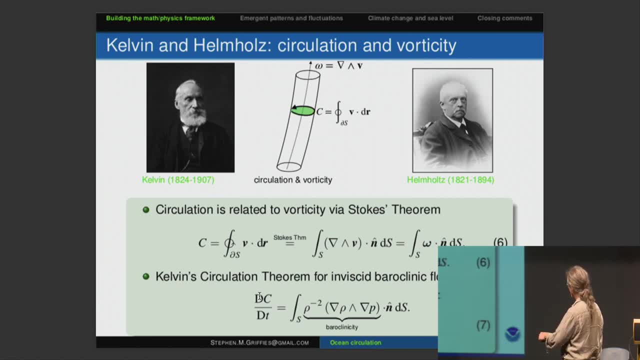 The History Of The History. Exactly, The Kelvin's circulation theorem is a very important theorem that tells you how, and using the equations of motion, how the circulation changes following a fluid parcel. okay, And it changes because of what's called baroclinicity. It's where you have density, surfaces and pressure. 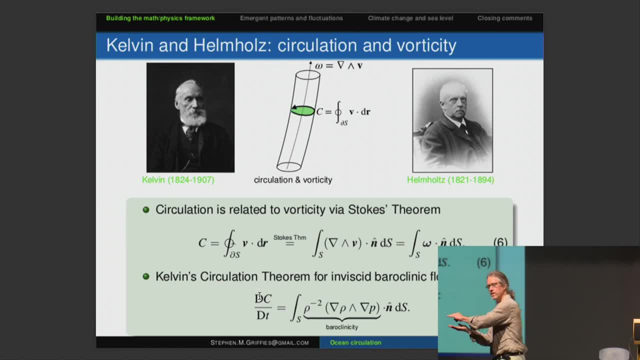 surfaces that are misaligned and you have a net torque applied to that circulation that spins up these features, And so it's sort of take an everyday experience of just whirlwinds. This is a vortex tube and you have these whirlwinds of motion that have a circulation. 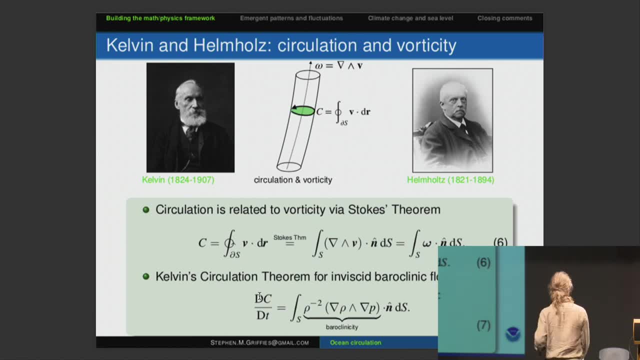 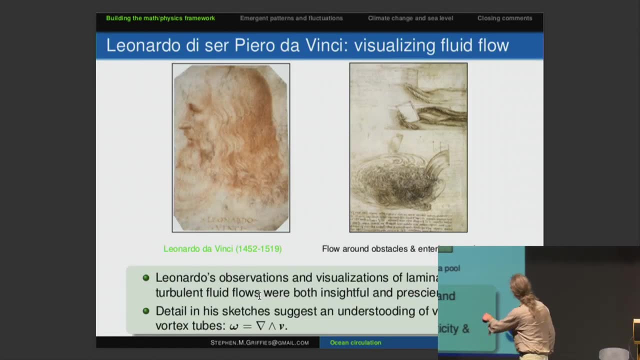 and the vorticity that creates these vortex tubes. going back to- if you can see the image from old Leonardo here, this is a vortex tube from that following from that obstacle there, and these features here are vortex tubes And there's lots of small vortex tubes in. 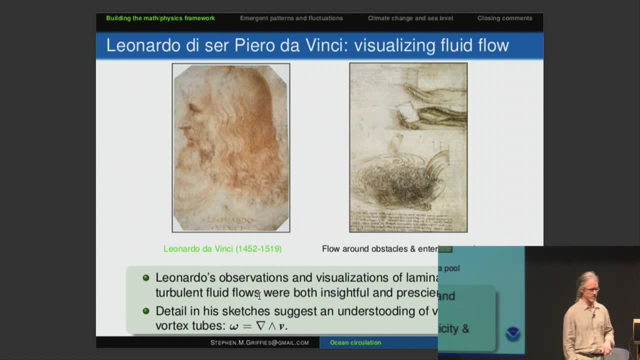 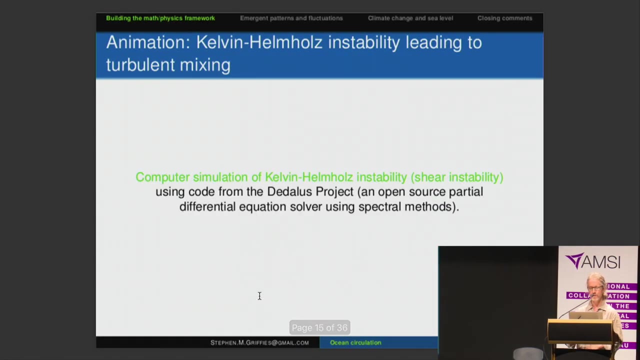 this pool of water that he's drawn here And it's, it's, it's. you can see vortex tubes and everyday experience. I've- I've seen water spouts and and just water going down a tube or a bathtub. You get vorticity going through that, So let's take a break here. There's. 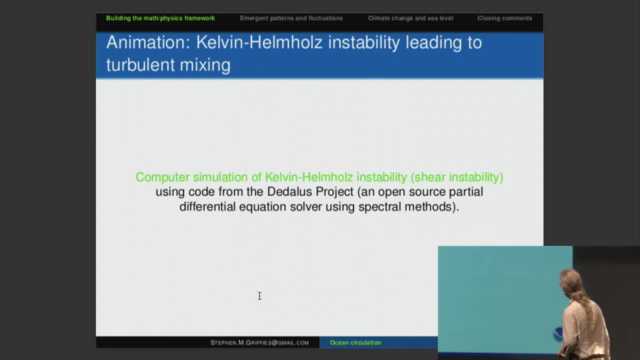 something called the Kelvin-Helmholtz instability process, And I showed you this image, this big circulation movie, to start off with. I'm gonna do. I'm gonna jump to the opposite here And look at a process that is in, animated by a piece of software that I was turned on. 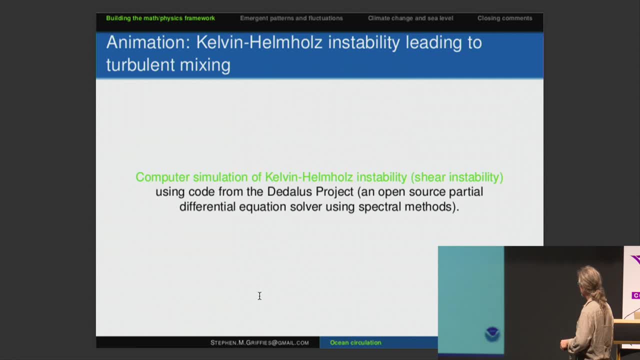 by a postdoc in Sydney a few years ago, when I when he showed me this Daedalus, I said: you lazy guy, why don't you go write your own code, you know? And he says: but this is such an amazing tool And I, I'm, I'm a convert, I have a graduate student, that's. 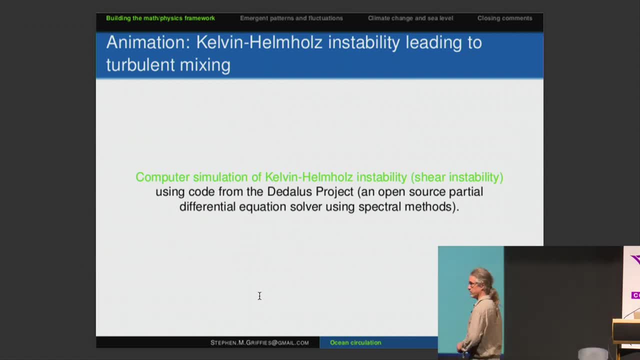 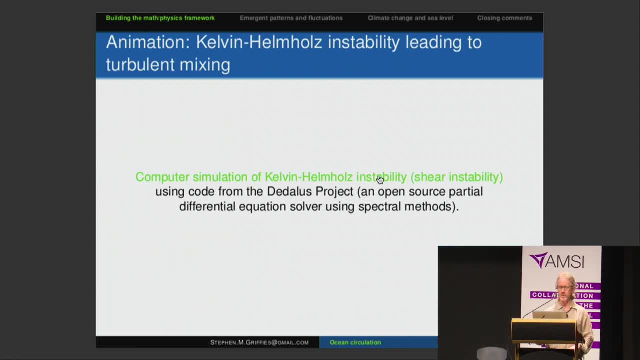 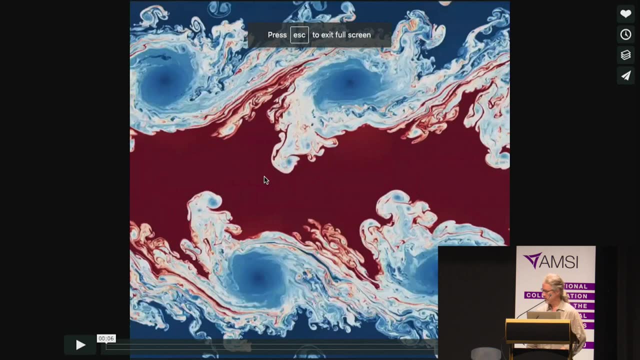 and feet. this, this one. I won't tell you what it is. So the computer simulation is of of just a mixing event A, a hydrodynamic instability known as Kelvin-Helm Oates, And you can. this happens everywhere in the ocean. This kind of instability creates mixing. 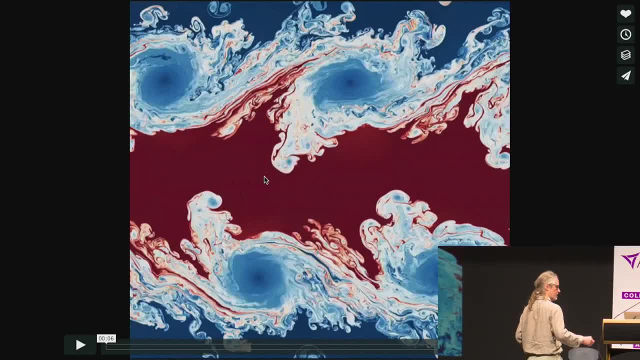 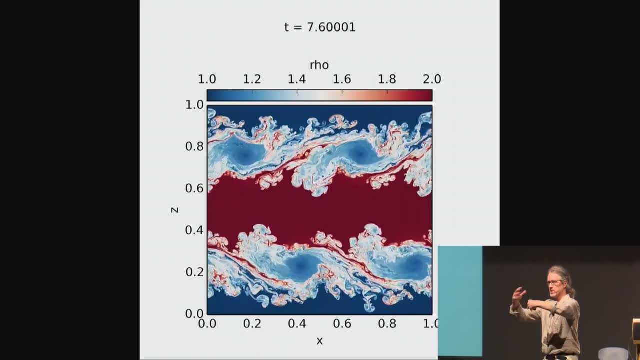 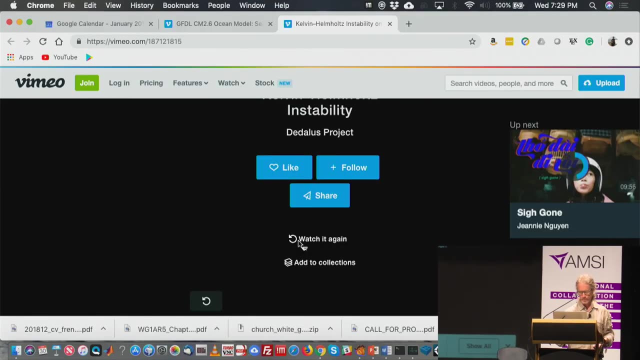 It. it mixes heat and and salt and water, And so you just, you just start a simulation where you have this shear, this motion of fluid moving in different directions, and you create these, these. it's such a short animation. see if I can redo it. Watch again. I'm not going to go to full screen, Let's just watch it from. 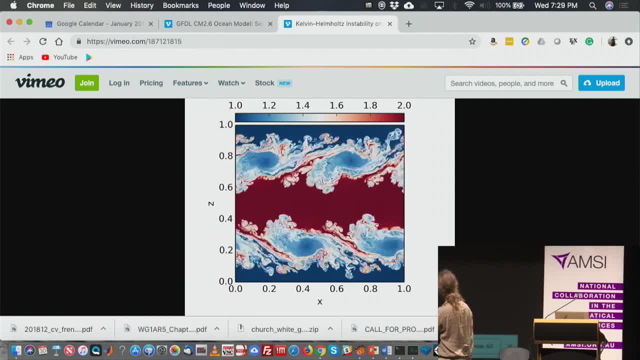 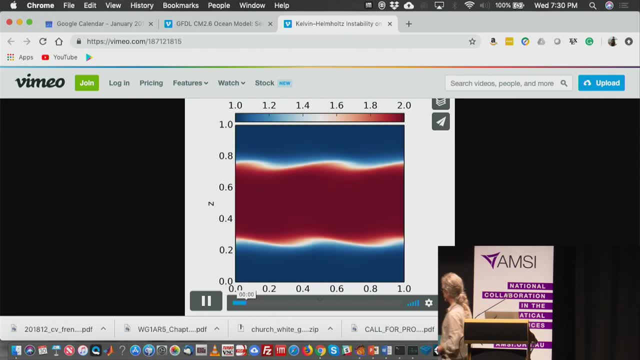 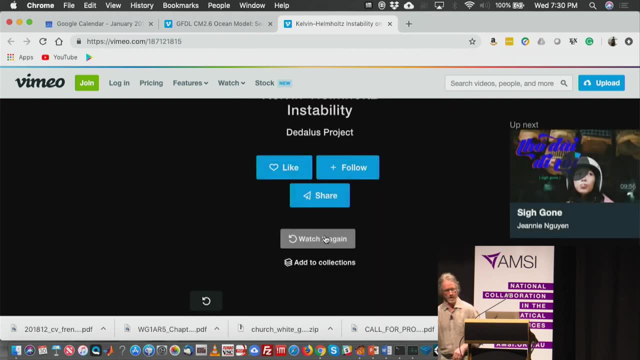 this And you create these cat's eyes that are really beautiful, And then you get this homogenization near the edges And if they ran it longer, you would see homogenization throughout most of the interior of the layer. here It's a brilliant piece of animation And it's indicative of the 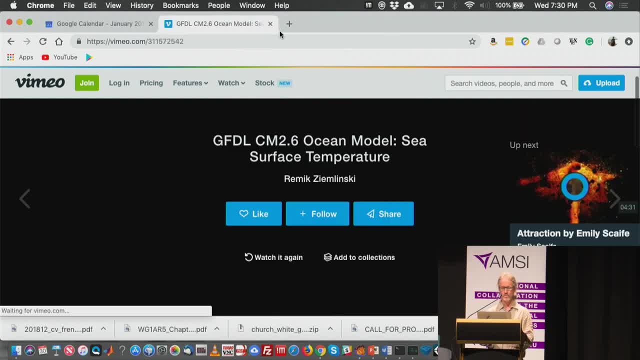 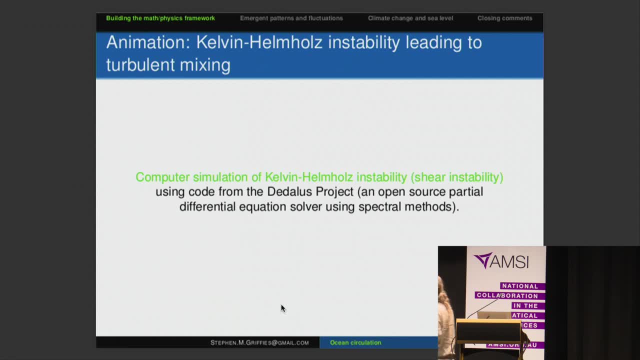 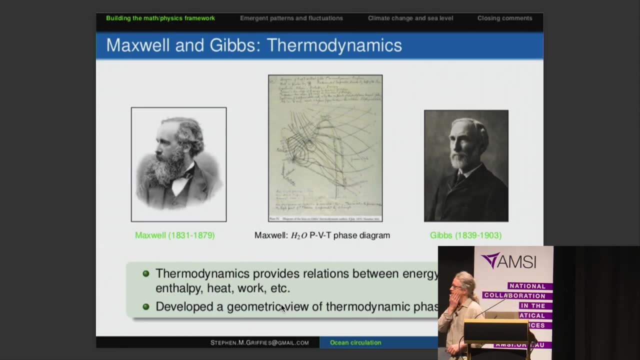 fact that fluids are intrinsically unstable through many different mechanisms, And that particular mechanism is one that Calvin and Helmholtz worked on a couple hundred years ago, almost 150 years ago, Gibbs and Maxwell. You can't go far in physics without talking about 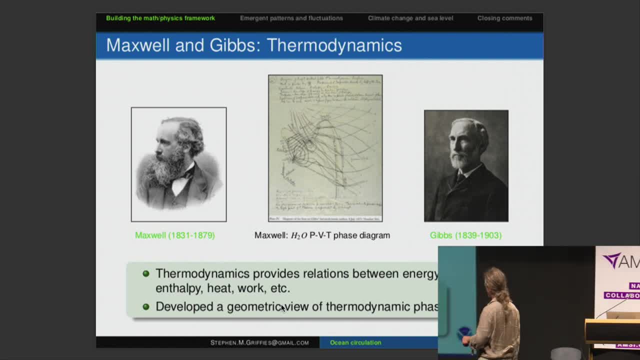 these two guys And their contributions were massive in all different areas and in particular in statistical mechanics And in thermodynamics. This is really one of the last pieces to this process of building up the equations of ocean fluid mechanics is to remember that we have heat in the ocean And heat and the 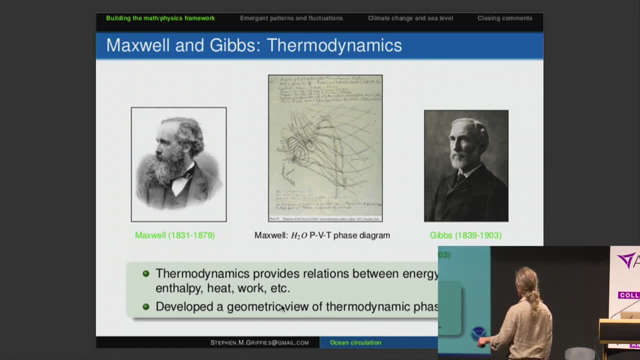 movement of heat and energy involves thermodynamics, And the thing that was also impressive about some of their work is that they develop a geometrical view of thermodynamics. This is a sketch here that Maxwell wrote on a piece of paper and sent it to Gibbs. 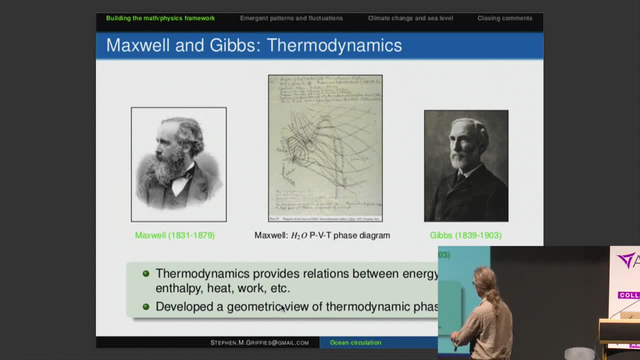 This is a sketch of the phase diagram, The pressure volume, temperature phase diagram for water- pure water- And Maxwell was so impressed by a piece of work that Gibbs published that. Maxwell created a 3D model out of clay or whatever and sent it to Gibbs as a present. Gibbs was at Yale and Maxwell was at 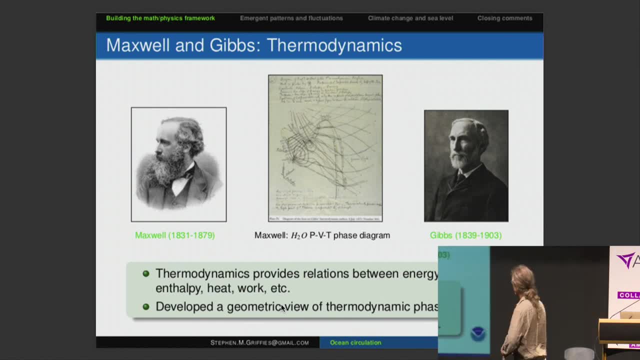 at Cambridge And you can imagine. he put it on a ship and it probably took a couple of months to get over And Gibbs was like, wow, what an amazing present. And that's still at some museum, I don't know It's체. 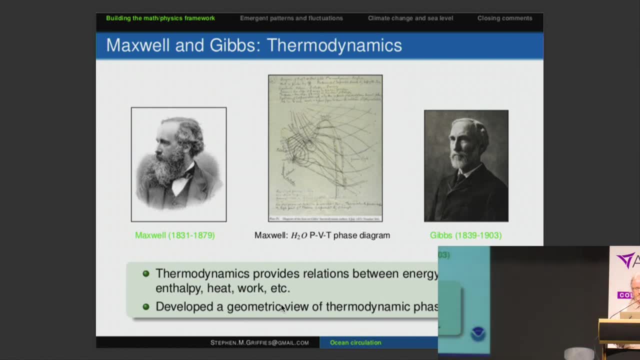 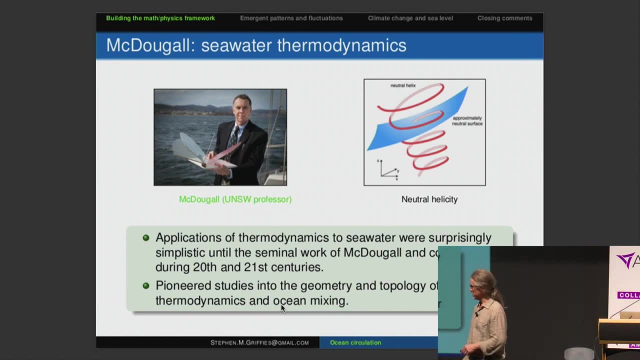 maybe at Yale, I'm not sure. so I'm gonna jump ahead to a modern thermodynamic person that is in many people's. he's a mentor of a number of people in this room and his professor at UNSW is Trevor McDougal. he has done a lot to modernize. 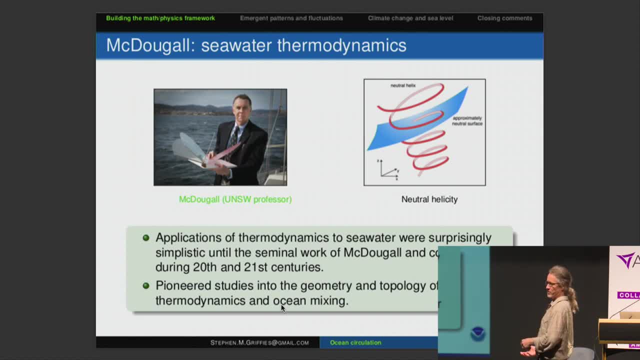 the treatment of thermodynamics in the ocean and really to bring it back to the fundamentals and in thinking about the geometry of ocean circulation and ocean mixing and just ocean thermodynamics, and this is a picture of a very interesting process in the ocean called neutral helicity, where you have these. 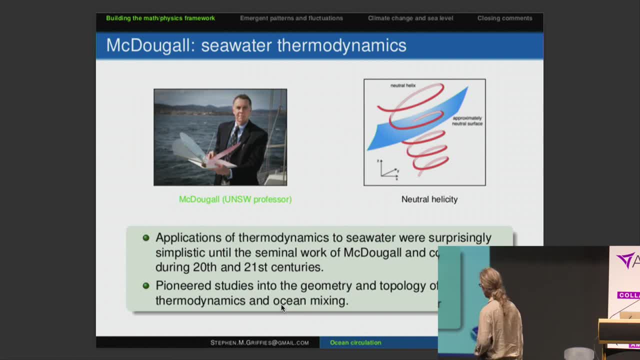 topologically, non-trivial, helical structures of trajectories if you follow a particular recipe to get through, to get the mixing to happen in that way. and so yeah, McDougal is is an icon in the field and he's sitting right in this in this room and he's sitting right in this in this room and he's sitting right in this. 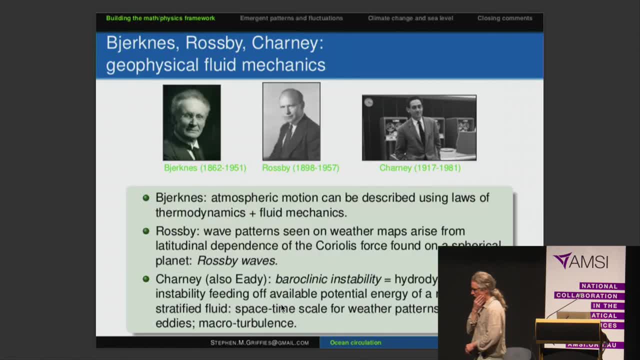 in this uh University. so now we've got some of the main pieces here. we've got the Navier-Stokes equation, we've got thermodynamics, we've got lots of different stuff, and so let's uh, what is geophysical fluid mechanics? well, there's a number of icons of the 20th century. these are three that I chose in particular. 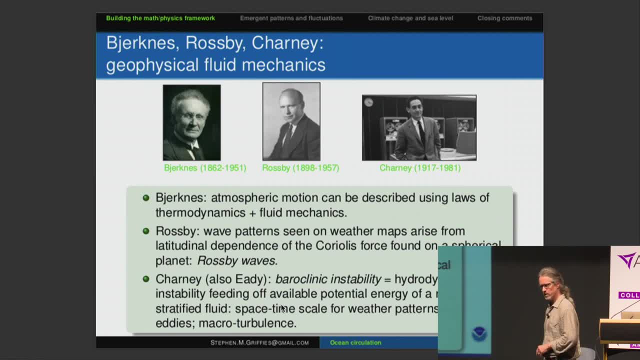 Bjorknes, Rossby and Charney Bjorknes in the in the turn of the 20th century said: hey, we could use physics, we could use math to describe what we're looking at in the atmosphere, because before that they were just making maps, they were doing sort of predictions based on what they saw. 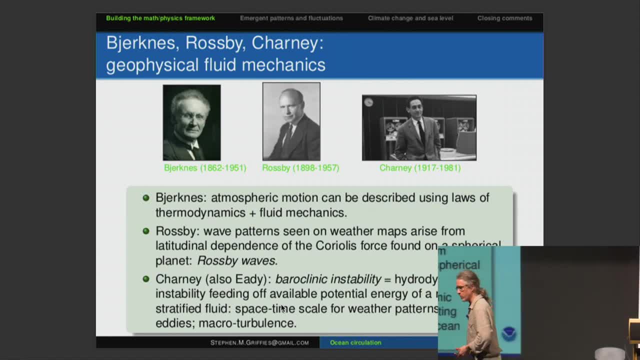 the previous week or whatever. they weren't using the laws of physics, they weren't using continual mechanics, they were just doing it empirically, based on just looking at maps. Bjerke's said and he did some work and he started the Bergen School of meteorology, which is continues to be quite an. 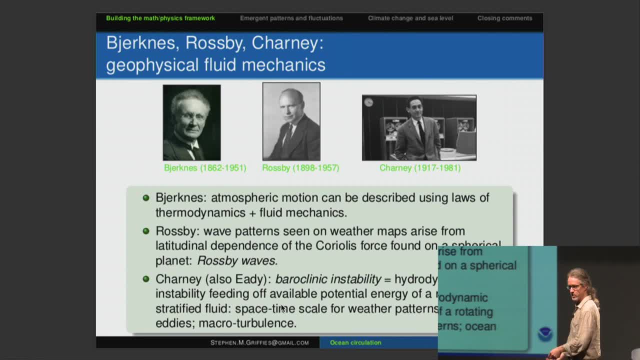 influential piece of work and he had a son who became a big professor at UCLA. blah, blah, it's, it's, it's itself. can imagine at the time. I don't know if it was an aha experience or if he had to push through and figure it out, but it's like wow, we could use this stuff that these guys in the physics 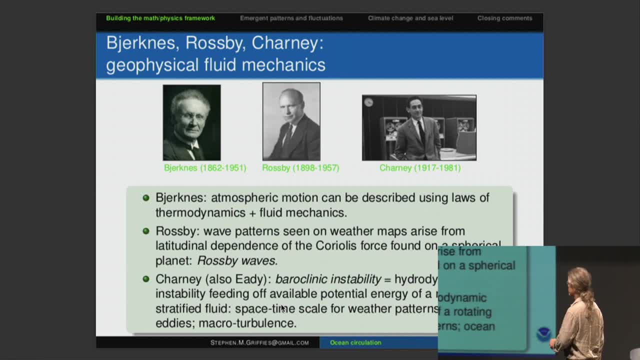 department are doing. Rossby came along and said: these big waves that you guys are looking at on the weather charts, these are planetary waves due to the fact that the Earth is rotating and it's a sphere, And these waves later became known as Rossby waves And we see those in the Earth. 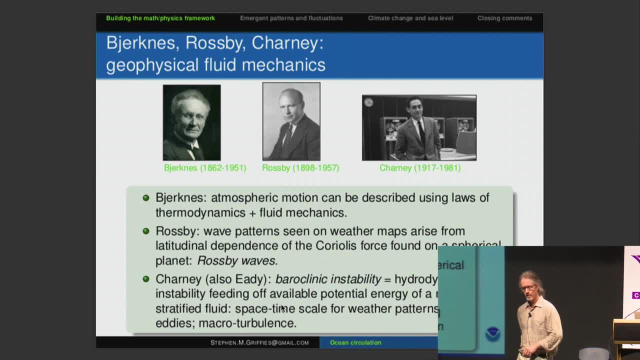 in the ocean and the atmosphere. Charney came along and described the instability associated with these eddies that we're looking at, known as baroclinic eddies or baroclinic instability. It's basically an instability that releases the potential energy. 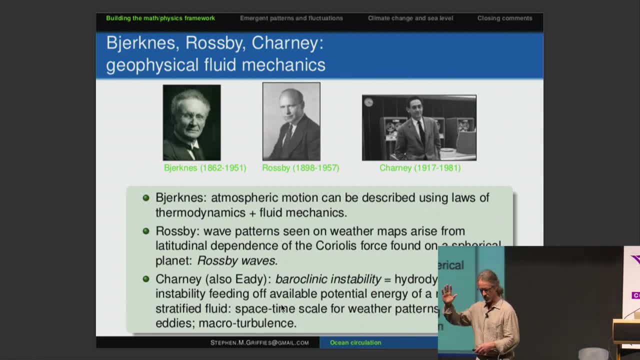 of these sloped density surfaces or these sloped buoyancy surfaces. I love this picture because it shows an old digital computer back then, back probably in the 60s, which was very similar to the one that was started at my lab, And Charney was one of the founders of the. 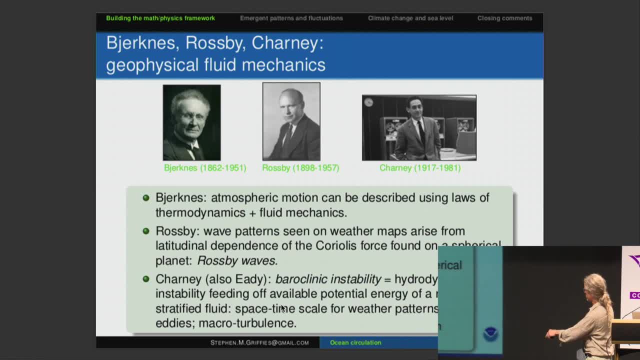 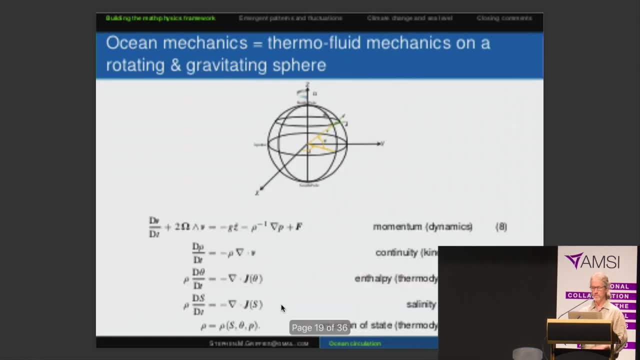 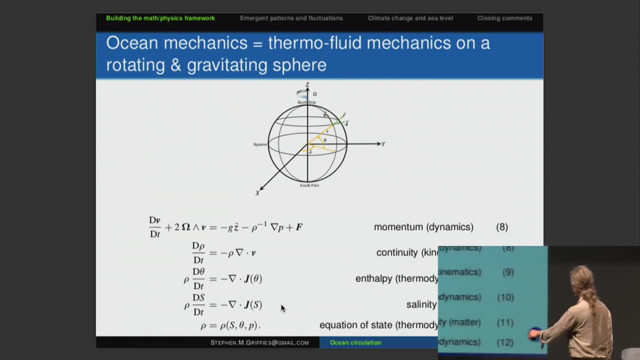 lab that I work in Princeton- Also, just to give some shout out to Eric Edie who was also came- was very influential in baroclinic instability. So here we are, the equations, the grand unified equations of ocean and atmospheric dynamics. We have the Navier-Stokes equations on a rotating 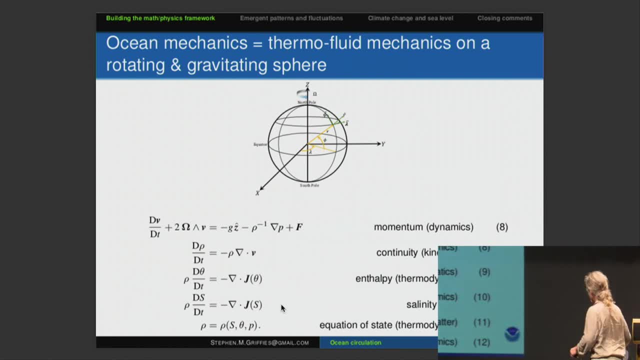 sphere, which is the momentum equation, which goes under the name dynamics. We have kinematics here, which says that you conserve mass of your fluid, and that goes under the name of the continuity equation. We have the heat equation, or enthalpy equation, which the theta is a potential enthalpy or some enthalpy, and the J. 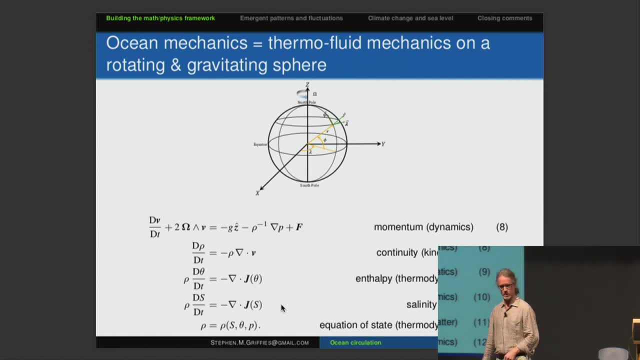 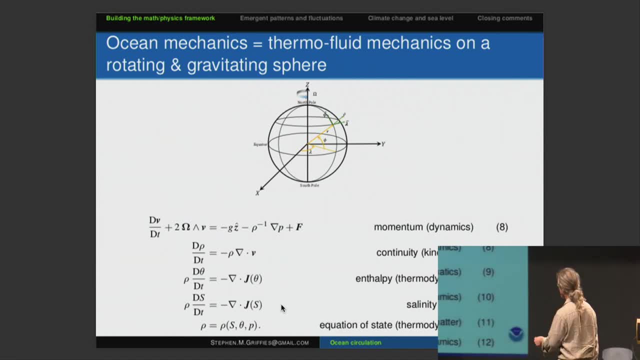 we don't have a lot of energy. we don't have a lot of energy. we don't have a lot of energy, We don't have electromagnetism. we don't have strong force, nuclear force, We have gravity, we have pressure. 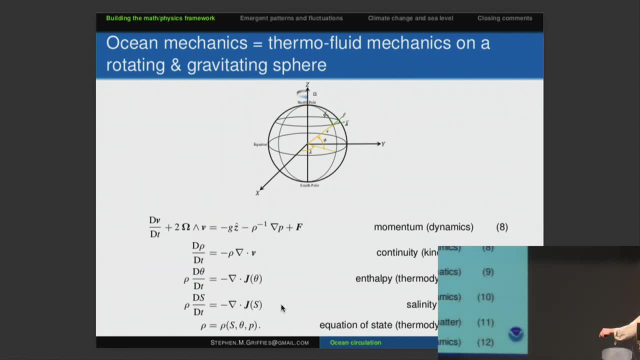 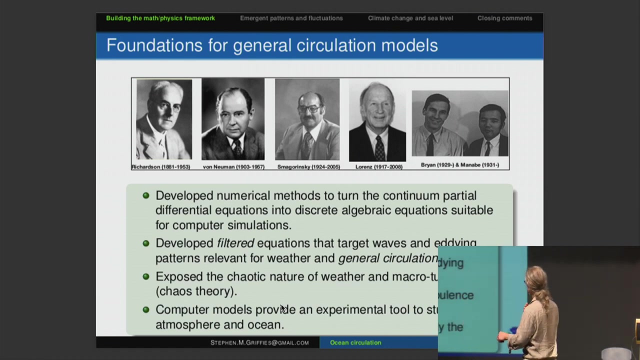 we have Coriolis and we have matter conservation in various forms and we have thermodynamics. Those are the equations that we use, those are the fundamental processes that we use to think about the ocean, And so here's a suite of people that really founded general circulation models. 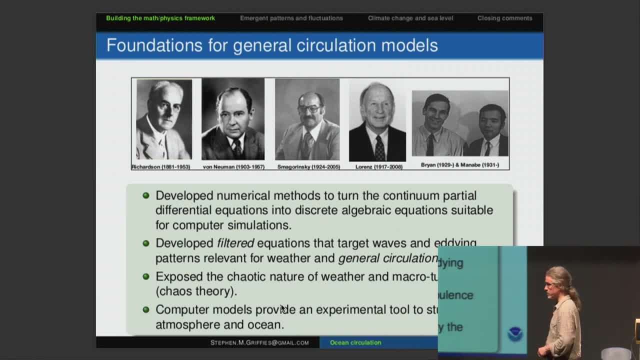 mostly atmospheric work, but they were translated over time into ocean: Richardson von Neumann, Smagorinsky, Lorentz and Brian and Manabe. So let me give you the brief on these guys. Richardson came along around World War I in the 20s and said: 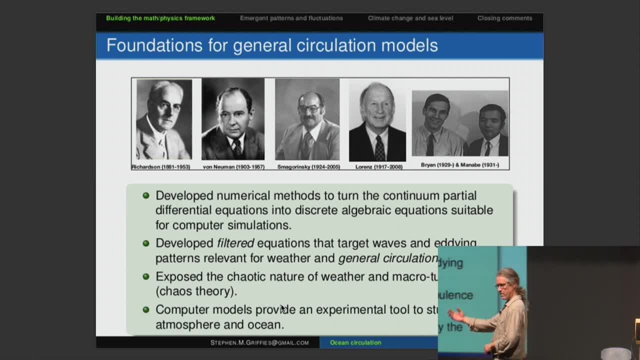 I think we can compute the state of the atmosphere. if we've got the equation, now Let's just compute. Well, what computers were in his time was a room full of people, mostly women, who could calculate really fast by hand. Well, the problem with what he was doing is he didn't. 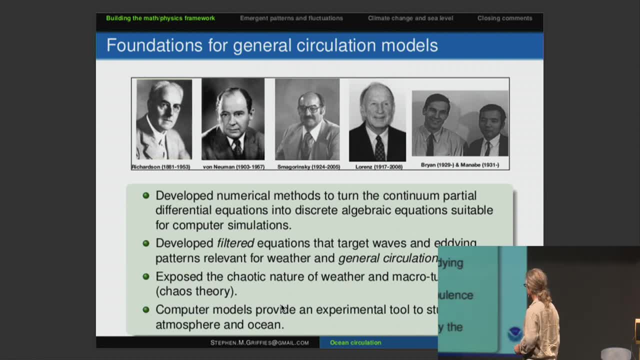 he applied the full Navier-Stokes equations that I was showing you on the previous slide, and it just proved to be too complicated. You had these fast modes that were unable to be represented. Von Neumann was at the Institute for Advanced Study in Princeton. 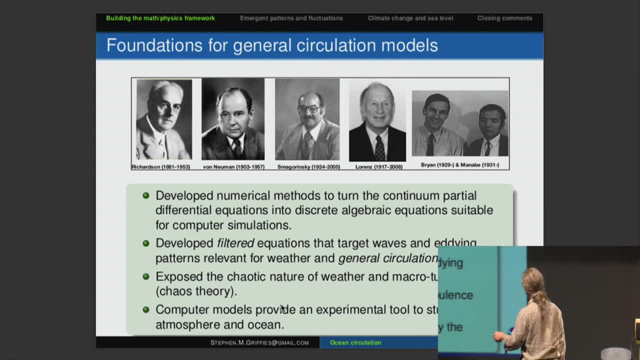 and grabbed a bunch of the best meteorologists- Smagorinsky, Charney, a few others- and said: let's build a general circulation project with this new computer we've got here. And these guys knew about simplified equations, approximate equations, 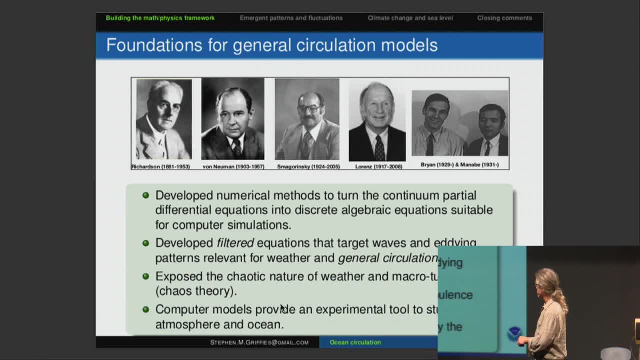 and they succeeded in building it. They were the first weather models. Smagorinsky started the lab I work at in Princeton Lorentz. of course, founder of chaos theory was a meteorologist, And this is my mentor, Kirk Bryan, and his partner in crime, Suki Manabe. 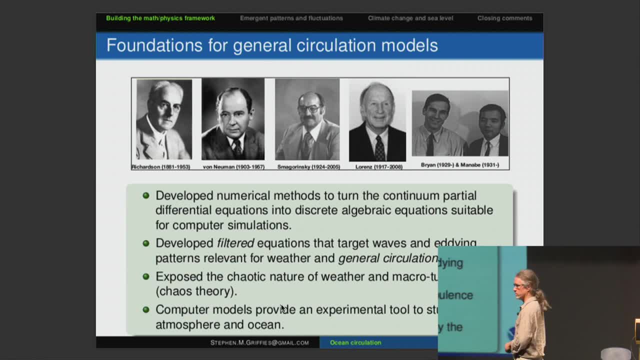 two of the most famous, the founder of ocean numerical modeling and father of global warming. effectively, They produced the first climate model in the 60s, which has won them all kind of accolades. So that's the first climate model. 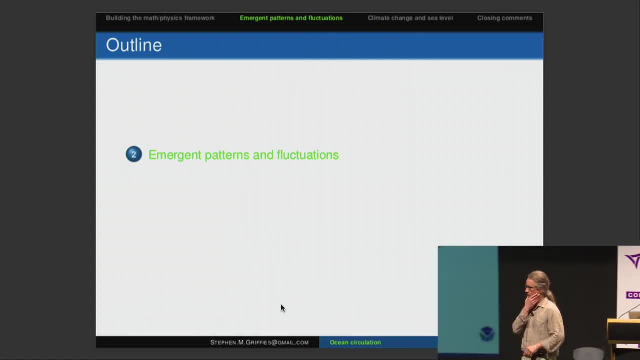 So that's the first climate model. So that's the first climate model. So we've got the equations. What emerges from those equations? So you might have heard this term before- emergent phenomena, If you write down the. I came out of string theory and so the goal. 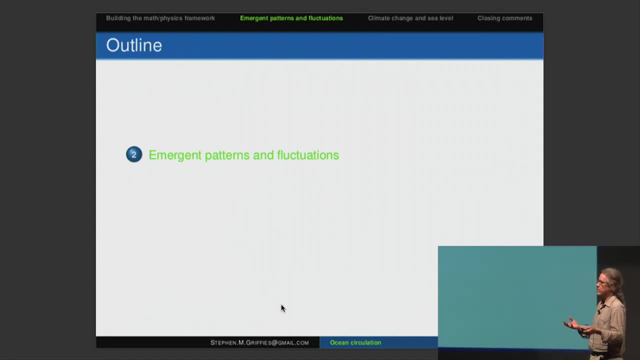 of string theory really was to understand the basic equations of the universe. We've got that. You know, when I came into the field I go: what's the big deal? You've got the equations, You know what's to do. 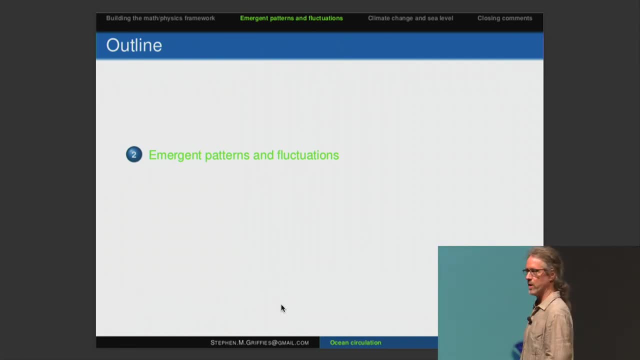 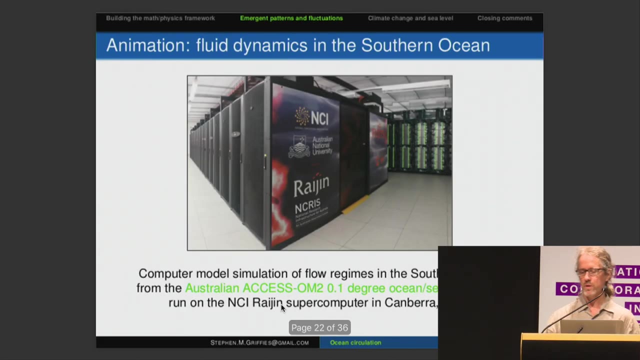 Well, there's a whole lot of stuff that matters, that comes out of those equations that emerges. It's hard to predict the ocean circulation Just looking at those equations that I showed you. So that's where computations come, of course, where analysis comes involved as well. 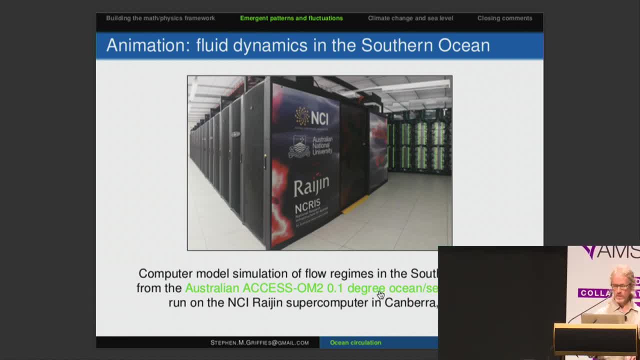 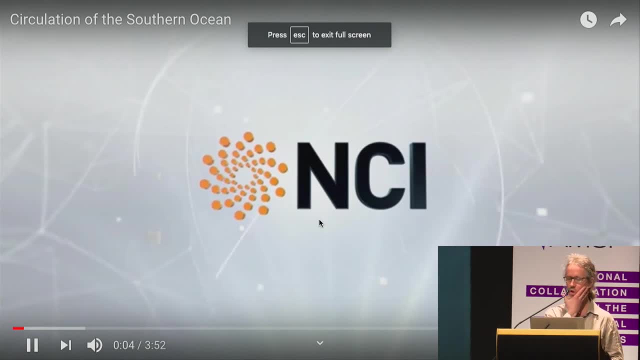 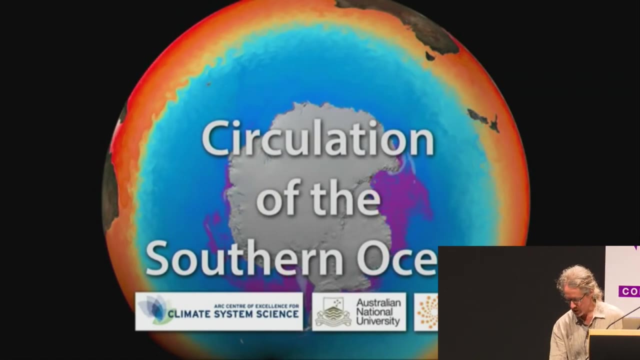 And so I would like to give a shout out to some of the work that's done here at in Australia, using models that I helped build in Princeton looking at circulation in the Southern Ocean. So here's Antarctica, Here's sea surface temperature. 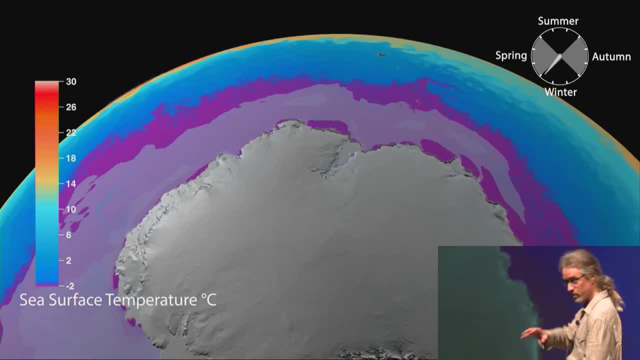 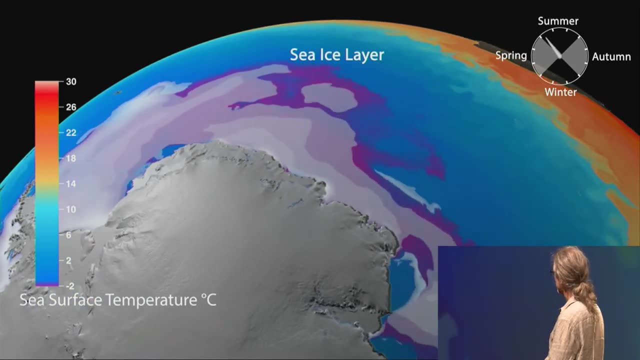 So this is a circulation model very similar to the one that I showed you, where we looked at the big patterns of surface temperature, the Gulf Stream and all that stuff. What we're going to show you here, that's a little bit unique, and why I like this animation. 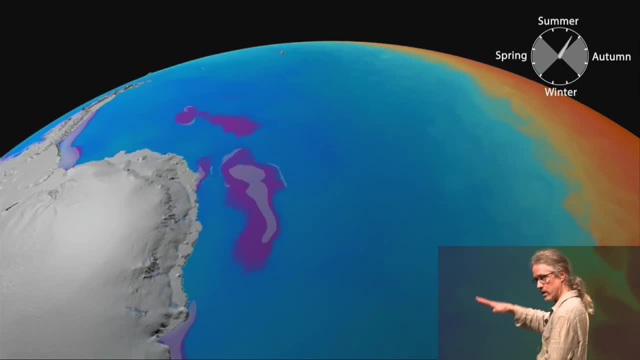 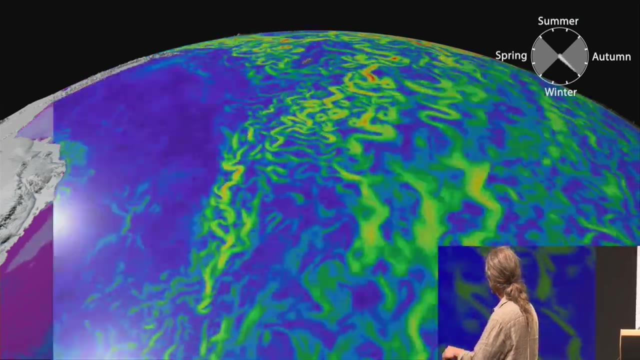 is. we're going to dive into the ocean a little bit to show you what's going on in the interior, around the continental shelf of Antarctica. So just give me some time. here We're going to first show the speed and see all this flickering. here is a fast waves. 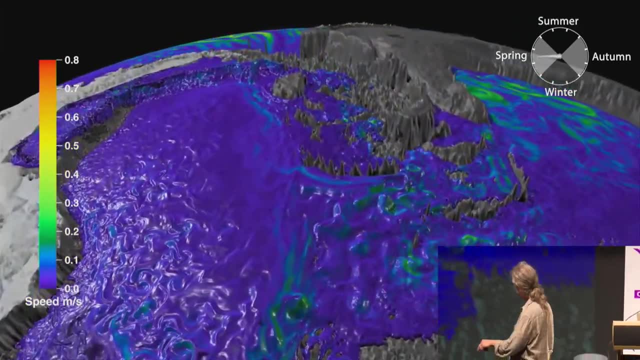 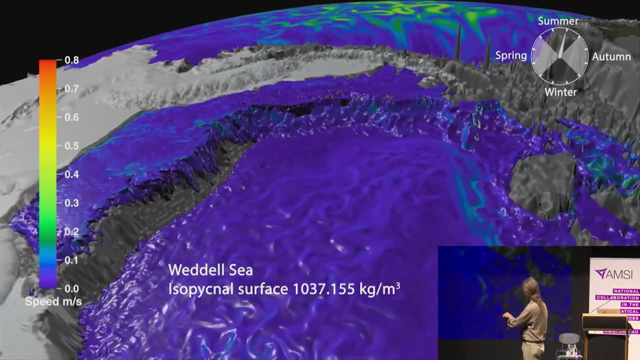 because of the winds. and now we're going into the interior of the ocean here, Looking at the speed and lovely patterns along the continental shelf and off the edge of the shelf and you see these patterns of water spilling over like waterfalls underneath the ocean. 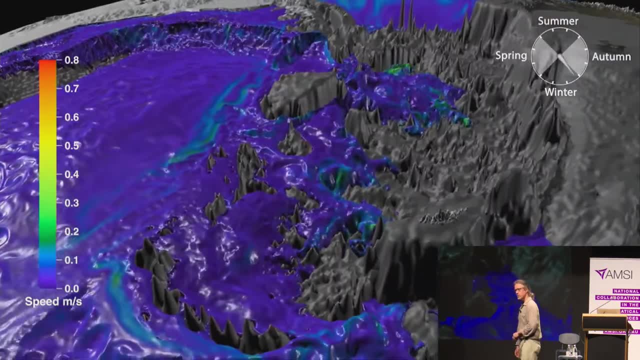 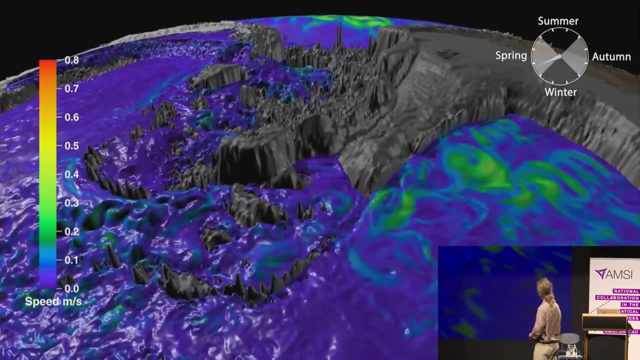 you know, underneath waterfalls That's creating some of the densest water on the planet. well, the densest water on the planet is these features falling off the cold shelves into the deep ocean And you have a nice clock up here. 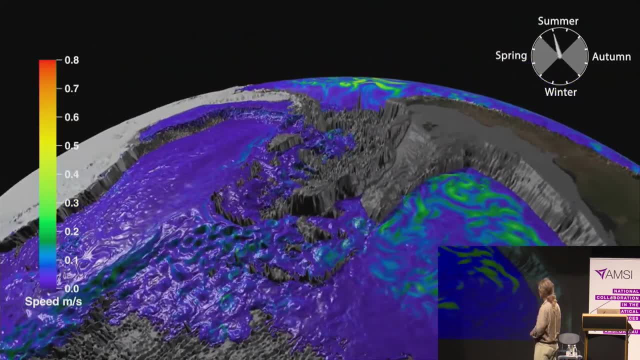 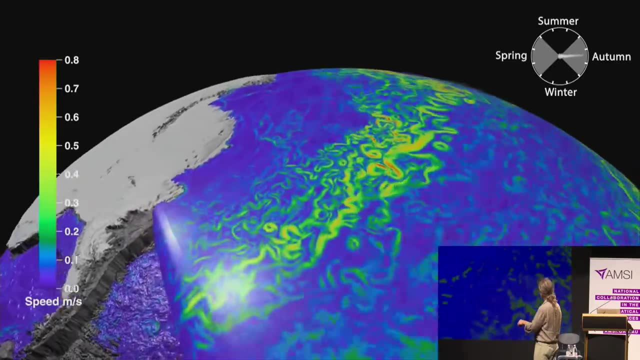 Springs, Summer, Autumn, To give you a sense for the seasonal cycle. down there, In the wintertime, of course, there's sea ice that we're not showing in this image. here And now we're back on the surface and we're going to come up here to. I believe the next is 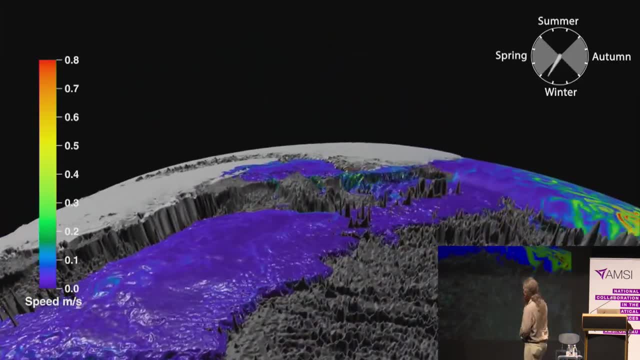 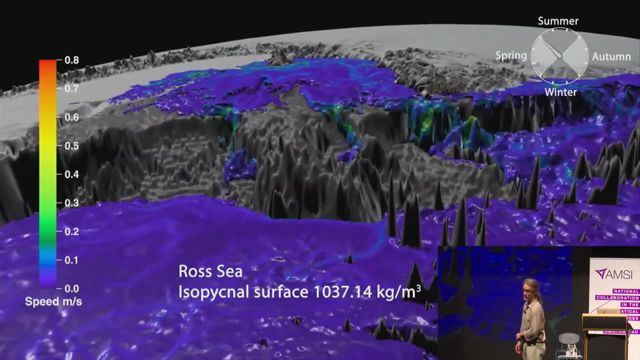 we're going to start to slice through the ocean looking at these density surfaces. Now we're looking here. I think this is the Ross Sea. Yeah, the Ross Sea. isopignol, that's just a buoyancy surface or a density surface. 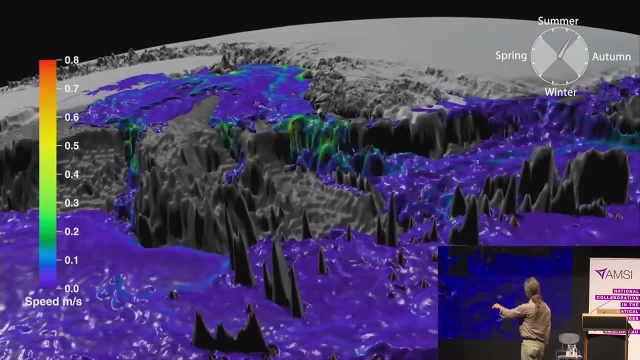 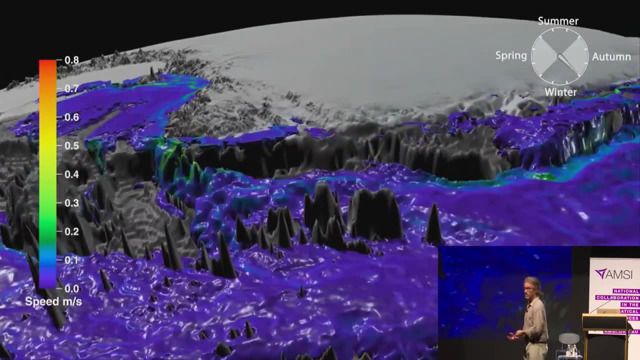 of a particular class here, a particular density class, And you see all this rich activity of water moving into the interior of the ocean. You may think that's simple to simulate, but it actually is not a simple thing to simulate in these models here. 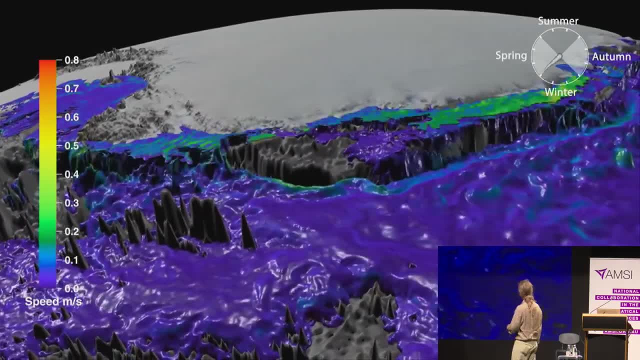 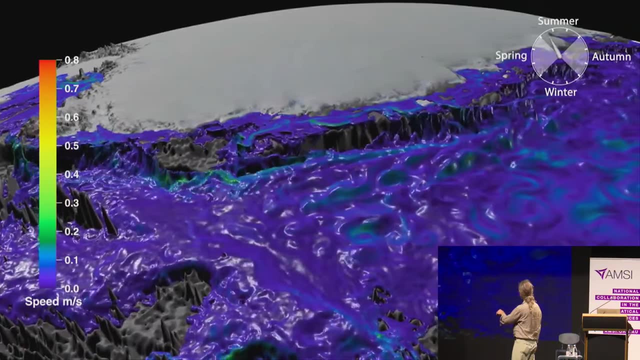 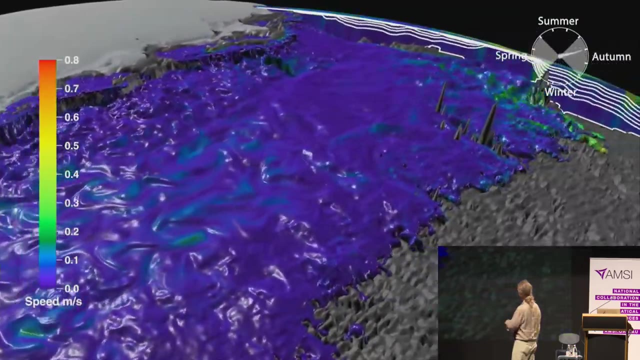 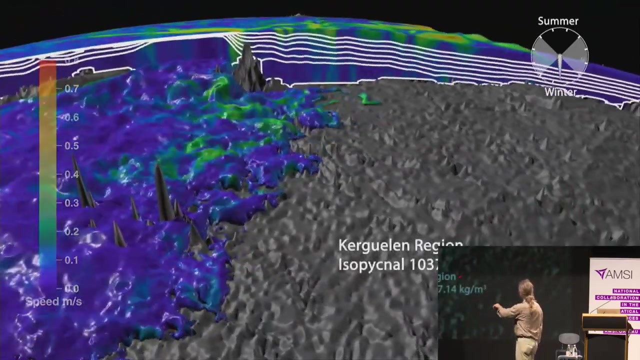 And this is quite a pioneering effort here that's been done with these simulations. So these patterns. here are some of those mesoscale eddies that I mentioned before, And now look at the density structure here. So you can see that if we're moving through the interior here in the Kerguelen region, 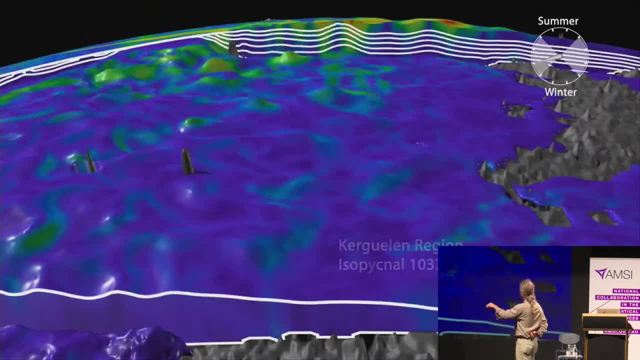 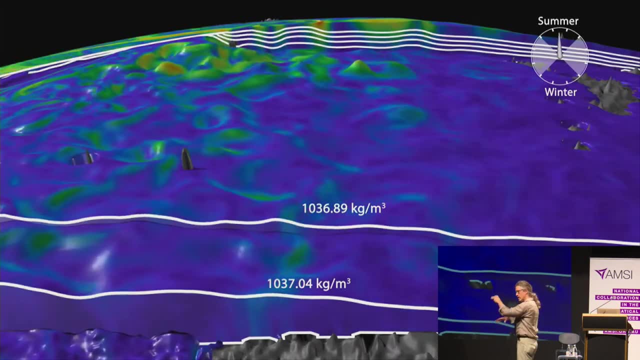 which is South Pacific, South Indian, and we're seeing patterns of these eddies, these undulations on these density surfaces here moving up and down. they create up and down motion on these surfaces, undulations, And so we're getting the different density classes here. 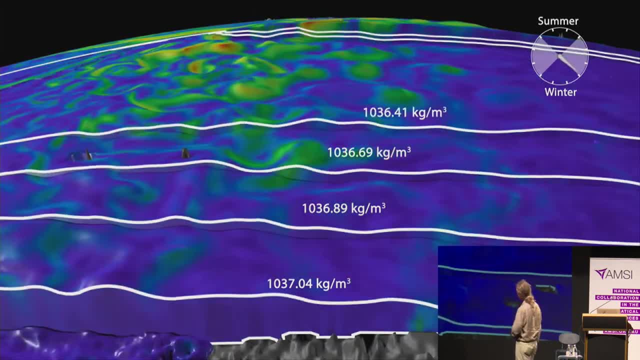 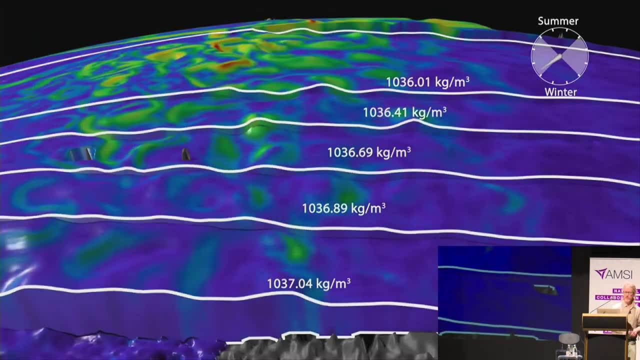 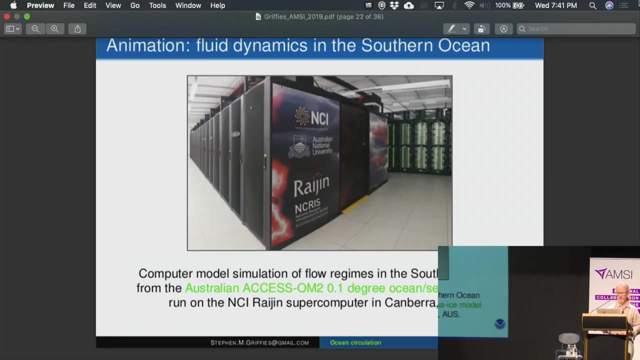 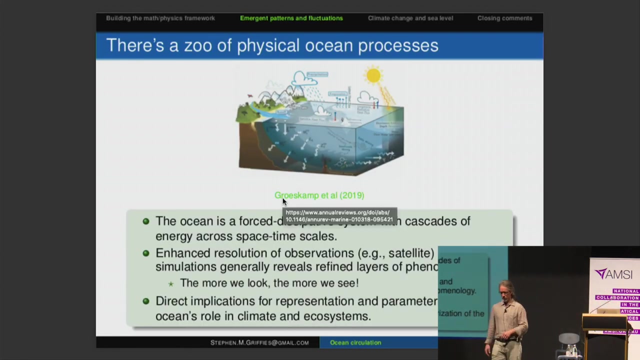 going into lighter water as we're moving more toward the surface. That's probably about the equivalent. Yeah, Yeah, Yeah, To the extent that I want to look at that simulation. So the ocean is a zoo. There's a zoo of processes that go on in the ocean. 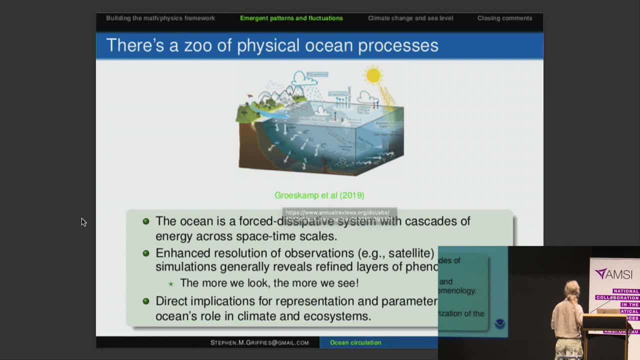 Lots of things. Groskamp et al. Get away, Get away, Get away. All right, This is from a. this is an image from a paper that short Groskamp led It's. I'm sorry it's so small. 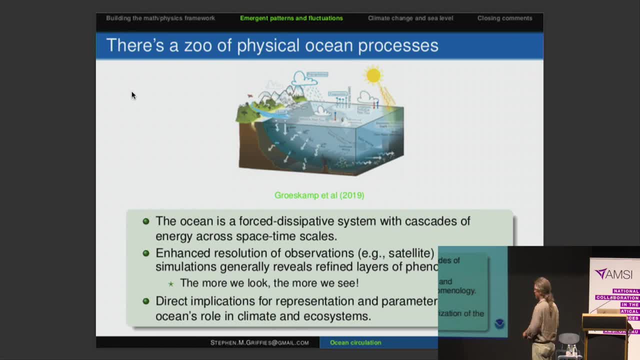 But I couldn't get everything to fit. There's a lot of stuff going on that creates phenomena in the ocean: emergent phenomena, Lots of mixing events, Lots of turbulence, Lots of eddies, Lots of currents. The ocean is a forced, dissipative system. 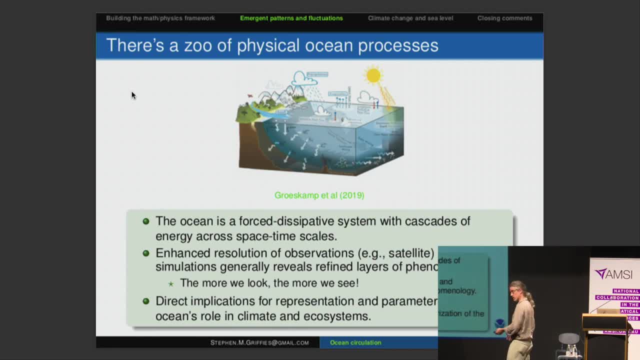 It's largely forced at the boundaries and dissipated also largely at the boundaries and in the interior as well. But mostly, you know, if you idealize the system, the ocean, as a physical system, it's a, you know, a spherical cow. you know, you idealize it's mostly a forced, dissipative system. 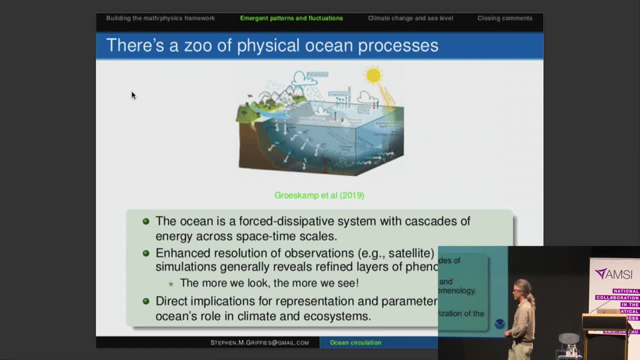 with dissipation and forcing at the boundaries. enhanced resolution of observations and satellites, for example radars and simulations, generally reveals refined layers of phenomenology. Now, some of you may have taken some physics classes and heard about the desert of stuff between the standard model and the Planck scale. 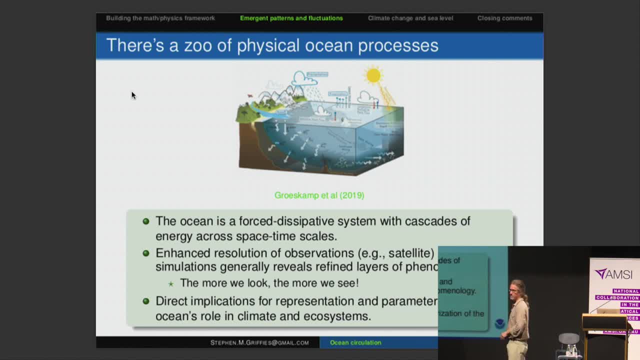 It's hard to know whether there's anything there or not, But there's. there's predicted to be a desert. There's really no desert that we can find in the ocean. There's layers and layers of different phenomena, And that has direction. 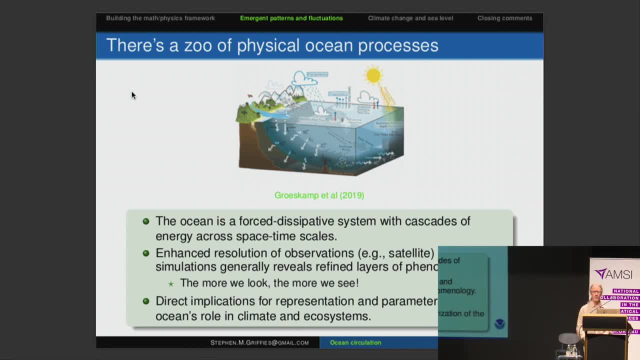 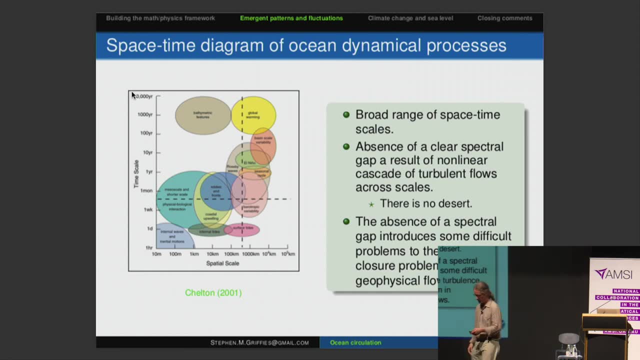 There's direct representation or direct implications for how we represent the ocean in simulations and how we, how we, how we think about the ocean. Here's another way to show the same piece of information. This is a space-time diagram with a spatial scale on the horizontal axis. 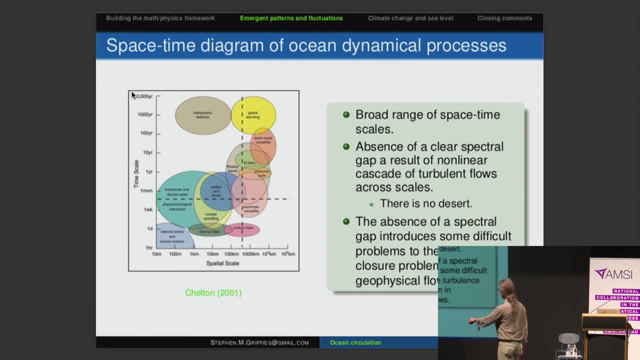 and a time scale. time scale on the vertical Down here is very fast processes and small processes starting at an hour and tens of meters here And on the on the high end you've got about ten to the third, ten to the fourth kilometers. 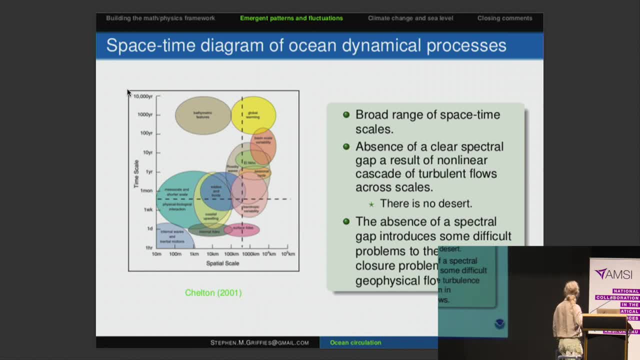 And on the scale, a piece of space Up here you've got many different, about 10,000 years. So starting from the slow scale and large scale, you've got the global warming scale, the general pattern of warming of the planet, here at the, the, the decadal to centennial scale. 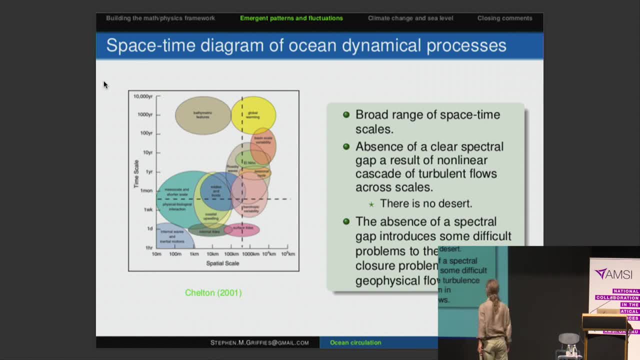 and at the planetary scale, At the fast time scale. you have small scale processes, acoustic wave, internal waves, And you have all different kind of processes that overlap. here There's no gap, There's no, here's a phenomena, and then you go space-time very far away. 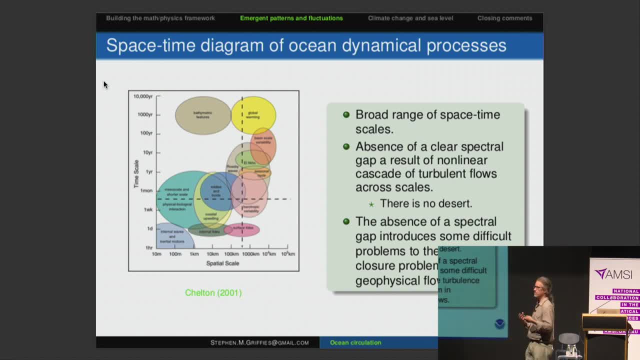 And so that is. it's a multi-scale, complex system, self-interactions that go across scale. There's a cascade of energy across space and time scale that make it very different to disentangle all this different phenomena, And that adds a lot of the richness and the the complexity to these partial differential equations. 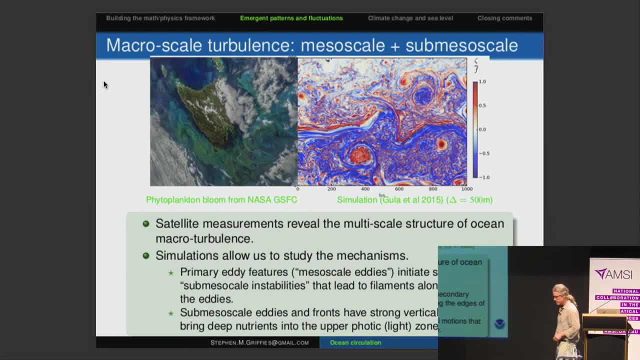 that we're trying to solve and simulate with, And this is a brilliant image that if you looked on my laptop, it would look even better. On the left, here is from a satellite. On the right, here is a simulation. This is Tasmania. 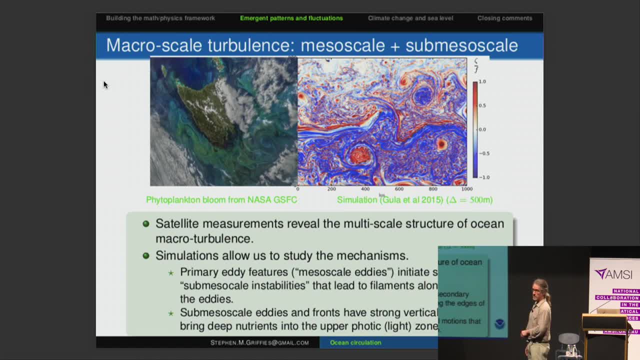 And for some reason Tasmania just always seems to come up in these NASA satellite images of the best image of the day because they have wonderful phytoplankton blooms that reveal eddy features, these whirlpools and and eddy features around the the. 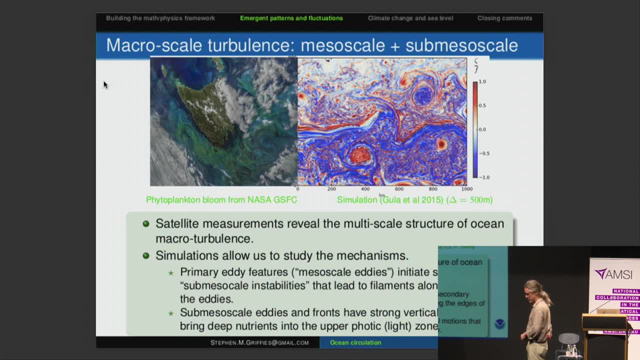 that little island down there. that are brilliant examples of of turbulence, macro turbulence of the ocean, the term macro turbulence, This is not turbulence of your coffee cup. This is not turbulence of your coffee cup, This is macro turbulence of the at the planetary scale. 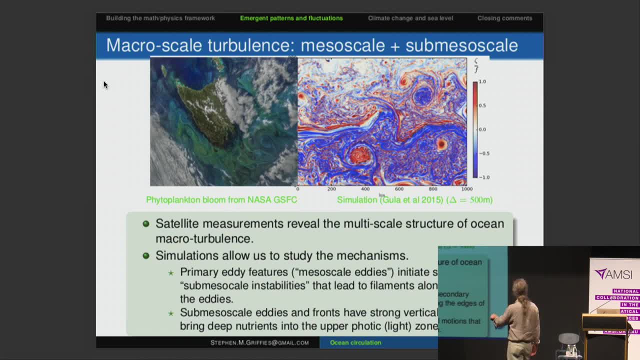 And here you have a simulation of scale. This scale here is- I don't know what that scale is, It's kilometers down there, So 10,000, or 1,000 kilometers- of a very high resolution model. I think it's got 500 meter resolution in the X and Y direction. 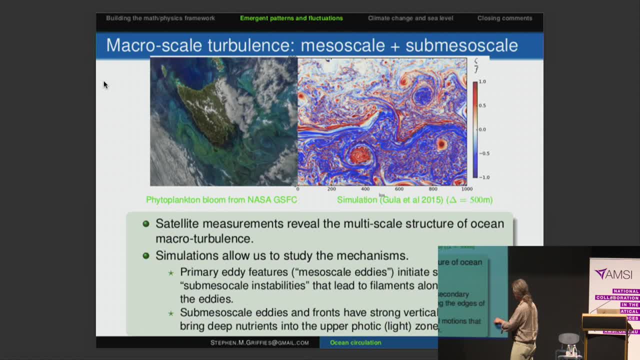 So that means each pixel is 500 by 500 meters and you've got 1,000 kilometers on the side. So there's a lot of grid points there And you get a, a simulation here which creates these jets and whirlpools and eddies. 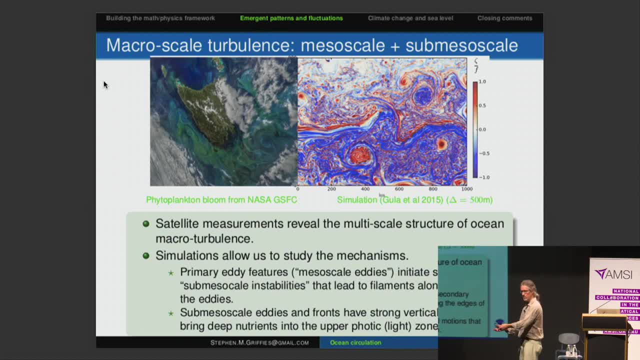 that cascade in filament and secondary instabilities acting on primary instabilities. So and the terminology we have for these, these modestly big size eddies are called mesoscale eddies and the fronts and filaments on the edges of the eddy. 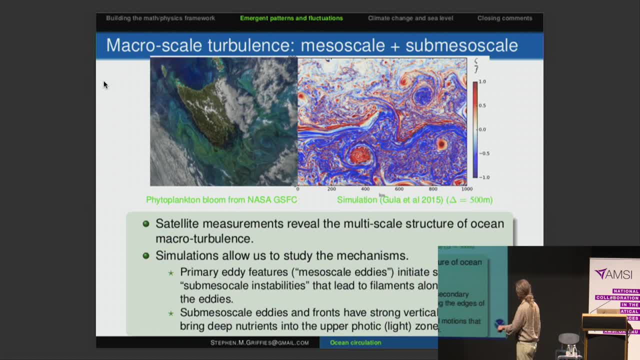 the mesoscale eddies are known as sub-mesoscale eddies And there is a big, big research area moving toward the, the, the regime between mesoscale and submesoscale. The submesoscale has very big impact in particular. 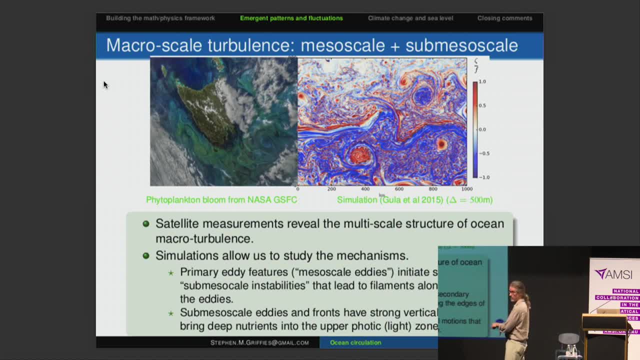 on nutrients in the ocean and so the biophysics. people are very keen to understand the physics and the biophysics of submesosceles because they bring a lot of nutrients from the intermediate depths up to the surface where they can get light and the fish and the other marine life. 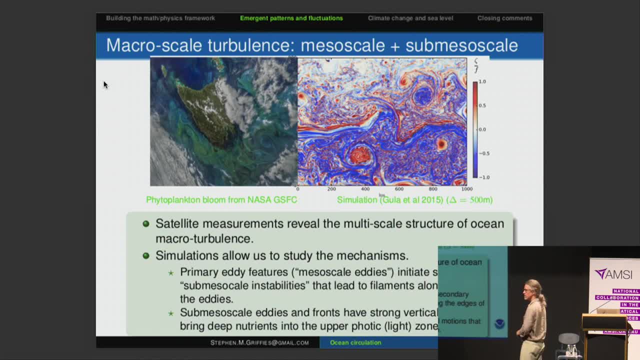 can act and eat on them. You actually have whales and people that go out and fish that follow some of these eddies because they prefer to hang around in particular temperature water and where they have a lot of biology activity, And the fact that we can start to 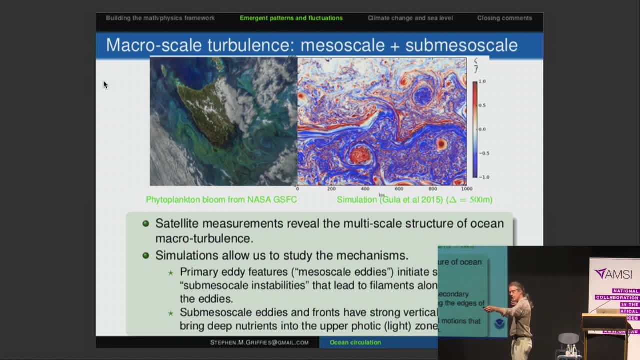 get models that represent that scale over a large region is phenomenal. We're moving into a new regime of our ability to simulate and to observe the planet, because we're able to simulate these different scales at a much bigger scale, at a much bigger scale. 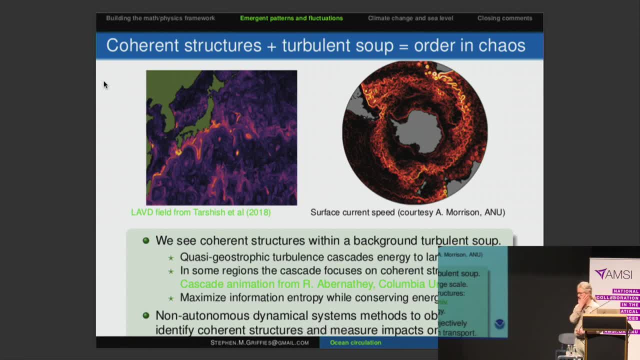 Subtitles by the Amaraorg community Over the planetary scale. Here's another image here of back to. it's too dark, I apologize. Coherent structures, so order and chaos, So turbulence in the atmosphere, in the ocean is not just like a box where you just shake it up and everything is just chaotic and there's. 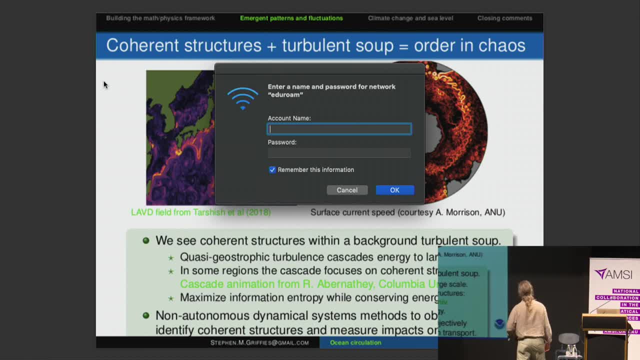 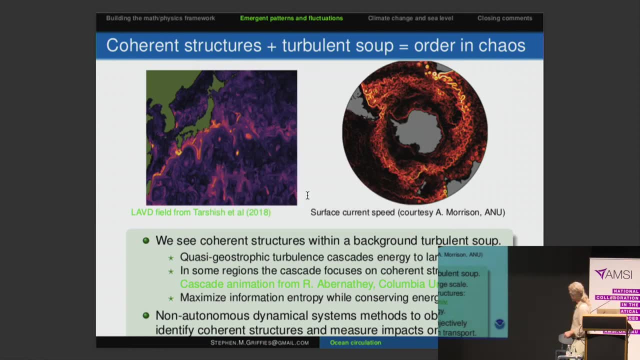 no order there. In fact, there's- oh shoot, Really All right. In fact, there's order that appears out of this chaos, And this is back around the Agulhas region of South Africa, where you see these beautiful eddies here in the simulation. 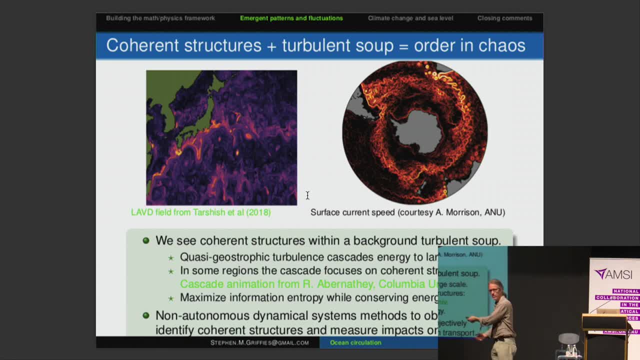 here that maintain their coherency over many, many hundreds of kilometers and over months and sometimes years of time, And I'm not even going to talk about that because it's too dark to see. The main point here is that the turbulence that we talk about in the atmosphere, 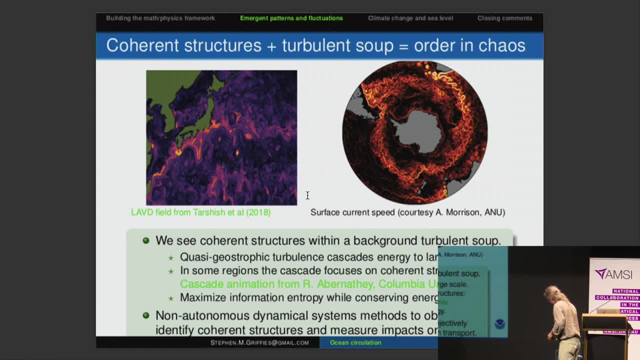 in the ocean. Subtitles by the Amaraorg community. the jargon term is quasi-geostrophic turbulence. there's a cascade of energy from the small scale to the large scale, And that's opposite to what we might experience in day-to-day life. 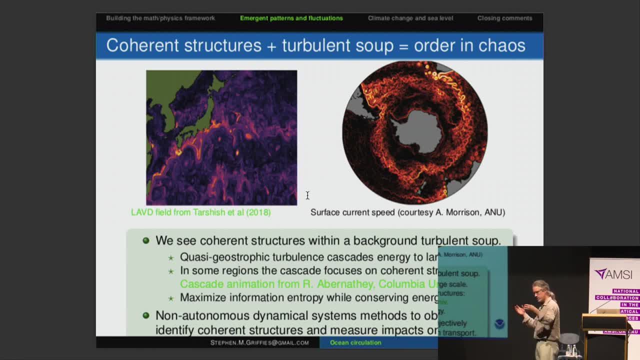 where you have a turbulent box where energy cascades to the small scale, And so it's an upscale cascade of energy that feeds into these large structures, that eventually gets stopped in these large structures and it sort of forms an object, a coherent object that stays around for a while. 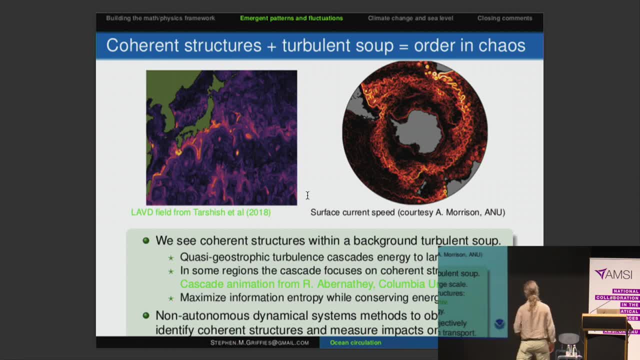 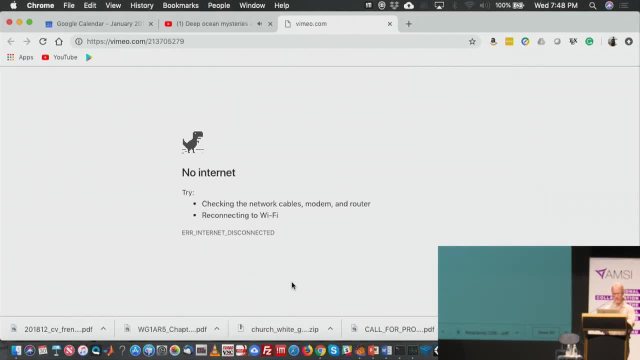 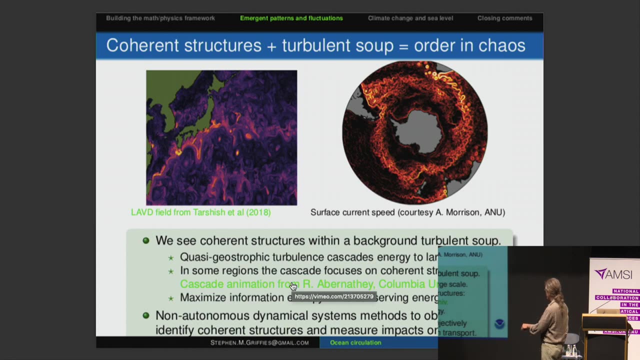 and creates some beautiful features in these simulations. So let me see if I can get on the Internet. Yeah, darn it. All right, I don't want to spend the time to re-log in to edge your room. Another area of analysis that is very important and very useful. 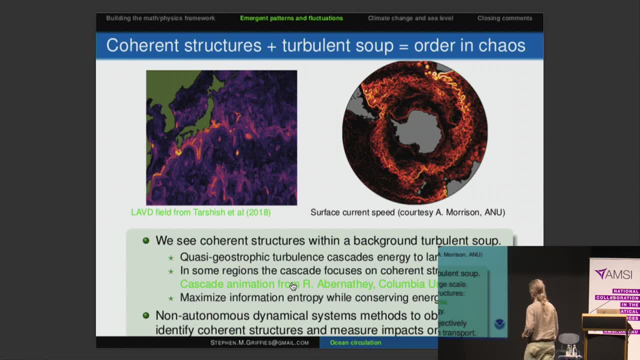 and actually some people here at UNSW. Gary Furlan, in particular in the math department, is pioneering some tools from non-autonomous dynamical systems to help identify these features, both in observations and in the ocean, and to ask questions about how important they are for transporting stuff. 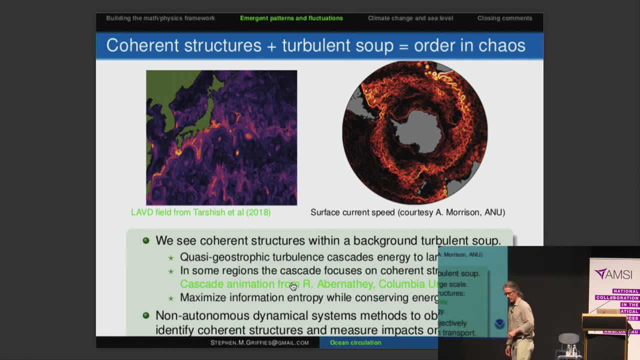 You can go and measure some of these eddies, and a colleague of mine in France, Sabrina Speich, does that with her ships and goes down and does sections through these eddies and sees these properties and the fish that like to follow them in particular. 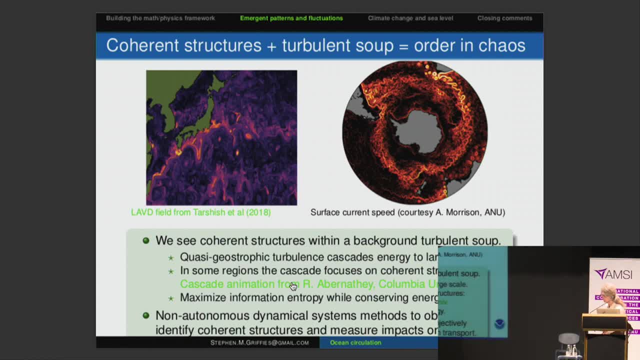 that remain reasonably safe. So it's really coherent for many, many, many, many months and for across most of the South Atlantic. Having said that, there's some new work- Ryan Abernathy in particular, this guy here that I have my cursor on- which is indicating that there's some questions. 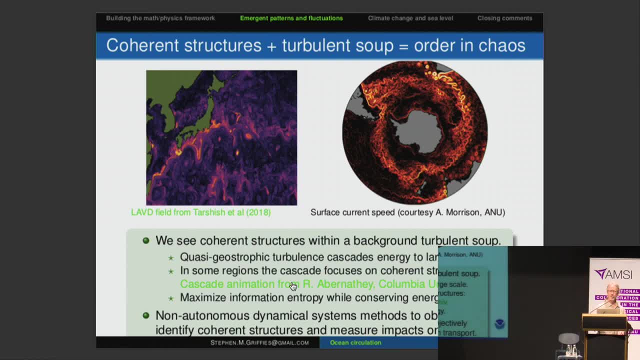 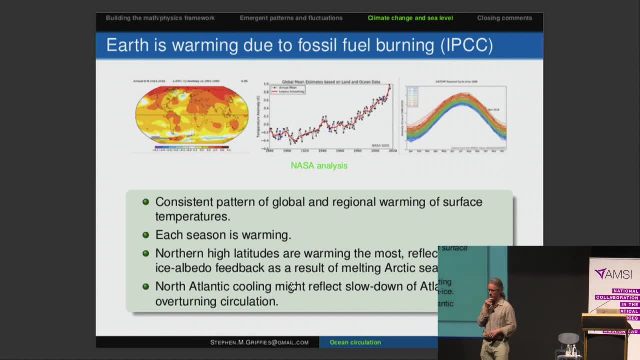 about how coherent those objects really are. So it's a cutting edge sort of research area that I like to play a role in. It's a really fun area because it involves some really deep theoretical questions about fluid mechanics. Now I'm jumping toward the end of the talk here. 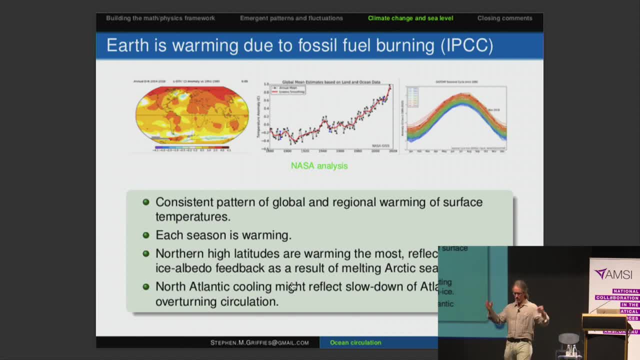 The last topic here is climate. So- and the elephant in the room- climate change. Earth is warming, humans are doing it, fossil fuel burning, all of that stuff. Here are, and so a lot of the work that I do at Princeton. 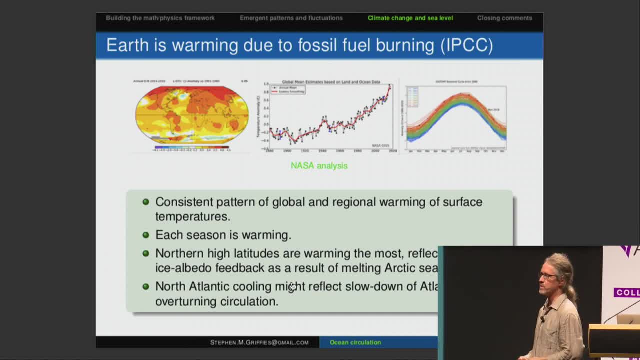 at Geophysical Fluid Dynamics Lab involves modeling the climate system, bringing pieces together. We started all the way back at Archimedes and moved through the equations for the ocean. similar things in the atmosphere. bring those two together, have a land model. 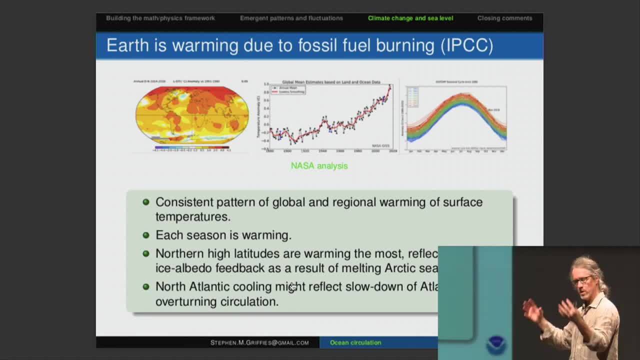 have a sea ice model? have biophysics bring those together into what's called a coupled earth system model? Those models are massive pieces of engineering science that have been created over the past 60, 70 years of bringing up the science and addressing questions. 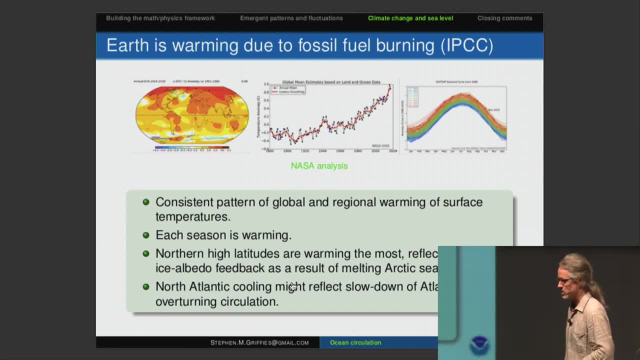 about climate change and it started, of course, in the 50s and 60s and 70s as curiosity driven work, and I feel, I still think, there's a huge amount of curiosity driven work that we need to keep playing, that we need to keep supporting. 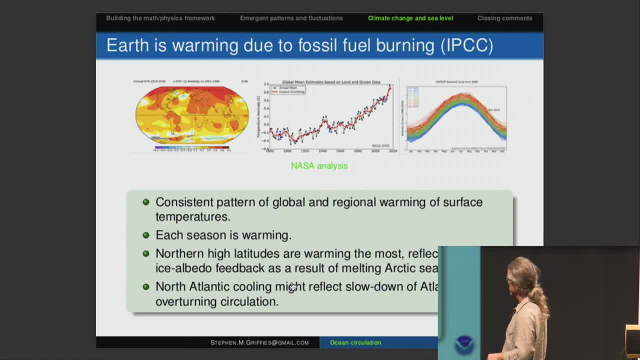 Curiosity driven science is the foundation for everything that we do in applied science, but there are some really big implications for what is happening on the planet today, and climate change in particular. So this is an image here, I think, of a five-year time mean surface temperature. 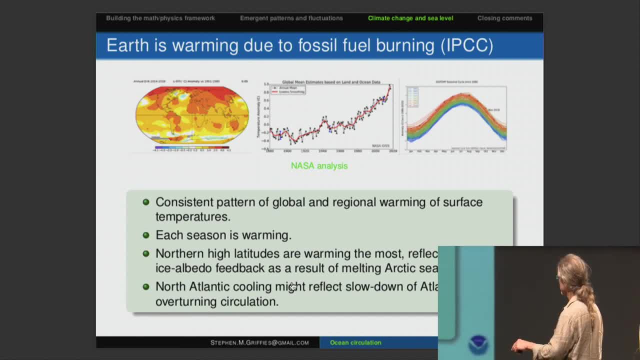 of the planet relative to 1980,, I think, or 19,, a few decades. You see lots of warming in the northern high latitudes, Some, some heat, Actually some slower warming and cooling in the southern hemisphere- not the southern hemisphere- in the Antarctic circumpolar current. 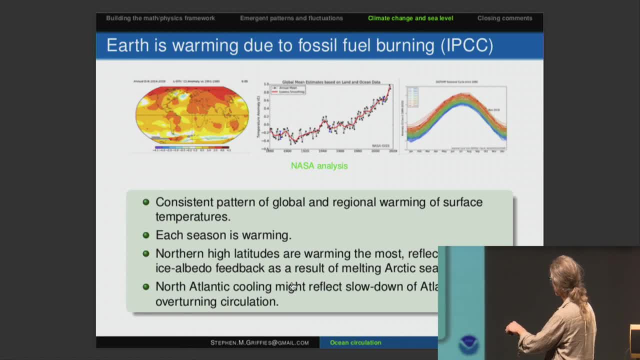 Global mean temperature on a rise. This is an image of the seasonal cycle: 1880 is in the blue, Present day is in the red. It just keeps seasons all just keep getting warmer, warmer, warmer. Interesting patch here in the North Atlantic. 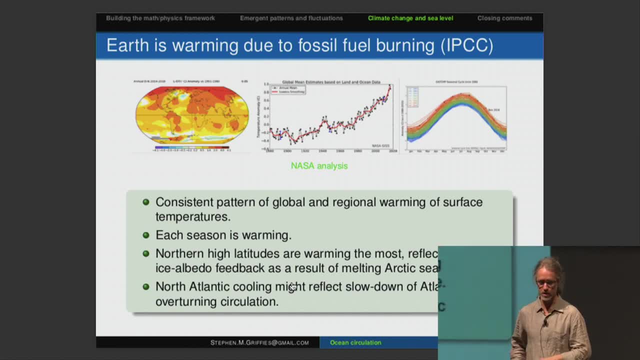 I'm going to come back to that. There may be some slowdown of the Atlantic circulation. It's contributing to that cold patch and I actually believe that that's really what may be going on there. The southern ocean cooling here or slower warming is. 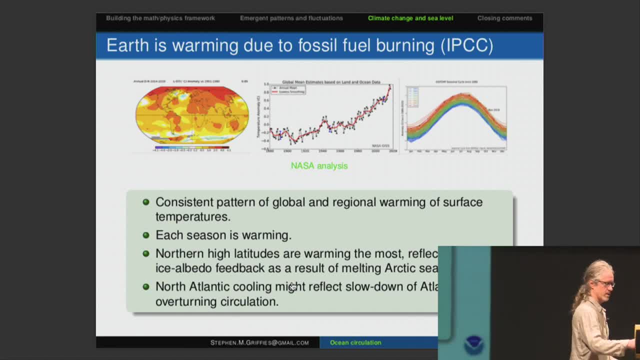 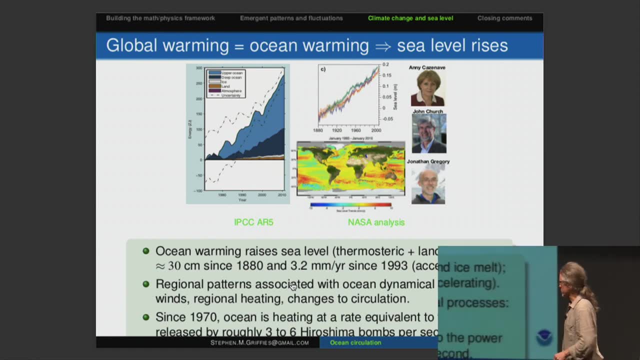 because the southern ocean is a completely different beast and I don't have time to talk about that in particular. but it doesn't discount global warming just because you have a couple of spots that are not warming. Ninety-some percent of the global warming is ocean warming. 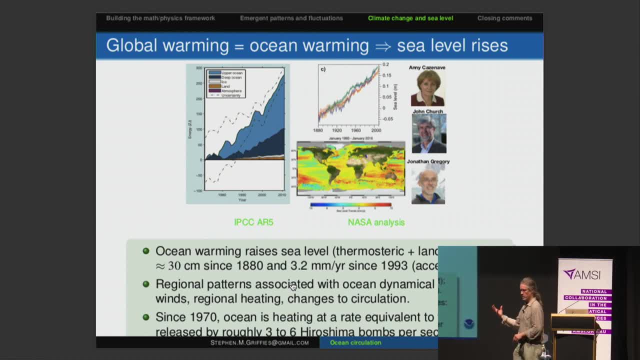 Global warming really is ocean warming, and that implies sea level rise. So I do a lot of work in sea level and these are three of my heroes: Annie Kazanov, John Church- another Australian at UNSW, and Jonathan Greger. 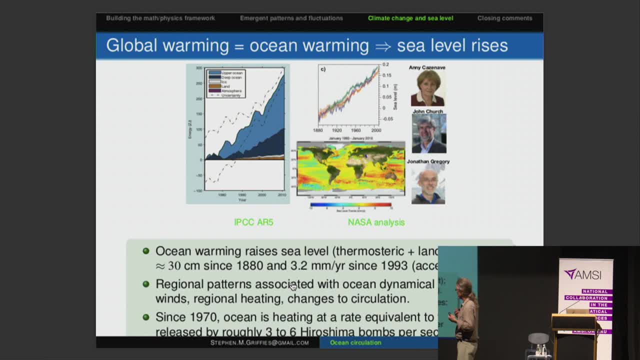 They just three- won a massive prize, which is really great that we're starting to get prizes, monetary prizes like the Nobel Prize for their work on sea level over the last 20 years, 30 years. A lot of the work that's shown in, all the work that's shown here is really 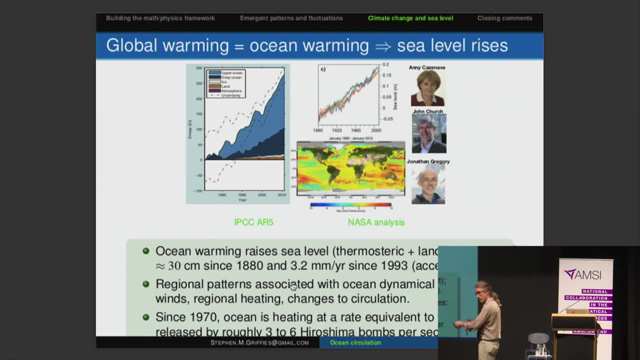 would not have occurred without these three efforts and a lot of other people, Of course, but these are the three champions. Right here you see a time series from 1880 to the early 2010s of sea level rise, with three different estimates all rising over the last since 1880,. 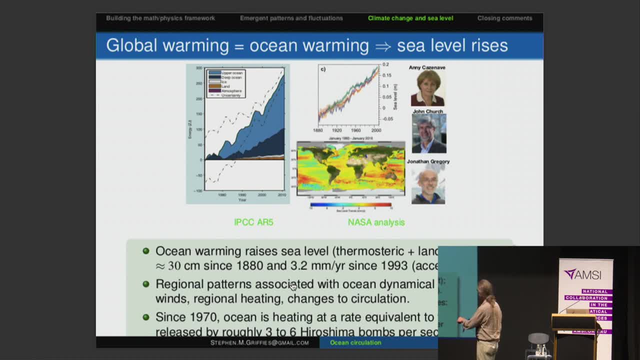 it's risen by about 20 centimeters global mean. This image down here is the trend from a NASA analysis of sea level, with global mean removed. okay, So it's just looking at a pattern where things are going up and down relative. 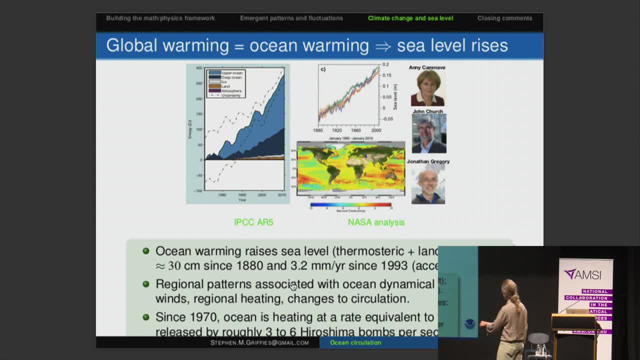 to the rising global mean on top of it. And you see, it's very inhomogeneous And that, from an oceanographer's perspective, is the interesting stuff. That's the stuff that you have to worry and understand because of ocean circulation changes. 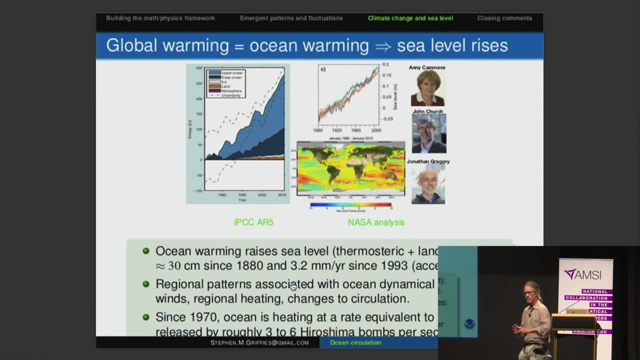 and different patterns of moving of heat around from one basin to the other across the basin. Some of the work that was done here with Matt England has looked at some of the heat movement in the Pacific that creates some changes in the sea surface height on one side of the Pacific relative to the other. 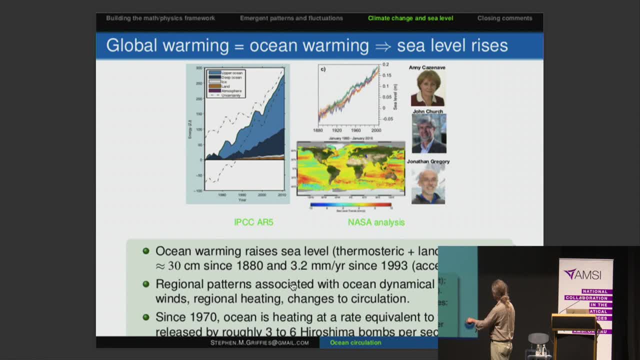 This time series here from 1970 to 2010,. this is the first time that we've done this. So the ocean is all. the blue stuff is where the ocean is absorbing the heat, And this little stuff down here is the atmosphere in the land. 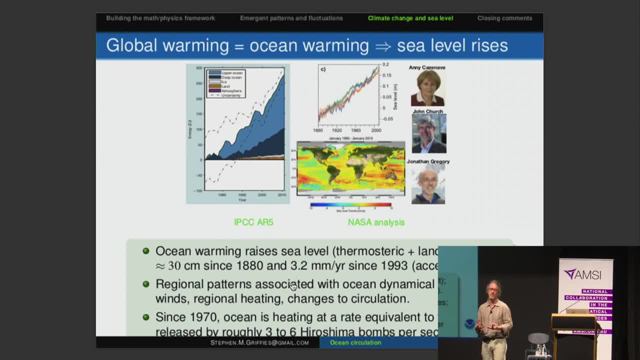 So the ocean has a huge capacity to hold heat and that's why it most of the heat that is stuck in the planet eventually gets absorbed by the ocean. So the ocean is doing a huge service to the terrestrial life here. but of course we have sea level rise and we have ocean warming, which affects the marine life. 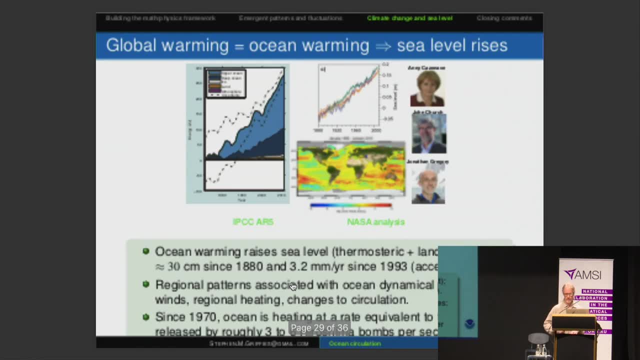 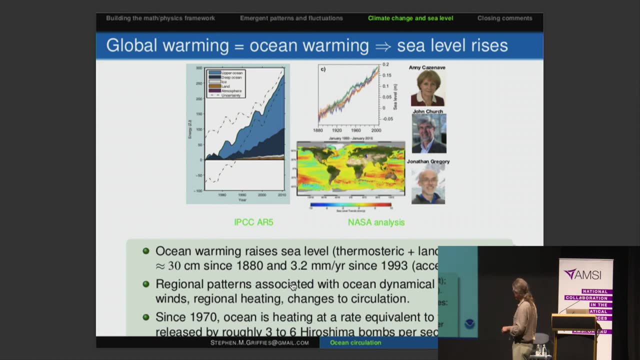 What did I say down here? This is a sort of cocktail party thing to share with your friends. that, to give you a sense, The ocean, the atmosphere, the climate has warmed by about a half a watt to a watt per meter squared. 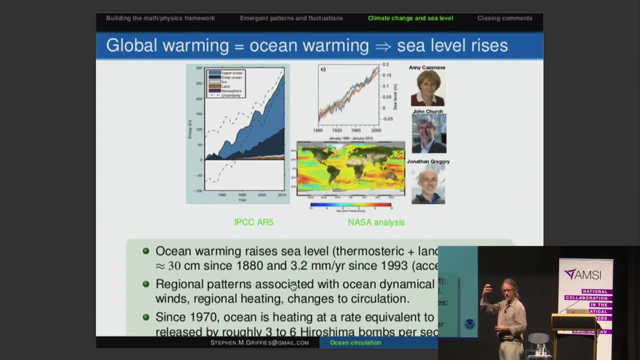 So these lights here that are blaring in my eyes are a lot more energy, a lot more power than that. You think. what's a watt per meter squared? That's really tiny, But if you accumulate that over the planet, you multiply by the area of the planet and you ask how much. 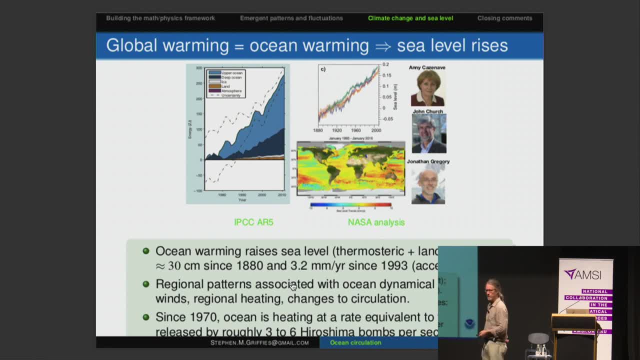 of an area of the planet. does that mean An atomic bomb? the energy released from blowing up an atomic bomb? Besides, forget about the radiation and all that stuff, just the energy content. So the energy that's gone into the ocean since 1970, if you do some back of the envelope, 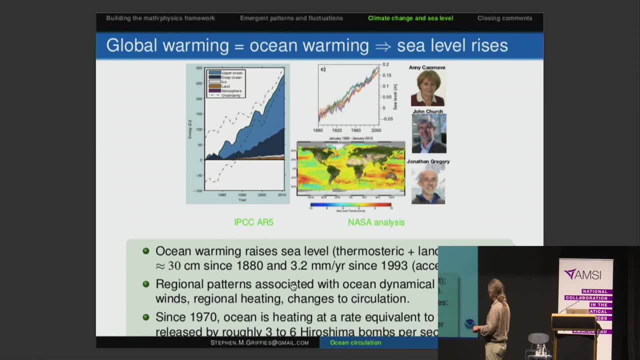 really back of the envelope. very rough calculation is roughly equivalent to about three to six Hiroshima bombs per second. That's how much we're putting in with that extra heat due to climate change, due to fossil fuel burning that we're putting into the ocean, relative to what was done before. 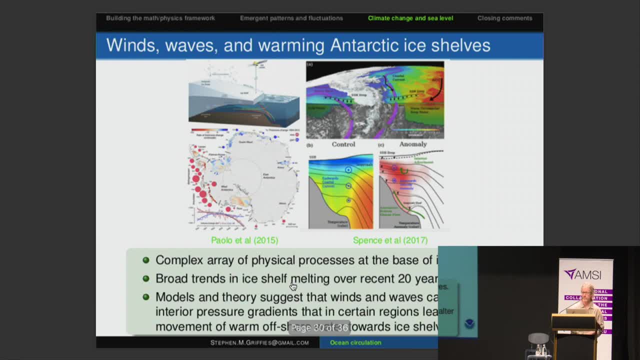 So that gives you an idea, So that gives you maybe some context for what's going on. Here's some work that is more detailed, but nonetheless let's show it. Here's an ice shelf. Big question around Antarctica is: are these ice shelves going to melt? 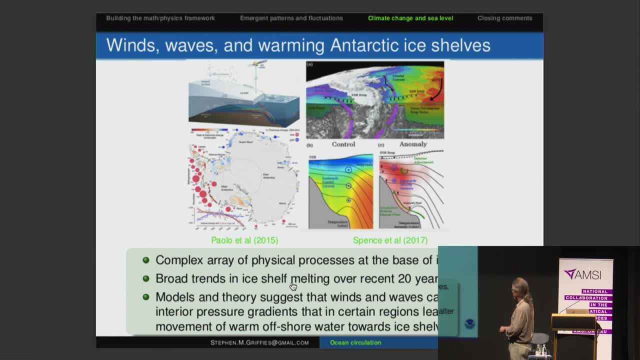 And the reason that they could melt is largely because of imposing warm water from off the shelf to the base of the ice shelf is a huge research area that's ongoing around the international in fact region and in fact Australia in particular has done a lot with UNSW and other areas of Australia. 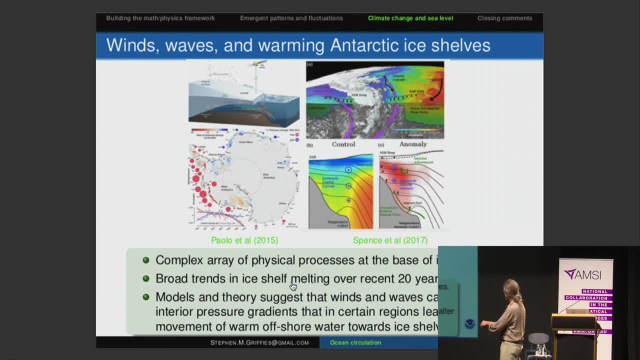 This is an image here of all this red stuff here means you're getting ice shelves melting. This is data, an observation from Paulo et al 2015.. Lots of red spots around the continent, some blue, but mostly red. And this is an image from a study that Paul Spence led, which had a lot of people here at UNSW and myself included. 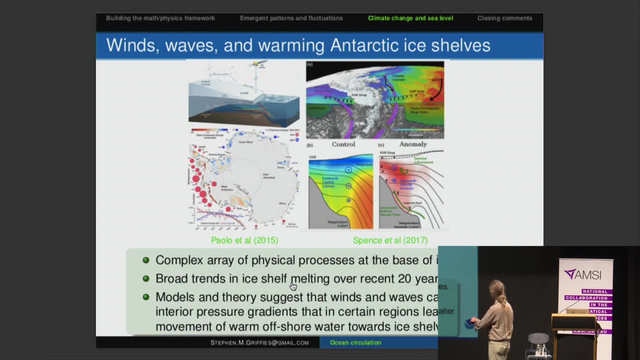 that I won't go into the detail. It talks about a mechanism in a model, in a theory that could bring some of that offshore warm water toward the ice shelves, based on changing wind patterns, And so there's a lot of effort in our community to understand different dynamical mechanisms. 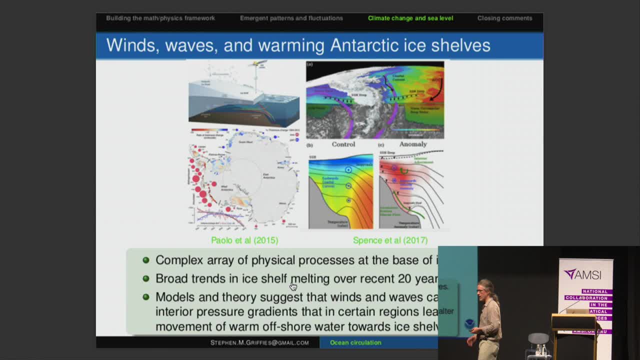 to potentially bring more warm water to the base of the ice shelves, because if you crack off that ice shelf it floats away and then more ice from land will come there and that will change sea level when you bring more land ice to the ocean. 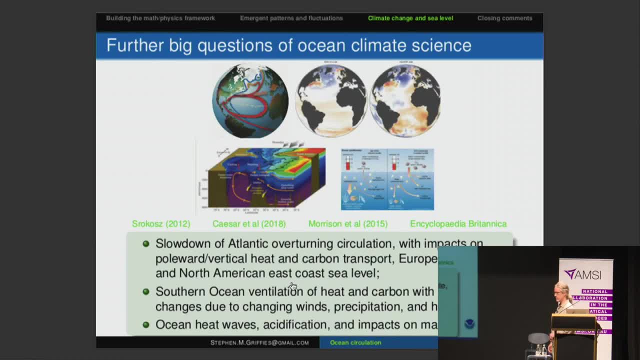 There are lots of big, big questions that are being addressed by climate modelers, climate scientists, oceanographers, and here's just a few. So the North Atlantic has a circulation called part of the Great Conveyor Belts, overturning circulation, different features. 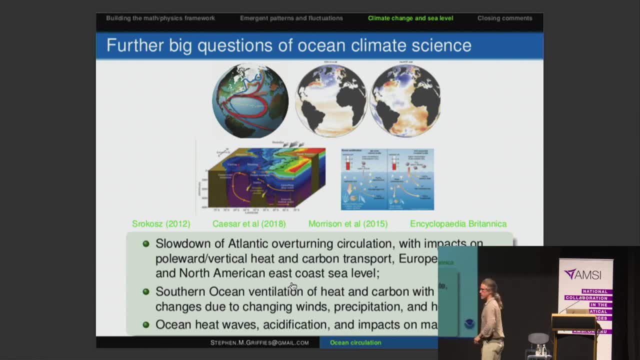 The Gulf Stream is part of that. The question is, is that circulation going to change? and if it is, may be changing now. So what you have in this slide is a lot of information. So this middle picture here is an image of the sea surface temperature change. 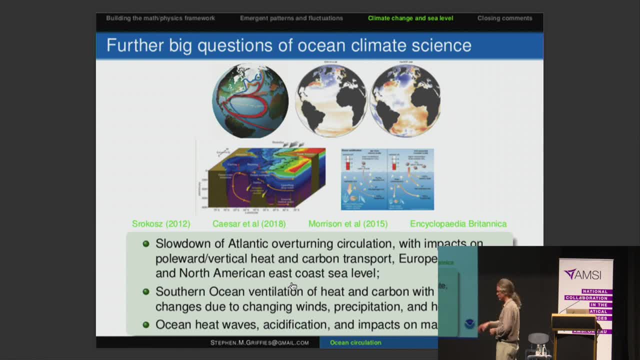 from a climate model, the climate model that I showed you, the image from the beginning, starting from the Manhattan, And here is an image from observed, the best of the observed, And so the pattern is very similar and this is a fingerprint, This cooling in the North Atlantic which I talked about with that sea. 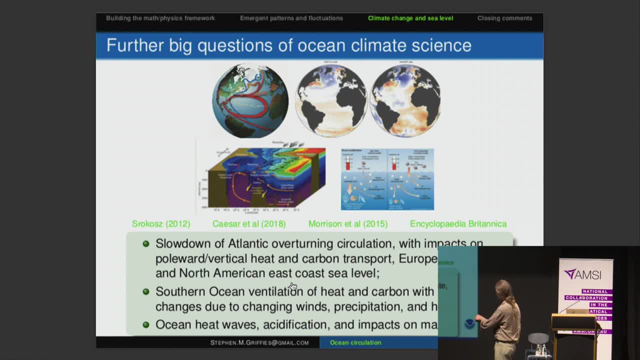 the surface temperature, having that cold patch and this warming off the coast of the east coast of the US. that's a very important fingerprint of climate change. or, for example, the climate change in the North Atlantic. So the climate change is a very important fingerprint of climate change. 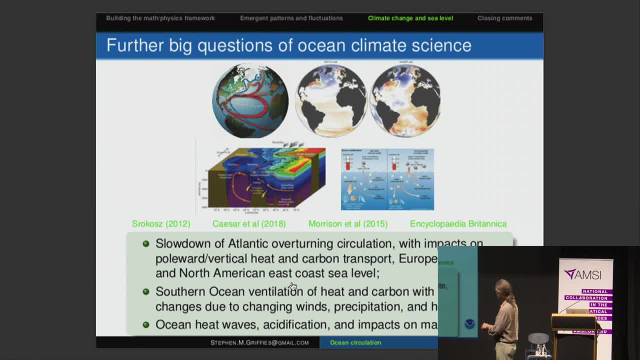 or, for example, the climate change in the North Atlantic or fingerprint of the slowdown of the Atlantic circulation, Turns out that that warming pattern off the east coast of the US creates, is also creating part of a sea-level rise along the east coast of the US, And it's the east coast. 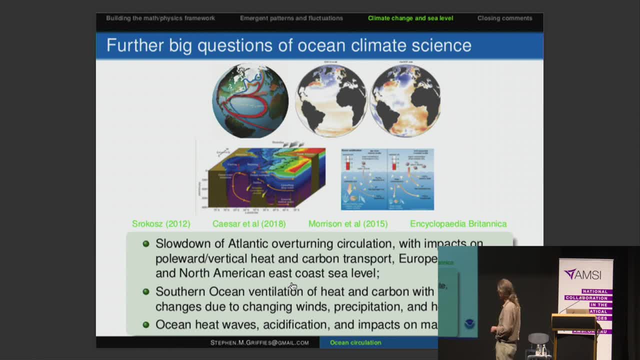 of the US is perhaps the hottest spot- hot in a sense of sea level rise on the planet. Another big question that we are looking at in climate science. it involves a lot of the dynamics around the southern hemisphere and around Antarctica. 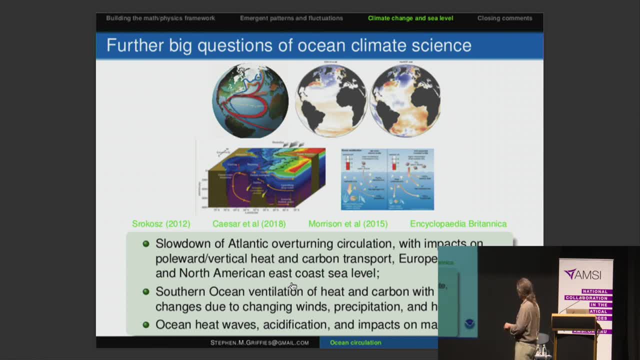 and I talked about that with sea-level rise. rise and the ice shelves, and one that involves chemists and biologists- is ocean acidification. you put more carbon into the ocean, even if it doesn't warm. you change the pH of the ocean, you change the biology of the ocean and it 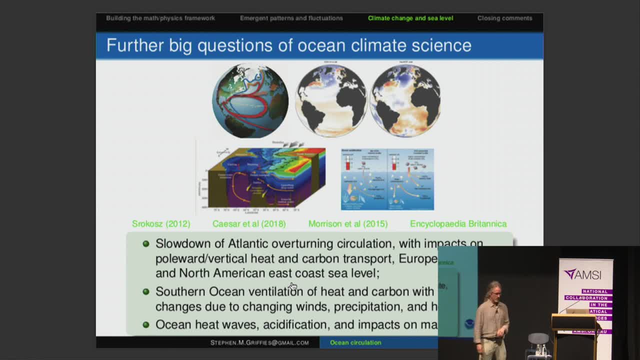 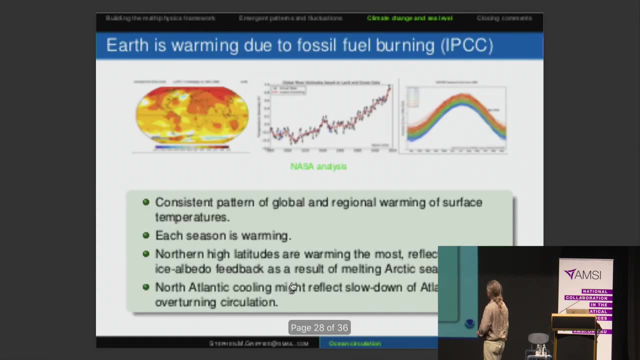 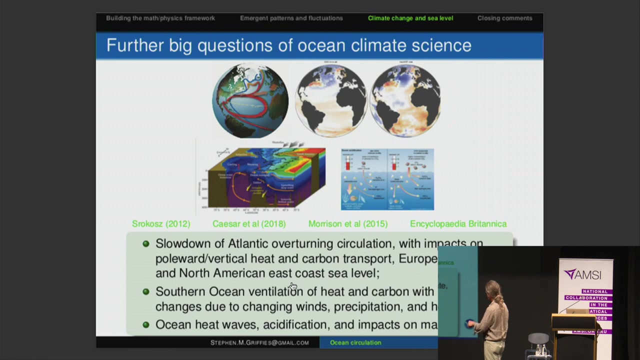 turns out that you start to start to um. a lot of the, the shellfish, the, the small shellfish at the base of the food web, start to dissolve. when you get a little bit more acidic, you have other processes known as heat waves shoot, sorry ocean heat waves. east coast of the us is again another place where the Gulf of 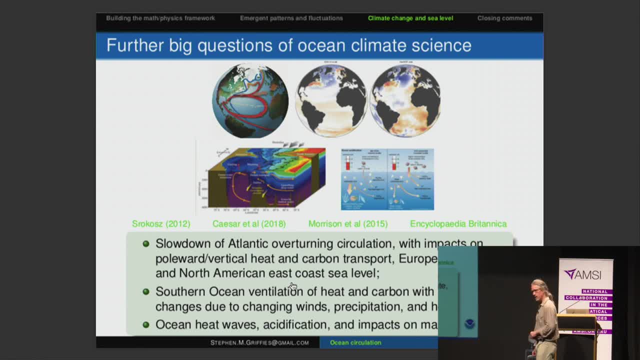 Maine has warmed more in the last few decades than 99% of the rest of the oceans and that's affecting, of course, the marine life there. acidification and effects on marine life. so, coming to the end, closing comments, trying to summarize a little bit, and I 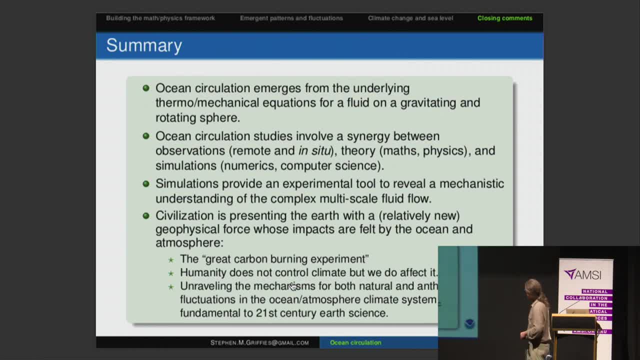 know this is a whirlwind and I appreciate the patience in the audience. ocean circulation is emergent from the underlying thermo mechanical equations for fluid on a gravitating sphere. ocean circulation studies involve a synergy between observations remote and in situ. in situ means in place, on a ship and on 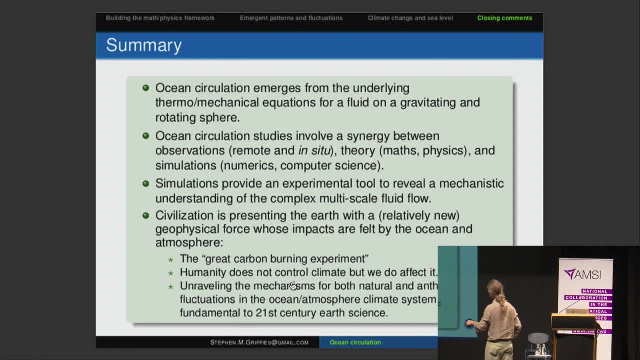 a float remote is from a satellite or radar. theory, Maths and physics- all about the stuff that you've been studying the last month- And simulations, numerics, computer science. So there's a huge community of people and, for the most part, we really are a community. 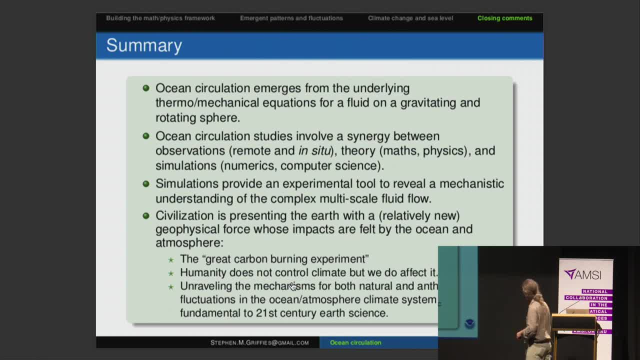 It's a very friendly community, a very vibrant community, an active community. Simulations provide an experimental tool that reveals mechanistic understanding of the complex, multiscale fluid flow. You cannot do experimental science, controlled experimental science- with an environmental problem. You can change it and we, you know, with humanity's great carbon burning experiment, we are affecting climate, but we don't control it. 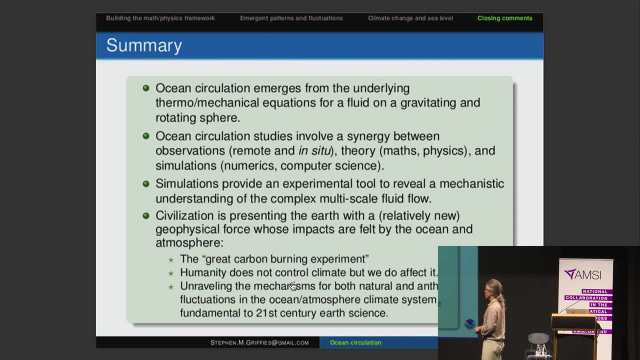 It's way out of our control And so the best way to do science to study these systems, just like astrophysics and cosmologists, you do simulations And the tool is as good as the tool is good. So we work a lot on. 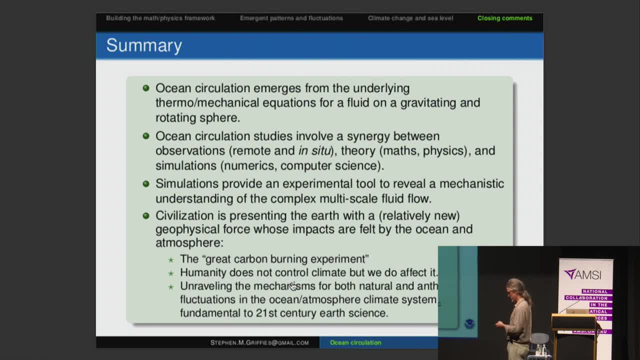 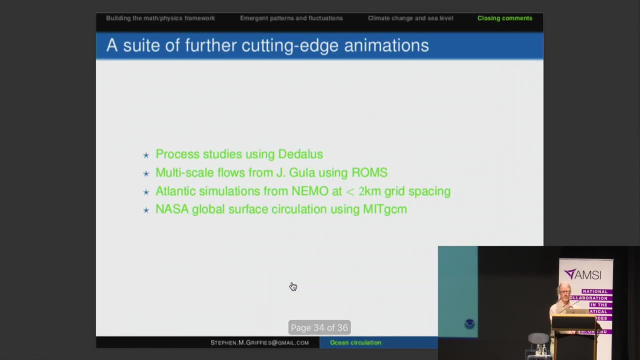 Making the tool better and then looking at the emergent stuff coming from it. Unraveling the mechanisms for both the natural and anthropogenic fluctuations in ocean atmosphere climate system is fundamental to 21st century climate or earth science. So I don't know if any if this talk is going to be made available, but here's here's some links to a number of other very inspiring simulations and animations that 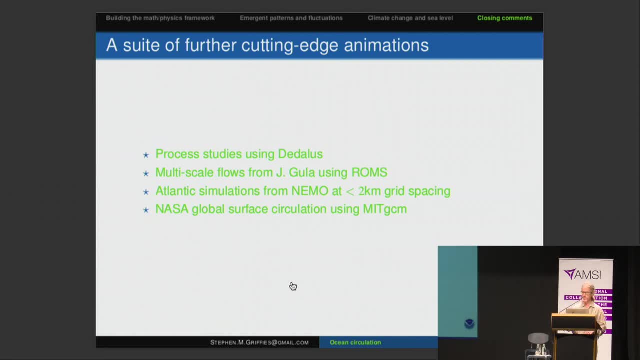 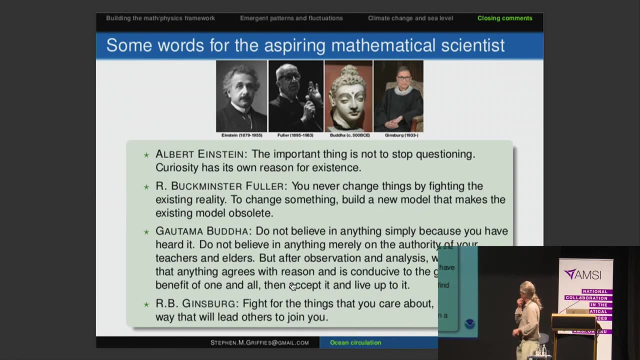 that some of you may also have heard about like to poke at. you can do some Google searches, but it's nice to have some, some hints as to where to go. so closing words for the aspiring mathematical science: you know there's a lot out there. you could google and a lot of this talk was 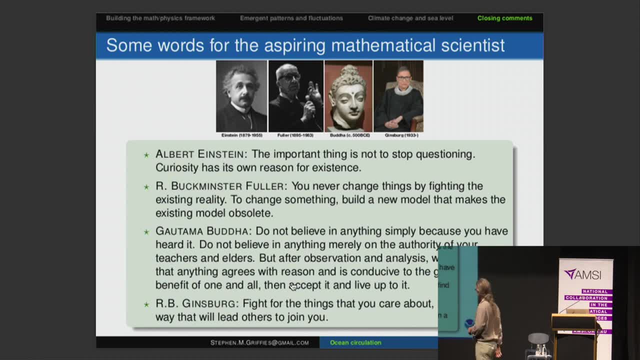 googling, but here is. here is some of the the things that I I like from some of my heroes. the important thing is not to stop questioning. curiosity has its own reason for existence, and so, in the process of doing science and mathematics, you've driven, I'm driven. lots of people are driven by curiosity. 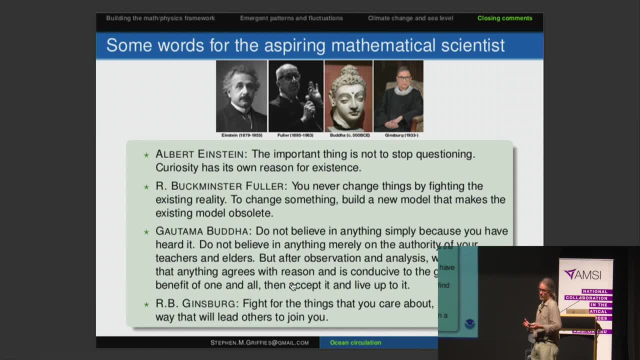 and it's important to pursue your curiosity stream and because most of the great understanding, the fundamental understanding, came from people just being curious and having the tools and understanding and ability to pursue that curiosity and help answer those questions that they may have had you. another hero of mine is Buckminster Fuller: engineer, mathematician, geodesic. 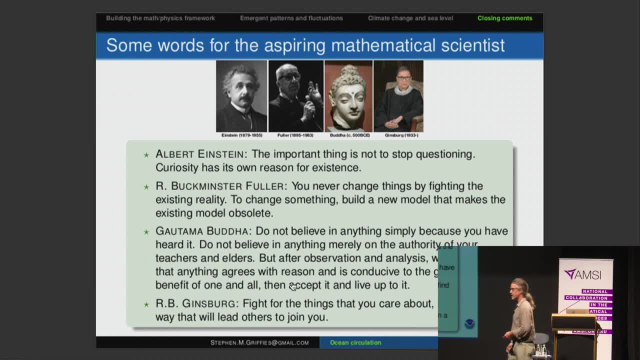 dome inventor. crazy guy. if you ever watch a YouTube of him, he'll stand there on the. you know he gave lectures. he went. he went around the world hundreds of times giving lectures. he would stand at the place like this for about five minutes in silence, just walking back and forth, thinking, and then he would just 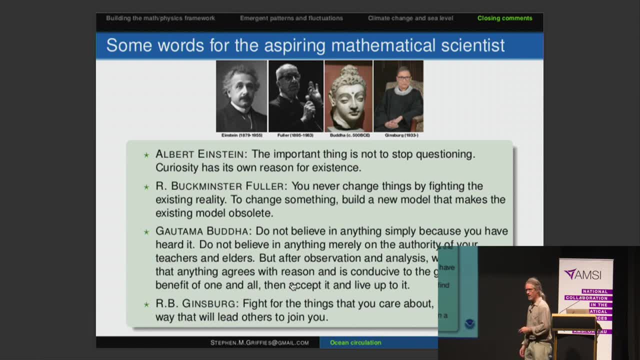 explode with thoughts. terrible speaker in the sense that you had a hard time understanding because he talks so fast, even faster than I do. you never change things by fighting the existing reality to change something, build a new model that makes the existing model obsolete. so if you do research, you're gonna, you're gonna. 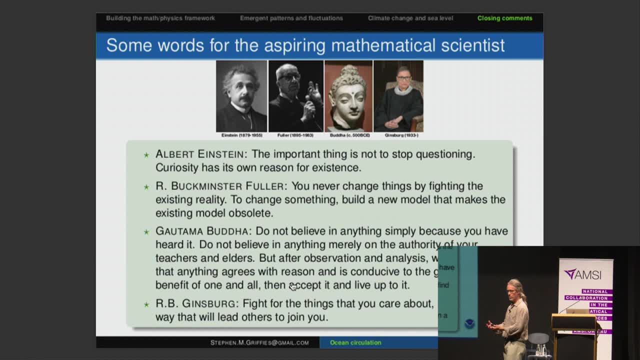 encounter people that don't understand, don't appreciate, don't like what you're doing. at some point, if you really believe in what you're doing, they're understanding. their approaches will become obsolete. make sure you stay healthy so you live long, and let the other people die before. 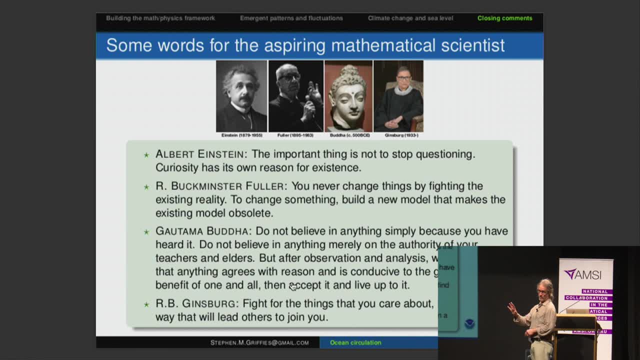 you die before you know. so let's you know a lot of. I think it was Bohr or somebody said: old theories never die until their inventors or till their proponents die. Buddha, This is a great one from Buddha. Don't believe anything simply because you heard it. Don't believe anything because of 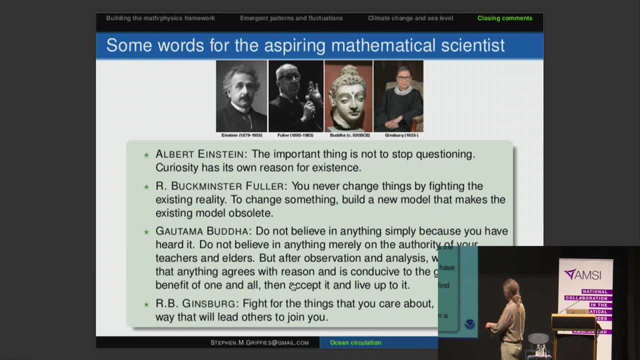 authority of teachers and elders, myself included, But after observation and analysis. when you find that anything agrees with reason and it's conducive to the good and benefit of all, then accept it and live up to it. So he was, of course, talking about the mind. He was a real, he was a mind scientist. 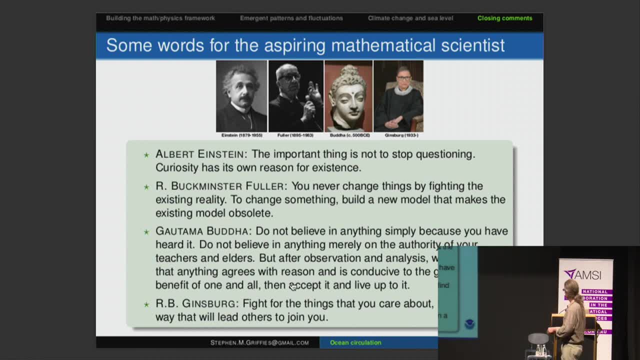 in many ways experiencing his own mind and figuring what was going on, But this has a lot of relevance to everything that we do in research. And then Ruth Bader Ginsburg, Supreme Court Justice of the US: fight for the things that you care about, but do it in a way that will lead others. 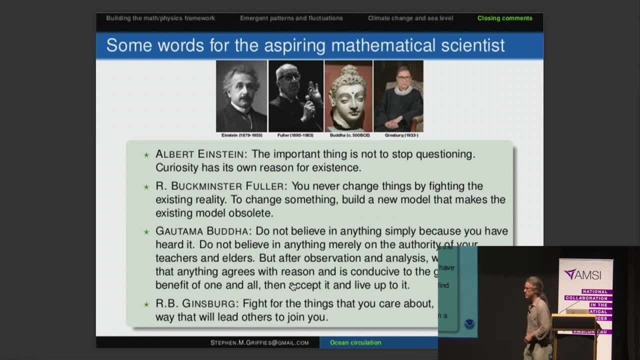 to join you, So be nice. basically, It helps. It really does. You can be a jerk and you will. eventually people won't hang out with you. It's very important to be able to work with others in this field and, in particular, in any field. 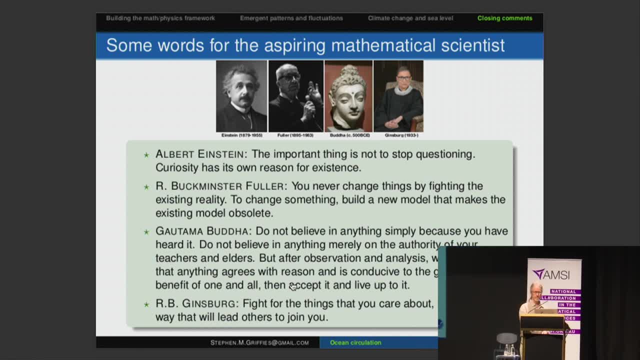 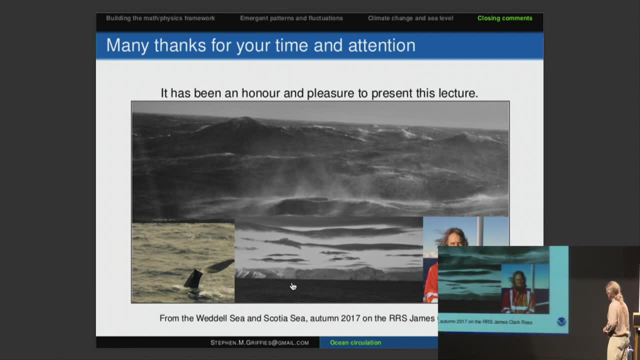 It's fun to have friends in your work, So thank you. It was an honor to give this lecture. It was fun putting it together. I had a lot of time while I was unemployed for the last month. This is an image from a trip I took- now almost two years ago- to the Southern Ocean. If you get into earth, 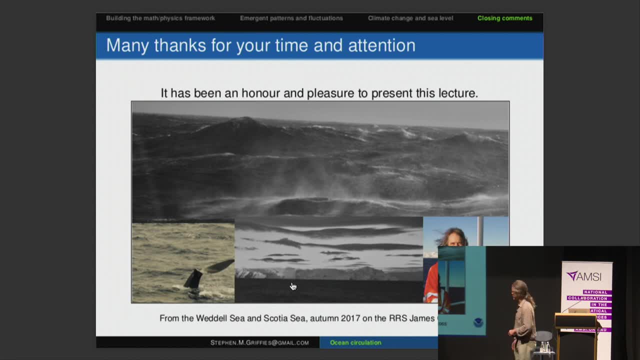 science, you will have the opportunity. even if you're a theorist or a modeler like myself, you will have opportunities to go to sea. This was a trip to the Southern Ocean, the Weddell Sea and the Scotia Sea- and the Atlantic sector. I went to the Southern Ocean. I went to the Southern Ocean. 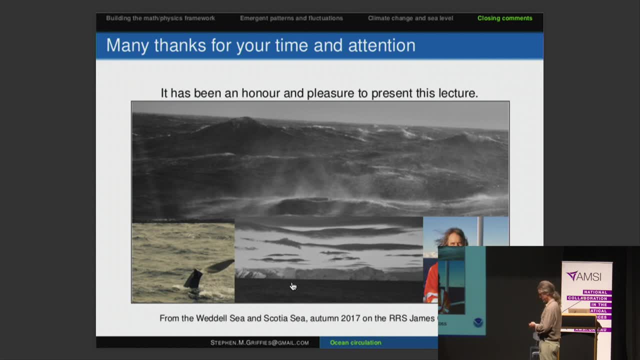 with a British ship. We stayed eight weeks down there. We saw some massive waves, A lot of my wave dynamics. people love this wave image. They show it in their talks. This is some gravity waves, or lee waves, going off of mountains off of this island in the South in the Scotia Sea. That's a whale. 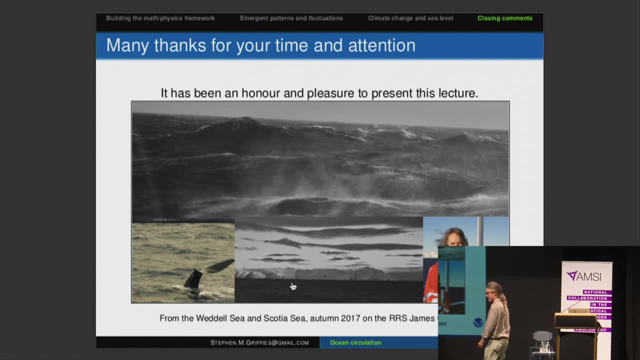 tail, and that's myself. So thank you. Okay, Thank you very much, Steven. That was an absolutely brilliant presentation. So how are we doing for time? You did brilliantly on time, by the way, So we actually have time for some questions, So is 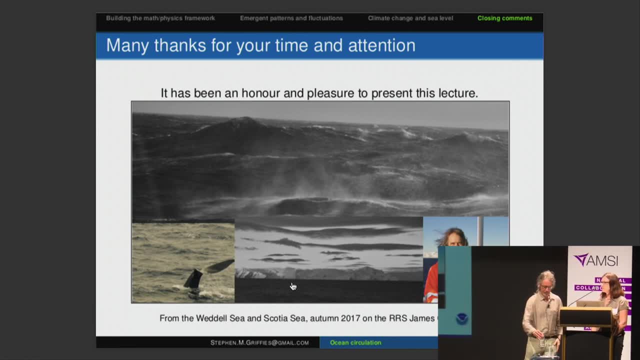 there anyone in the audience who would like to ask Steven some questions? So the first person to ask a question gets a prize. Oh, I might ask the first question. The first person who's not a faculty member at any university. the prize is. 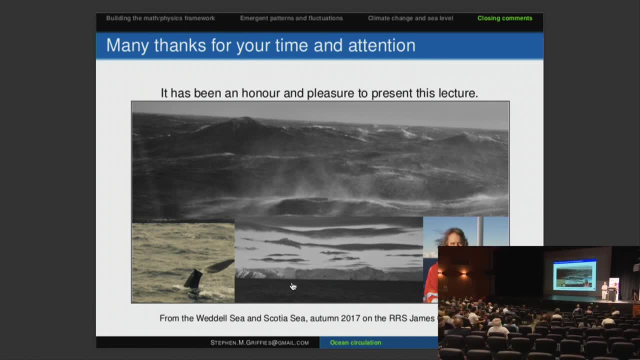 Okay, I know it's hard to be the first questioner. Oh, we have a first question. Beautiful, Okay, Excellent. Stephanie Downs, you're not a student? Okay, You need a microphone. Thank you for that great lecture. I just wanted to ask: do you think that the Global Ocean? 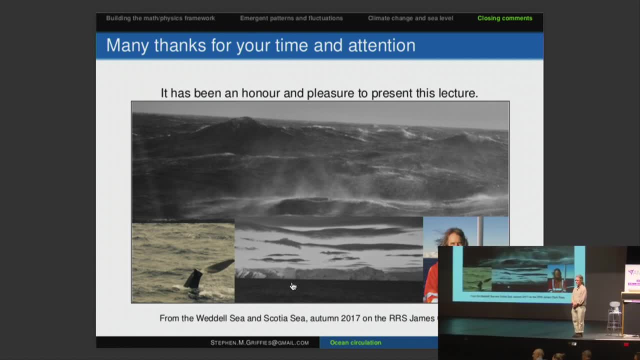 ocean general circulation models are good at capturing extremes in the ocean, like marine heat waves. Yeah, so marine heat wave studies. there's a lot of extreme studies going on in parts of the world and looking at heat waves, in particular the actually the simulations that we show the CM. 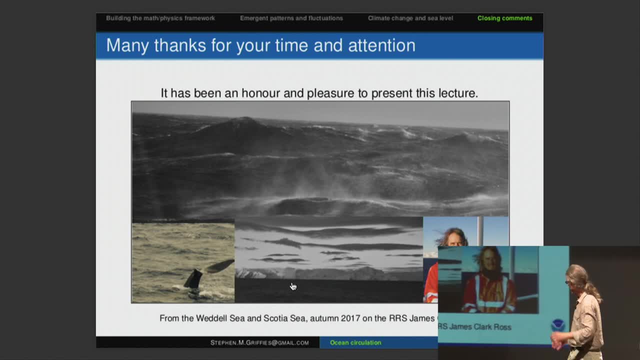 2.6 GFDL simulations that I showed some of the movies from do a reasonably good job of marine heat waves. The models that are coarser and less highly resolved, they don't do the marine heat waves, at least as far as we can tell. I'm doing some work with Thomas Froelicher. 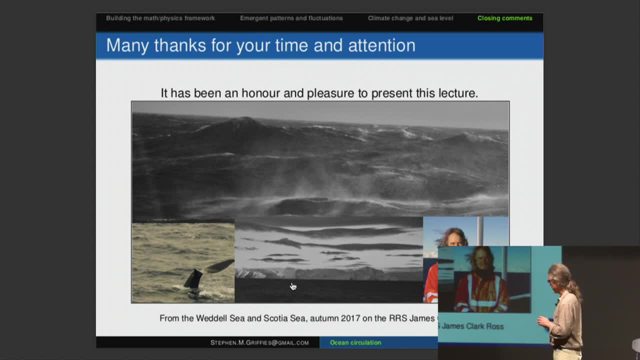 in Switzerland and other people looking at that, and everybody's very keen about these high resolution models, the models you can run globally at, say, 10 kilometers, 5 kilometers, and get the coastal. a lot of the marine heat waves are on the coast or near the coast. those are the ones that really 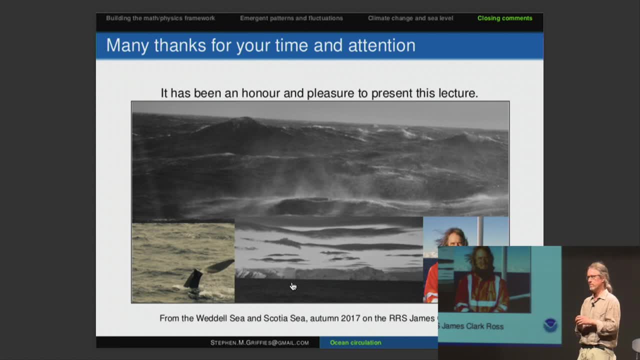 affect the fisheries that we care about and you have to have the model. if you have a 100 kilometer grid box versus a 5 or 10 kilometer grid box, it makes a big difference to the coast. So, no, I don't think that we're doing extremely well with some of the 1 degree. 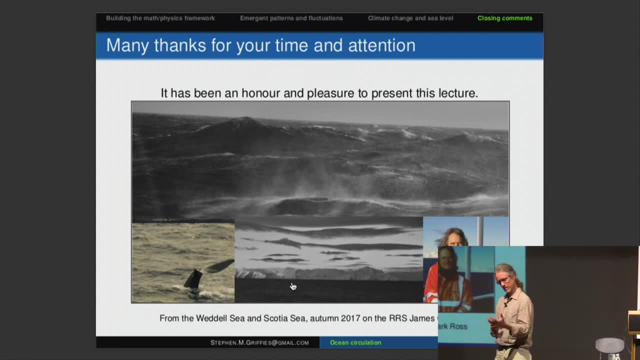 or 100 kilometer models, but they're given a hint, but you need to go to higher resolution. So this is a plug for more compute power, more funding for big computers, because if you really want to do good climate science, that has a statement about what's happening. 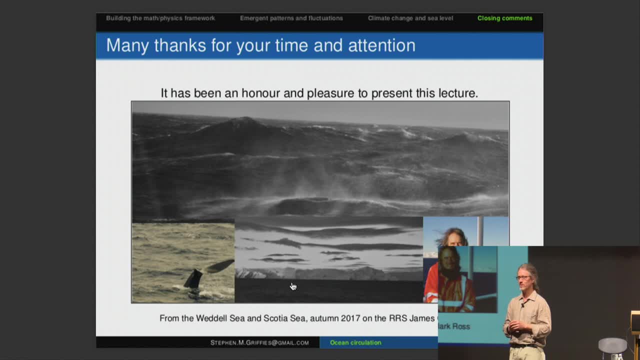 off the shore of your city or your town or your country. you really need a higher resolution. We're moving in that direction, but it's often difficult to get the compute power. There's a good rule that no matter how big a computer you'll have the climate. 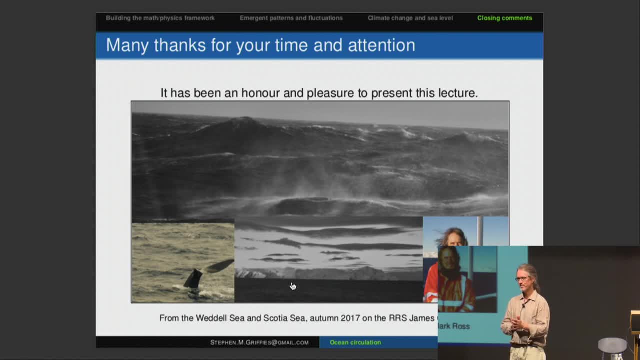 scientist will soon fill that machine. Because of this many cascades. the phenomena just get more and more rich as you go to higher and finer resolution. I think we want to have a microphone so it can be recorded, So you're recorded with your questions, by the way. 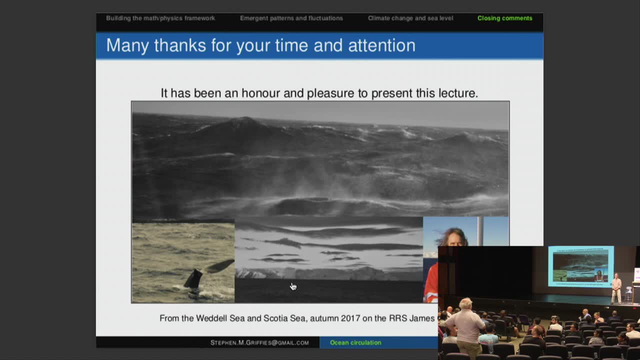 Russell Morrison from the School of Maths. Now the microphones come on. So you were talking largely about about the ocean models, but obviously the entire geophysical system is coupled And so everything's sort of going today towards more fully coupled system. 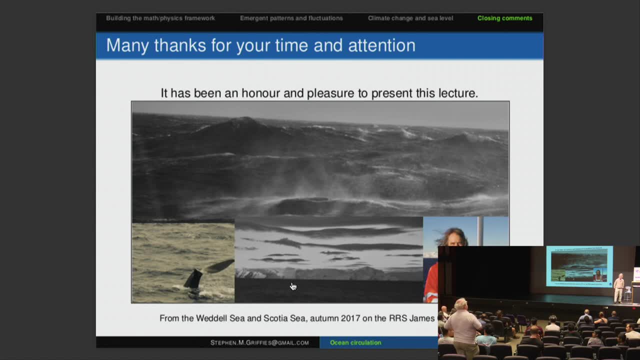 the atmosphere, ocean, terrestrial, all that together. So where do you see things going in the next 10 years in terms of model development and what we're going to be able to simulate with that? So there isthere are a couple of axes. When you have a computer and you 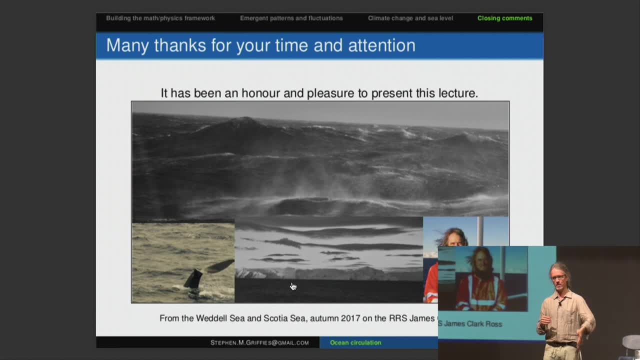 know you can fill it with different mathdifferent means. you can add complexity by adding more and more stuff. You canI mean the climate models that we are running now at GFDL- have a hundred chemical species in the atmosphere, 40 chemical species in the ocean. and then you start to say: well, my 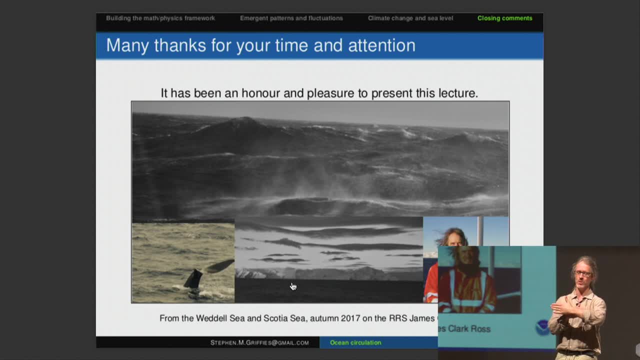 other axis is resolution. How fine do I want my resolution to be to represent some of the physics that I talked about here, And so we have to compromise on that resolution. And the other axis is numberlength of simulation and number of members of an ensemble. You typically want to have more than oneyou want to. 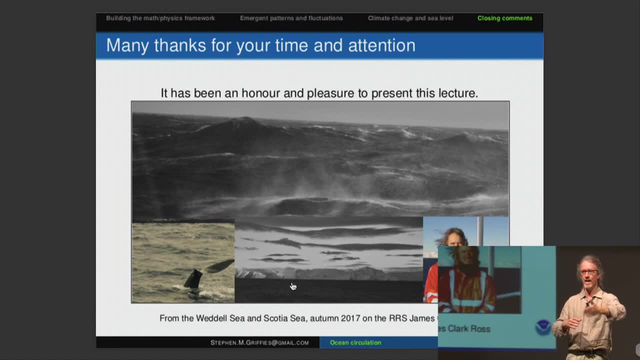 build an ensemble of simulations, So those different axesand also then you can assimilate. if you want to do prediction, You have an assimilation scheme. So the development is tryingat GFjust talking personally about my lab, we're trying our best to do a bit of all of that. We have different groups of 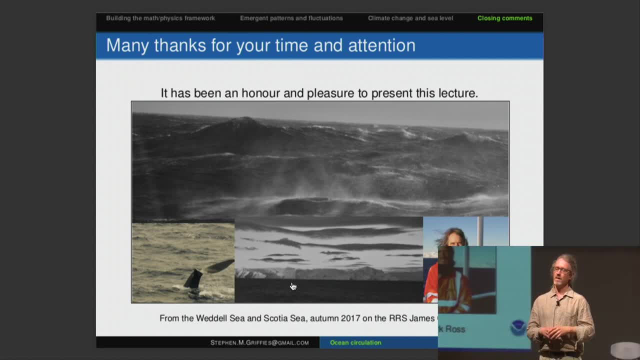 people that have different focus of theirof their work. and then you, every few years, when you start to say, well, it's time to build a new model, then you get everybody in a room and you shut the doors and you argue about what's the. 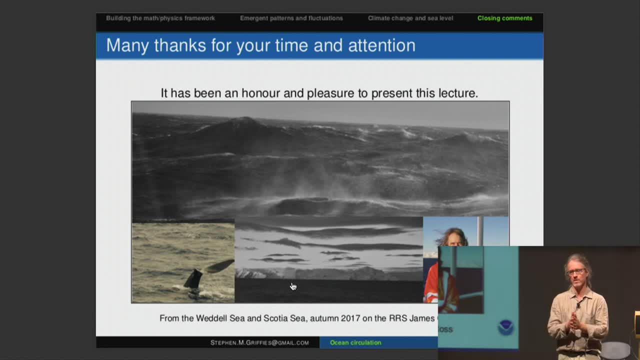 most important thing for the next generation model, And it's not always a it's a compromise you have to reach at some level. So, in answer to your question, I think it's enhancedeverything is moving upward, in a sense of enhanced resolution, enhanced complexity. I mean, I have my preference, I'm more interested. 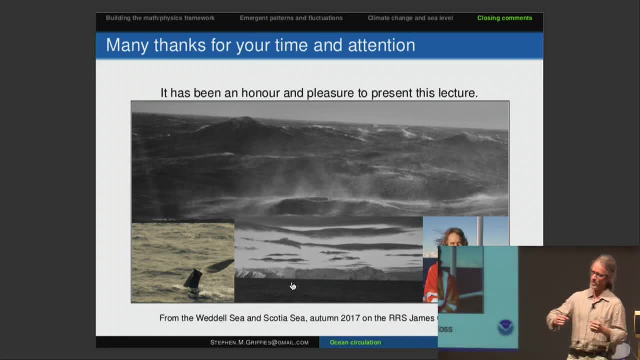 in the physics of the ocean. So resolution is what I want, but my biogeochemical friends want more biology and more species. So how it's moving forward, it'sI mean there's lots of numerical methods that are still being put to help advance the ocean physics. 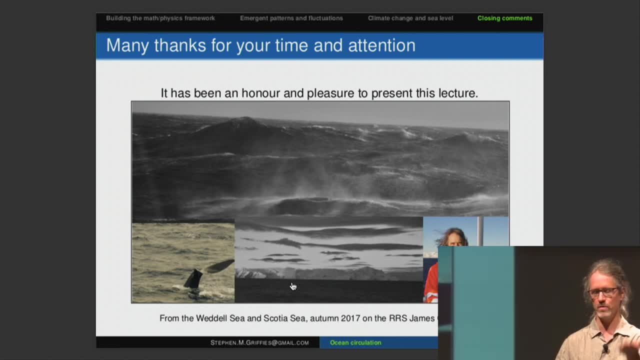 simulations, And one of that method is the representation of the vertical direction, the buoyancy field, in the vertical structure, And there's different verticalthe vertical direction is a very important direction in the ocean, as well as horizontal, But the vertical is distinct because you have gravity And 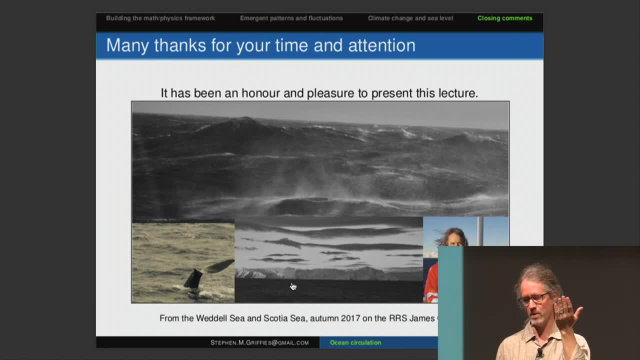 the representation of the vertical coordinate in our ocean models and the atmospheric models is being generalized in a way that 10 years ago was not done, And it'swe're using methods called arbitrary, Lagrangian or Eulerian methods, AL. And that took a bit of work, a lot of work. I mean the engineers and the 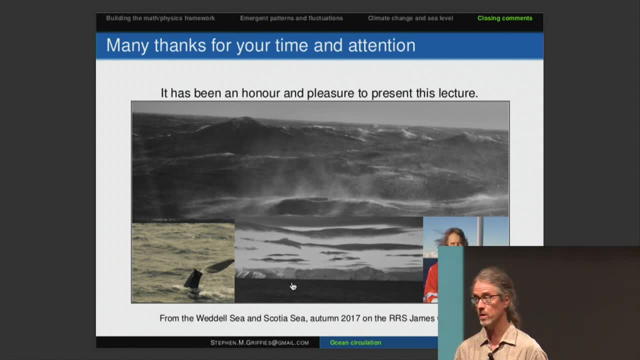 applied math. people at Los Alamos did this in the 60s. What's the big deal? Well, it'sthe ocean is a very complicated structure, very complex structure, and it's structured buoyancy. stratified fluid with that buoyancy variable is a complicated 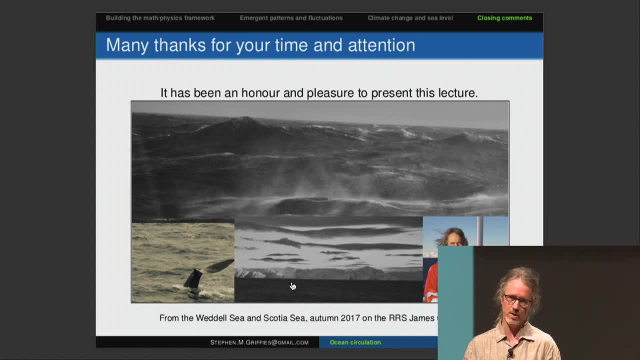 field. You have salinity and temperature creating differences in the buoyancy field that make it very complicated to do a very straightforward, fluid computational physics problem. It's not straightforward. That's amaybe a more specific example of moving forward. It's the AL approach, Also in the 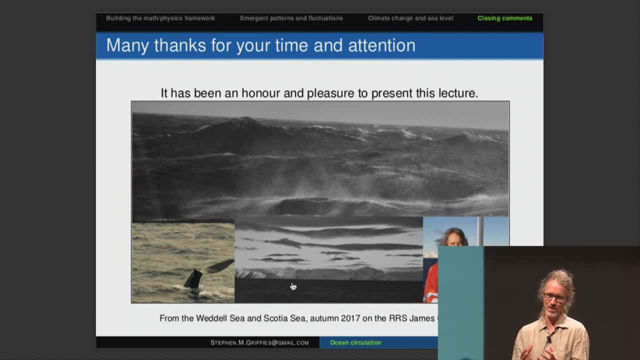 horizontal we are movingsome. groups are moving toward unstructured grids, The finite element or the finite volume. unstructured grids are moving toward unstructured the acosahedral grids and things like that, And so the sophistication of the computer models is moving forward in a way that maybe 10. 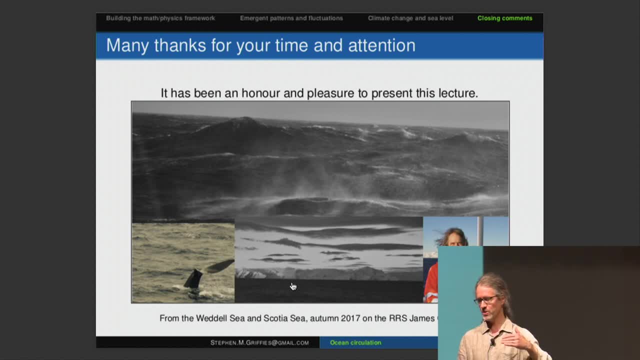 years ago- wasmaybe even less than 10 years ago- was just a pie in the sky, But we're starting to make headway at making real models from these things. But just remember: these models are massive pieces of software that take teams of people a. 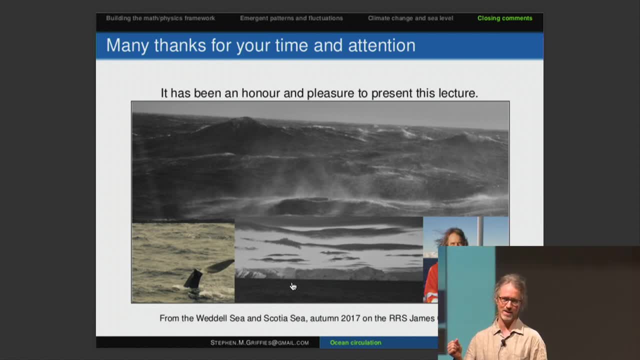 generation to build, And so just to say: you have a new idea, let's change everything. it's slow, It's very slow for people that are used to these. let's have a new idea and just generate a new model from it. 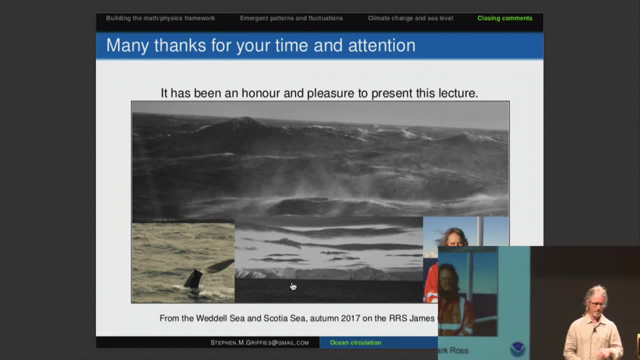 We have a question over here. I don't know if I'm allowed to ask a question. Some of my mates are using machine learning to generate new models. I'd like to hear what you think about that. I wish I knew more about machine learning to have a good answer to that. 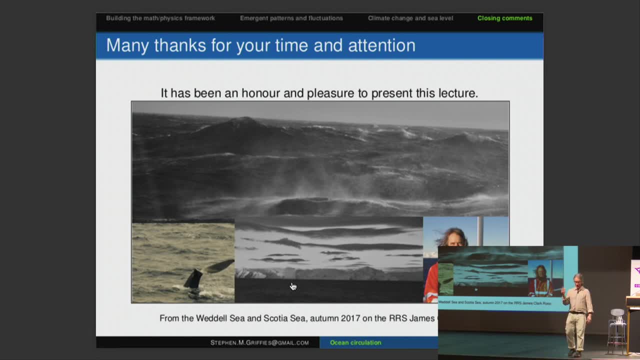 I have a colleague at Oxford who's actually moving to NYU in the year. Her name is Lozana and she is pioneering some work with machine learning for looking at the eddy parameterization problem. Now, you saw these eddies, these. 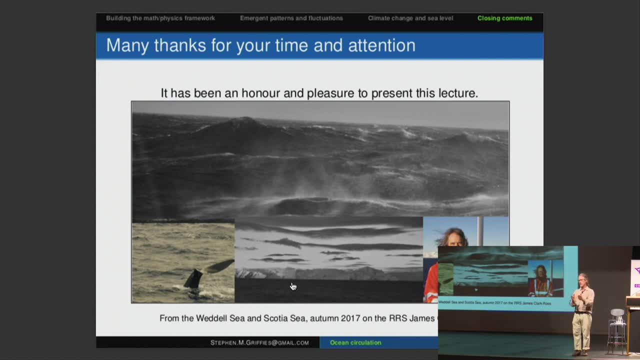 whirlpools and so forth. If you have a model that doesn't resolve those eddies, you parametrize them. Okay, And the methods we use to parametrize are often ad hoc and not really well thought through, although there are some very sophisticated methods out there. 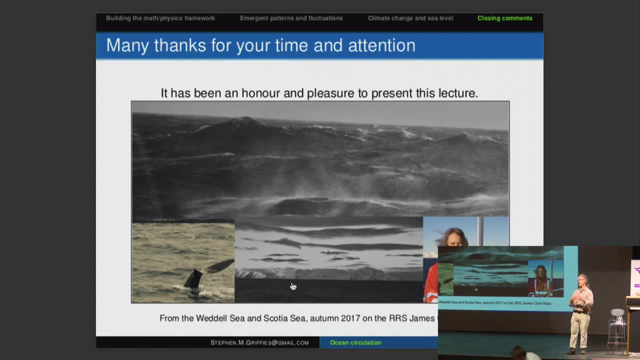 Machine learning to help inform those parametrizations, how you tune the parameters, how you find the parameters, is something that she's promoting and others as well. I don't think, and neither does she, that it is an elixir. It's going to solve all of our problems. It's not a black 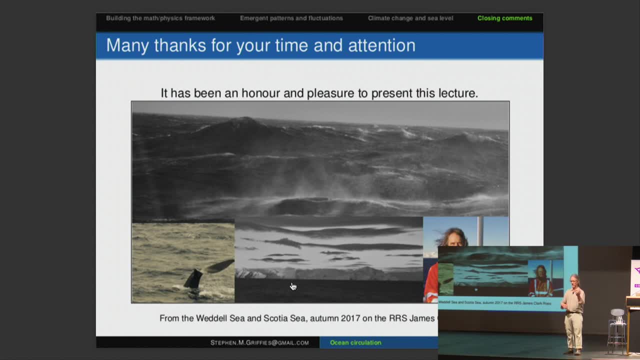 box, And so having it be something that you can open the hood and look inside the machine learning algorithm is very important. We're still gonna- I think we're still gonna- need the some the numerical simulations based on Navier-Stokes. We're not gonna go to machine learning climate. 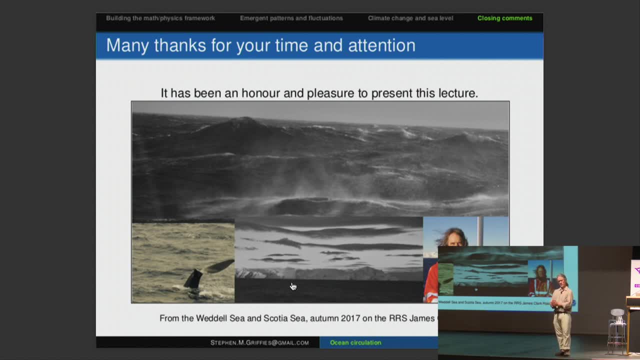 models. We're gonna still have dynamical foundations to our models. That's a prejudice that I have, and maybe I'm gonna be wrong. in 50 years, we'll have something that's not based on fluid mechanics. We'll have something based on. 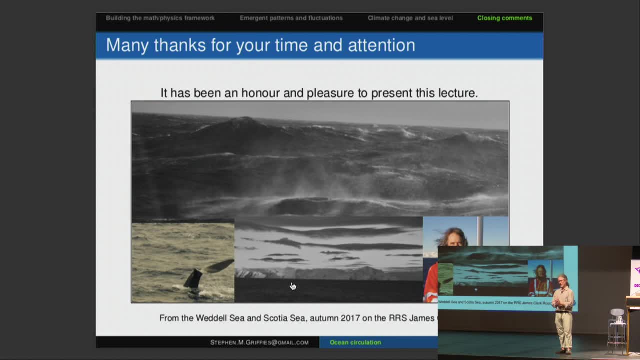 something else, but it will definitely be informed by fluid mechanics. if it's gonna be something that is very important, that is useful to the ocean. We have one here and then over here. So here first. Hello, I'm Eric Hester, a PhD student. 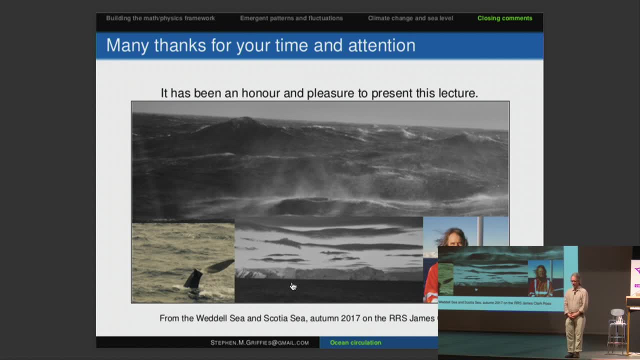 at the University of Sydney and I have a question somewhat similar but maybe broader than the second, which is: what are the general new frontiers to explore in geophysical fluid dynamics? Are there new theoretical problems that we need to understand? Is it really how different things? 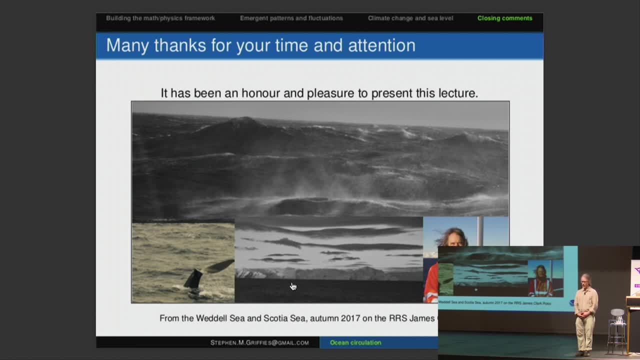 we already know, interlink, or is it numerics that we need to worry about, And where do you think a new scientist in this field should best focus their efforts? So the answer to that is a big answer and I'm gonna try to fine tune it. 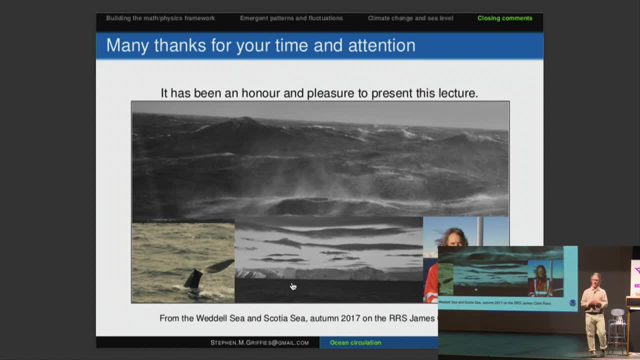 whittle it down. That's a big question. So, insofar as the geophysical fluid mechanics or geophysical fluid dynamics- I like to call it mechanics because we're talking kinematics and dynamics when we're doing fluid mechanics- The GFM or GFD questions. 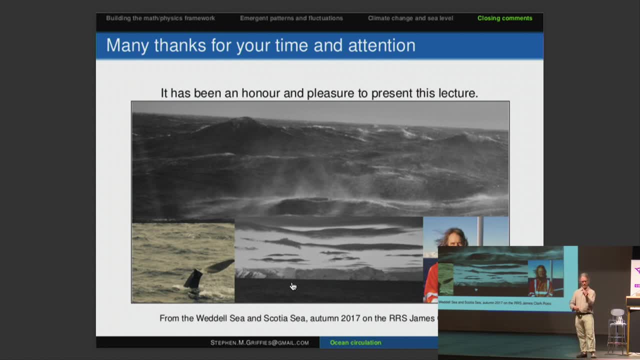 the scale interactions all the way down from the gravity wave to sub-mesoscale- not hydrostatic gravity waves, sub-mesoscale, mesoscale, large scale. The interaction between these scales is still a rich problem. These eddies generate waves. 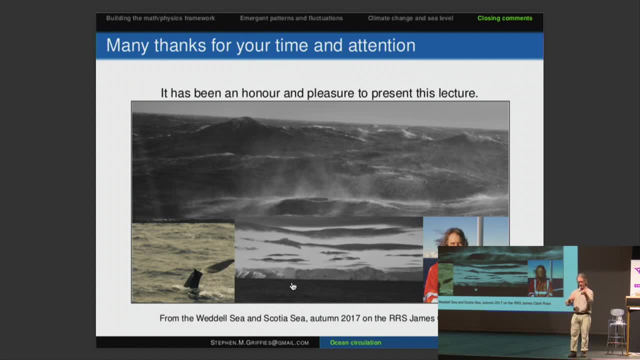 How do the waves- how do they generate waves- Break apart the eddies of the sub-mesoscale filaments and the instabilities that are created on the eddies, How do they affect the integrity of the big eddy itself? 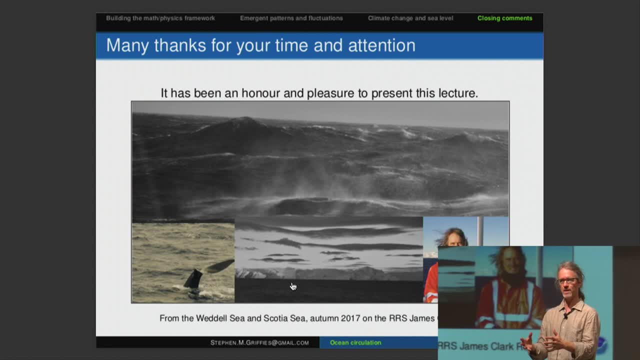 And those problems both involve numerical and theoretical analysis. And how we do the multi-scale problem still is a difficult thing And how we parametrize is still a very fundamental. it's the turbulence closure problem in many different ways because of that zoo, Each piece of turbulence. 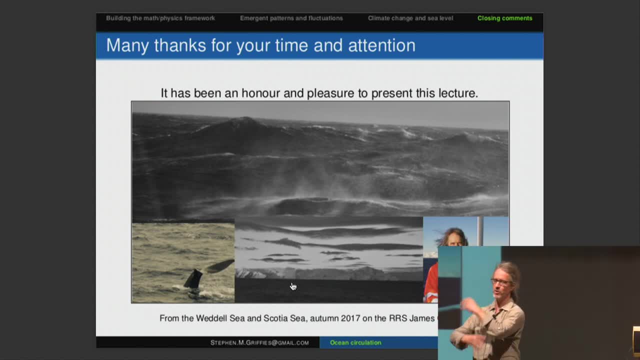 is a slightly different phenomenology. It's not just one three-dimensional homogeneous turbulence like Batchelor and others and Karl McGraw have thought about. There are different turbulent features in the ocean and you have some that are wavy, You have nonlinear waves or you have stochastic waves. 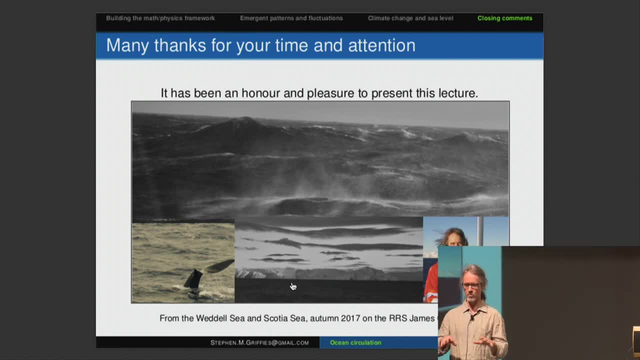 So there's a lot of rich geophysical fluid mechanics problems. related to the parametrization question. You have stochastic methods. You have fundamental GFD questions. From the numeric side, there is better numerical solvers and more friendly solvers. There's a lot of things that you can do. 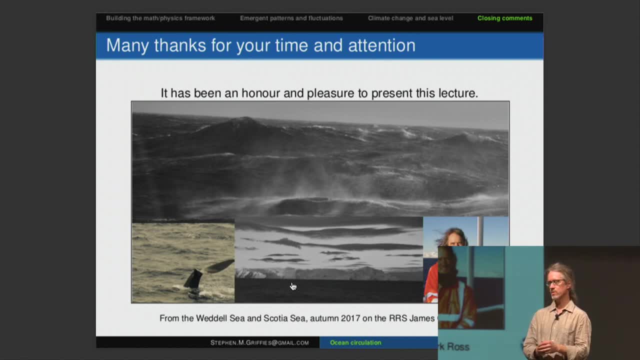 that you don't have to do anymore. You don't have to do the numericals anymore, So there's some freedom in that. but I also think it's important for a student to have some exposure to numerical methods so you know what's going on under the hood. 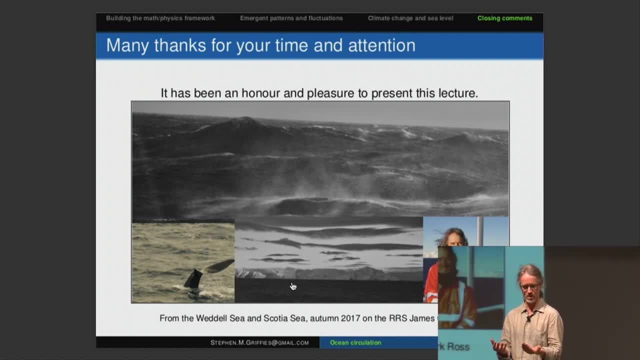 and so you can contribute to projects like Daedalus. It's not a black box, because in my experience, any time you deal with a black box it's going to bite you in the butt at some point. You're going to have a question. you don't know how to ask. 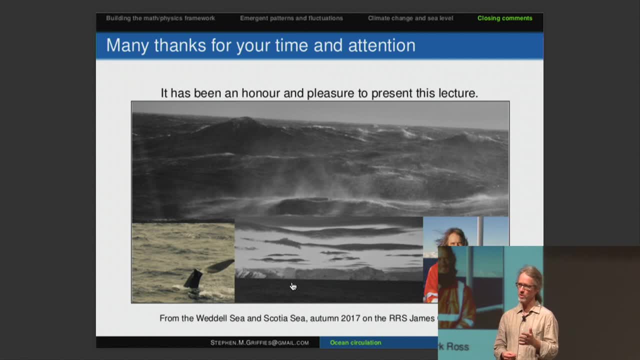 answer with that tool, but you're going to be able to answer it, Or the tool's going to have a bug and you don't know what's going on. The thing about fluid mechanics simulations is a bug can look like an interesting piece of physics. 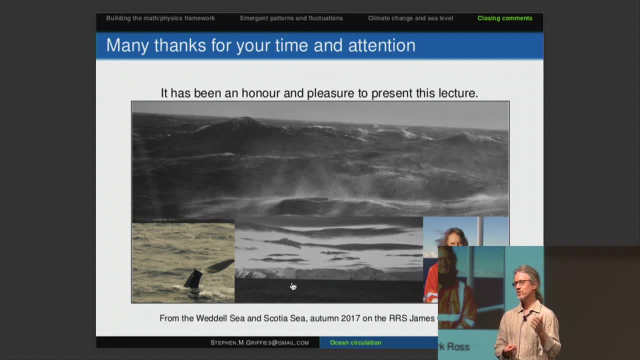 and you can go down a rabbit hole, and so you have to start developing your understanding and your experience and your trust of this tool. That's a big thing to understand. when you're doing this, You can't just be a take-it-off-the-shelf-and-do-it. 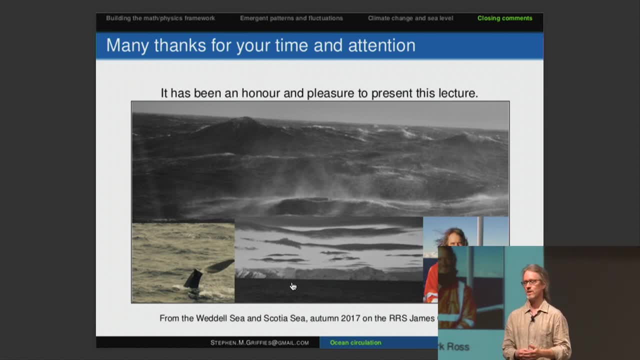 We're not there yet. These tools are tools that are imperfect and have many different things that you need to scrutinize. You can't trust. You have to trust but verify at some level. Talk to your colleagues, Become part of a community. 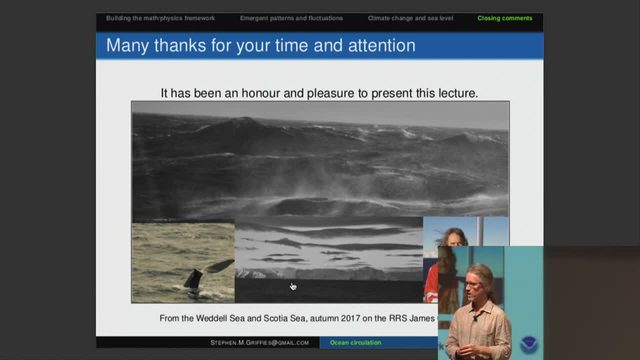 These open-source, open-access, open-development projects are really the way to go in my mind, because the days where you have one or two guys sitting in a room by themselves building their models and asking the world to trust those simulations is gone When I came in the field. 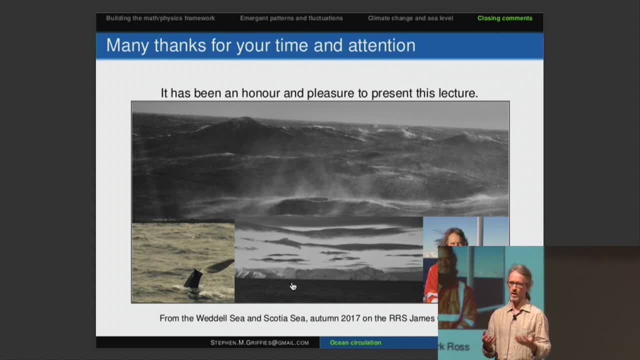 it was just a handful of people doing that and they were brilliant and worked hard and they did some great work, but it was not reproducible science. We need to do reproducible science now in our numerical models. You just can't. 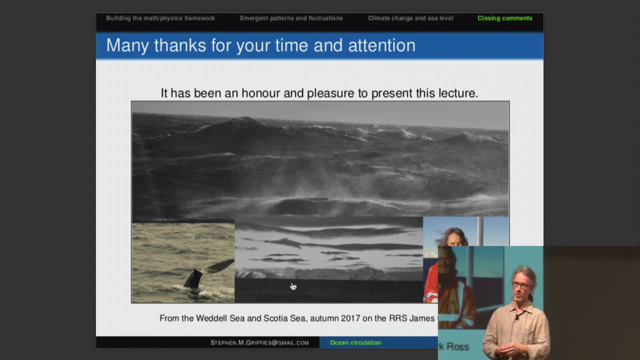 There's no way to argue anymore about it. So I don't know if that gave you some sense, but I mentioned some of the cutting-edge numerical methods. If you're a numerical person, there's cutting-edge numerical questions out there. If you're a physics, fluid mechanics person, 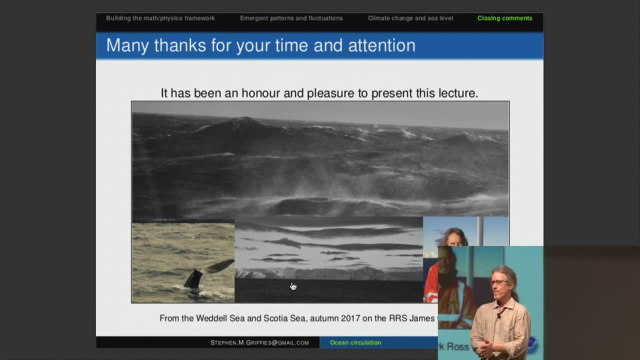 there's cutting-edge questions there too. Thanks for the response. Okay, My name is Songpin Zhu. I'm from University of Wollongong. Raise your hand, Oh, here, here. Okay, thank you. And given that the model has already been so complicated, 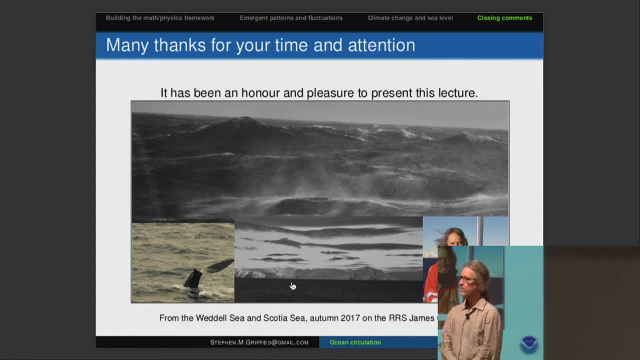 as you said. my question is: how are these models calibrated and validated? Yeah, so very good question. So philosophical response to the word validation: models are not truth and so validation. I would replace validation in every context with evaluate. So we evaluate our models by comparing it to data. 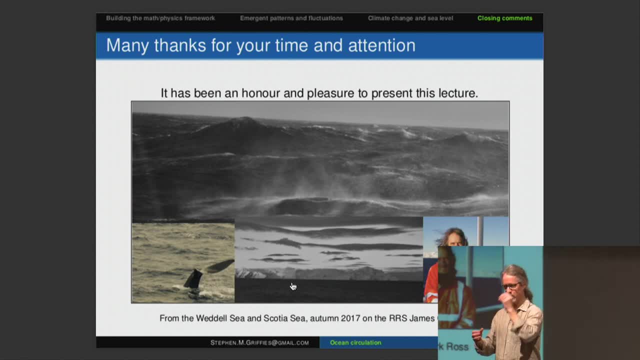 or our approximation of data based on satellites and observations and so forth. We have atlases, We have thousands of floats that are in the ocean that measure properties of the ocean on a day or a weekly time scale, And so we scrutinize these models based 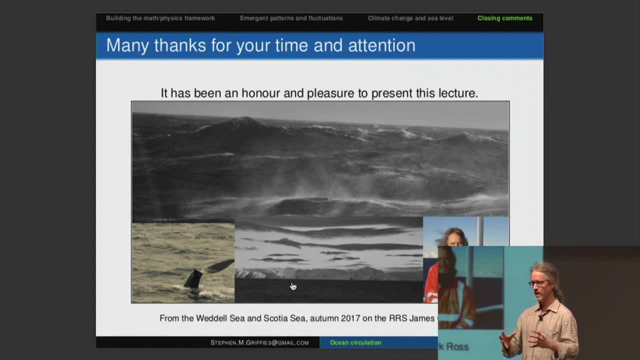 on the best observations that we've got, And the observational database is getting bigger and bigger in a very good way. So, and some of the models you know perform better than others And you get teams of people asking questions: Why does the model show a bias here? 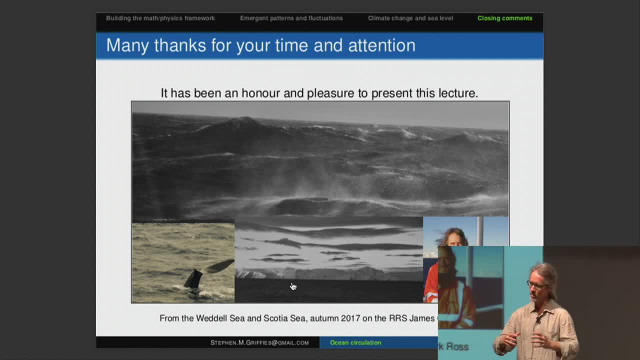 and other models show a bias there And you develop teams of people that compare models and you have model intercomparison projects and you develop ensembles of models whose mean is better than any individual model itself, because you're canceling errors and you're doing it in a way that's very useful. 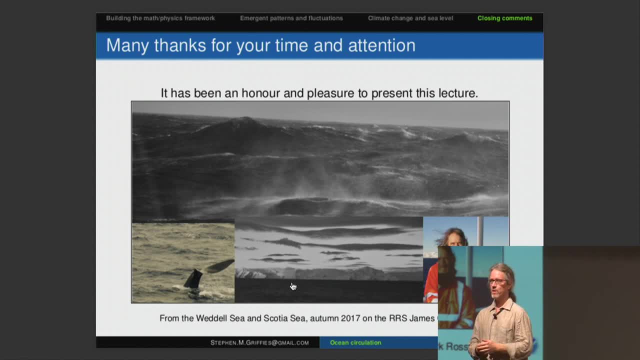 So that's how you evaluate the models. How you calibrate the models is partly due to evaluation. If you get a bias and then you say, well, let's change the parameterization to reduce that bias. So I like to use the term optimization of the model. 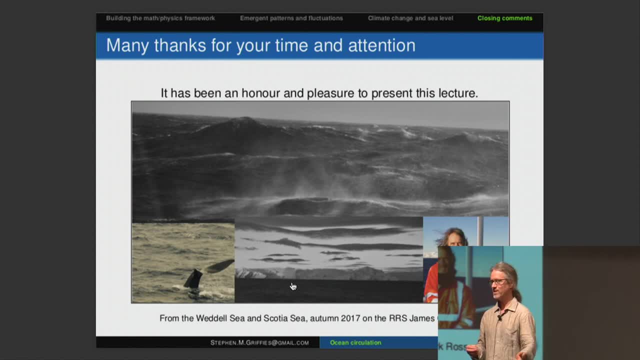 It's not something that you put into a steepest descent kind of optimization solver, but it is a process that's similar to optimization. Other people call it tuning, But that gives it a negative connotation in the sense you know, we're physicists. 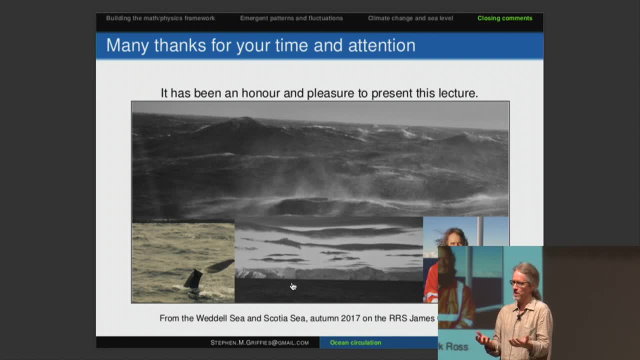 We're biologists, We're chemists. We're going to not look at a simulation that doesn't look like the real world. We want to change that simulation to look like the real world And so that spawns new research in the parameterizations. 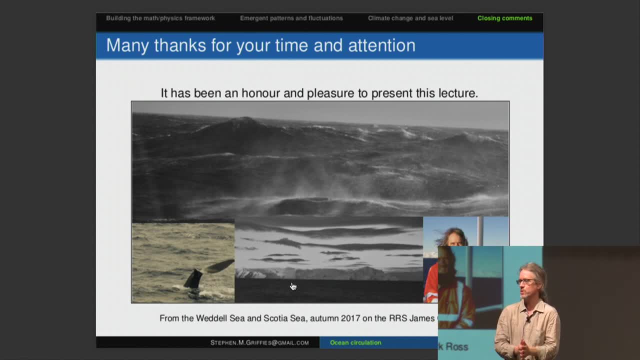 or refinements of our theories or our simulations to reduce the biases. And each stage, each generation of models, each 5 to 10 years, the generation of models is getting better and better and better And there's still lots of problems that are still there. 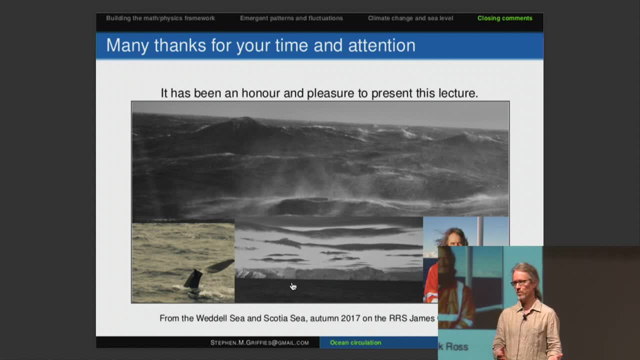 to be researched and understood, but we're definitely better than we were 40,, 50 years ago and even 10 years ago. It's an incremental process of building up the knowledge base and working from that foundation to do better and better and better with what we've got. 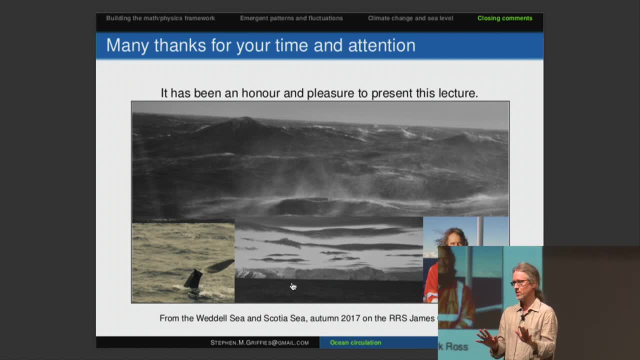 I'm not saying that it's perfect. I mean, if it was, then there wouldn't be much research left. But we know a lot about the system and how to do better than when we did 10 or 15 years ago, Or 10 or 15 or 20 years ago. 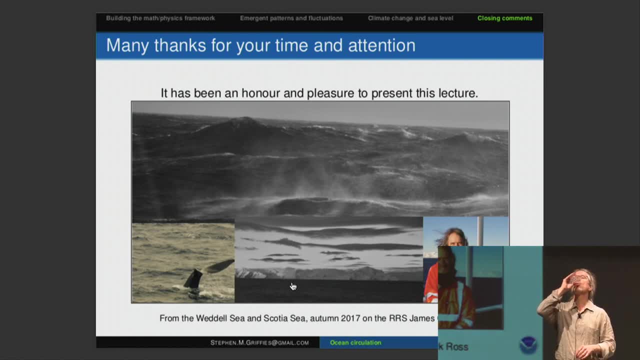 Do you have any other questions? Yes, one there. All right, Just following up a little bit what everybody had mentioned, a little bit about the computing power that used to simulate the models and like to predict and all So what's like the most promising current efforts. 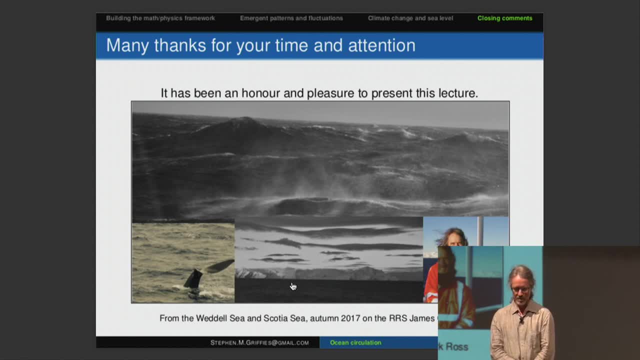 that to improve that computational model, to have more efficient computation for the models and prediction? Thanks, Yeah, so this is a good question for somebody else, but I will give you my shot Because I'm not a computer engineer or a person that even pays much attention to the computers anymore. 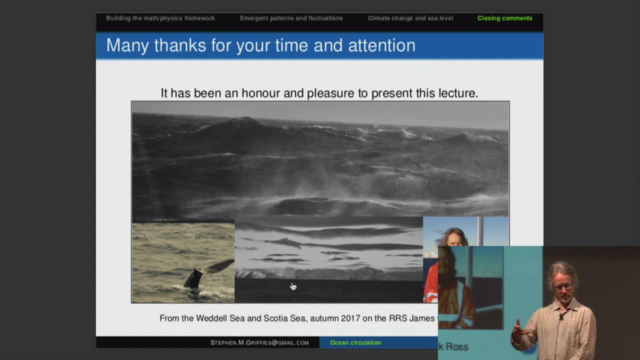 GPUs. does that ring a bell to you? The sort of tools that people use for computer games. That has taken over the industry quite a while, Quite a lot, And so there was some early- maybe 10 years ago- some indication that the climate modelers should pay attention. 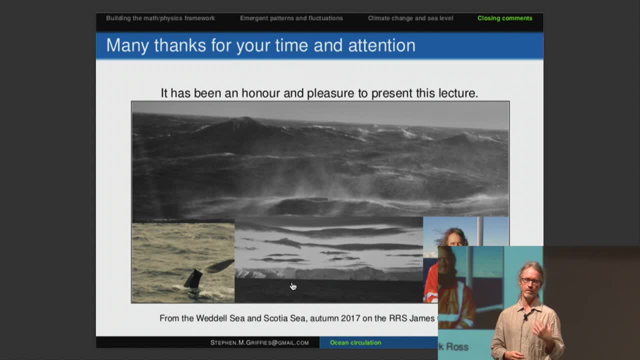 to that and should be developing our codes that could run efficiently on GPUs instead of CPUs. Some groups have taken that ball and run with it. Some groups just say let's be patient, Let's, because these are thousands, hundreds of, some millions of lines of code that you can't just. 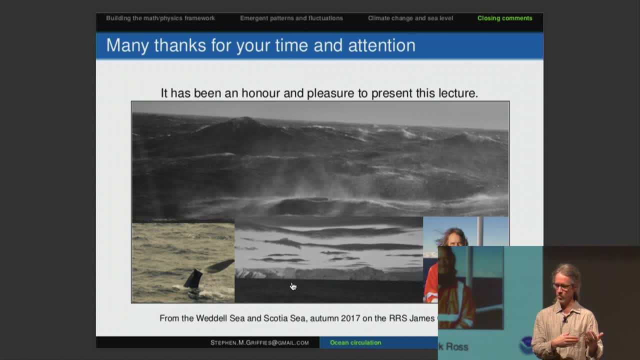 like I said earlier, you can't just turn on a switch and have them in a year work on completely different algorithms. So for many people it's an overly conservative computer science problem. And if our computer models jumped at every new idea that comes out of the computer science world? 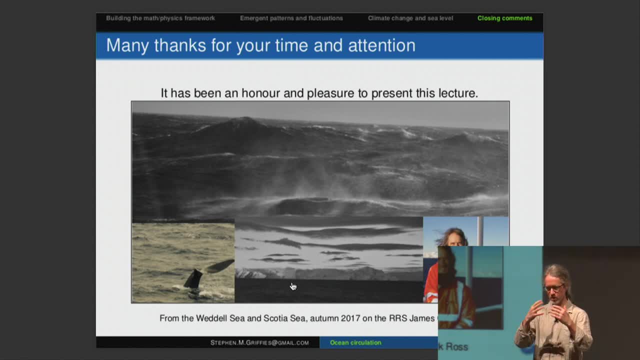 then we would never do any simulations to the degree that would allow for us to trust what we've got, Because every time you change a code, you have to worry about bugs, And so you have to do things, you have to do lots of testing. 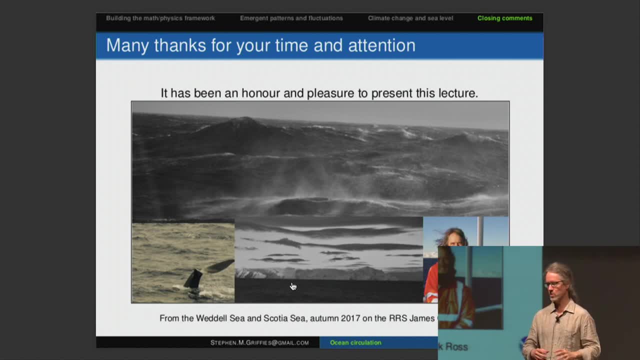 as you go forward with these compute codes. Having said that, there's groups in the UK that have said: let's start from scratch, Let's do this again and let's build based on GPUs or let's build based on other ideas. There's a group at Caltech that's building, I think. 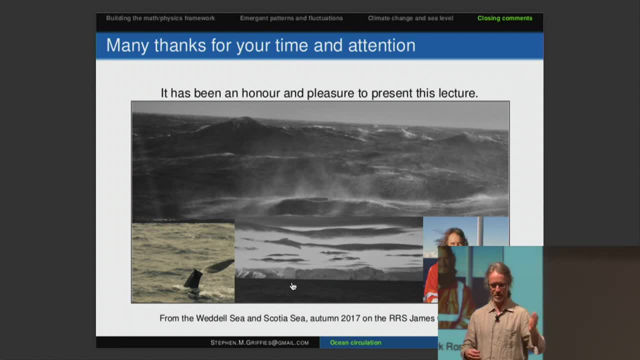 a new model based on Julia instead of Fortran. Julia is a software language And there's groups that are working with these icosahedrals, these other approaches, And every time they build, when you start fresh, you start with the hardware in mind to make the software work. 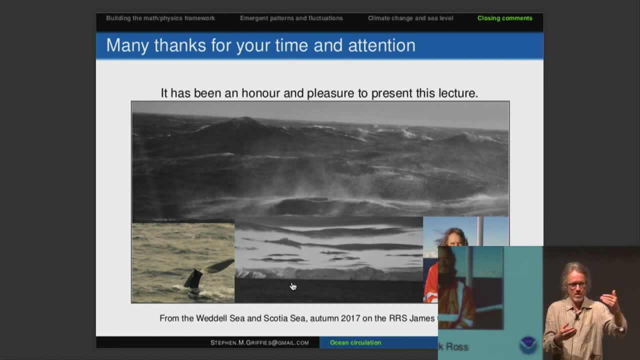 well with that hardware, And so the problem with that, of course, is that the hardware changes And you have software based on these many thousands of lines of code that has to catch up. So you have the physical scientists over here that want to simulate, want to look at the patterns. 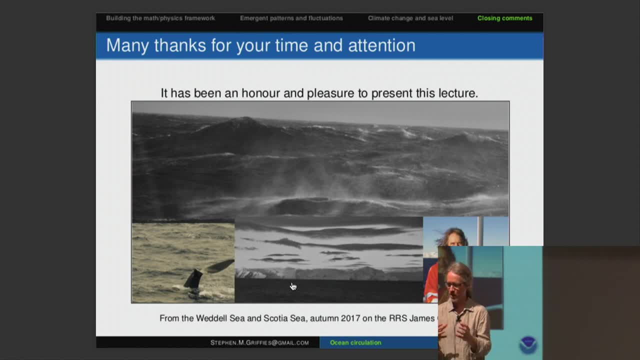 and want to do so with a code that they're used to working with, that they can trust, And whereas the modeling people or the compute people over here say, no, go to this thing, And then you go to that thing, and then you start working with it. 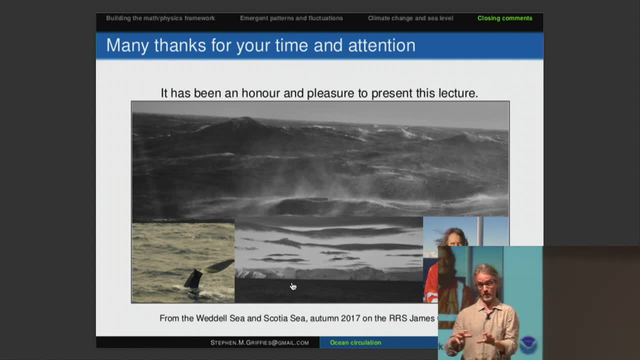 then they're up here again. So it's a very difficult situation at times where you have an interplay between these groups. But it works and you know it is what it is. It has to move forward at some level. We can't stay in Fortran 5 like we were in the 60s, right? 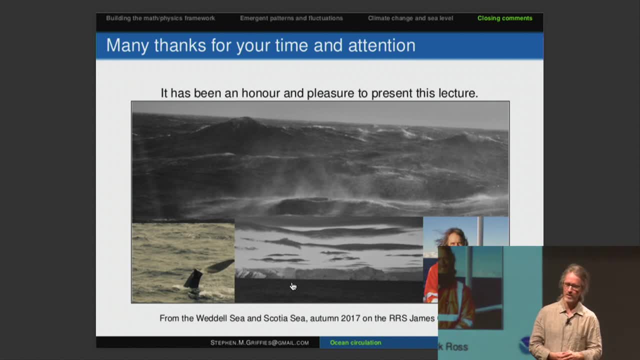 Watt 5, which is what I learned when I did did compute. But we're still working with Fortran for the most part and some of the big centers. We're not even using C or other codes, But you know, it's like Fortran looks more like C every day. 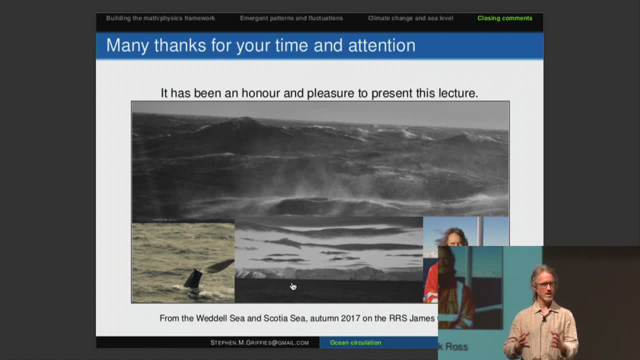 So it doesn't really matter that much. So I didn't give you a very, very coherent answer. I apologize, But there is a lot of compute people that are working with us that are being mindful of the new technologies that's coming out. 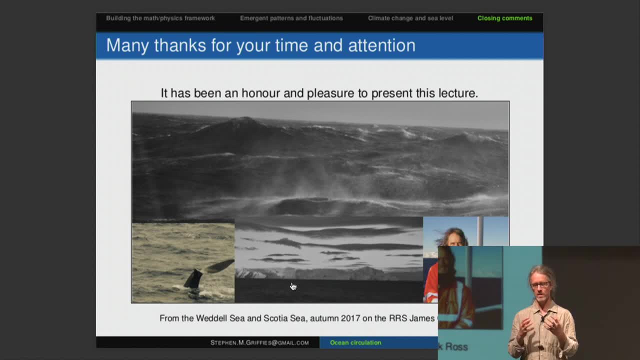 And somebody like me that just wants to have a code that I can trust. I'm very resistant at times to just going after the latest trend, because it can change. It doesn't always pan out, So we have to be like a step behind the latest trend. 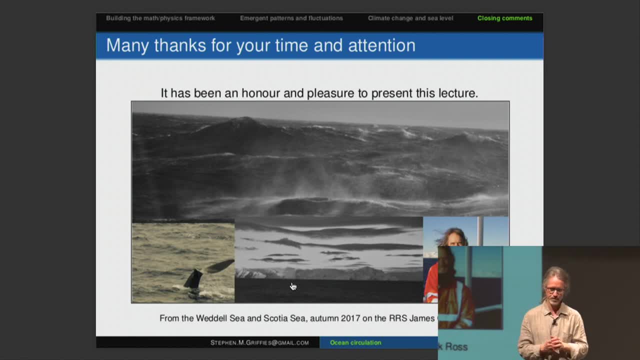 to really see what's robust from the hardware side. Okay, We maybe have time for one very quick question. if anyone. Quick question, long answer, That's what I would do. Yeah, Well, maybe I have a bit of a more. 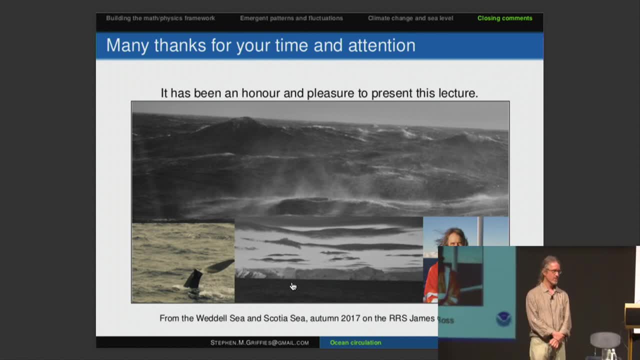 more pedagogical question for you, given that we're at the AMSI summer school. You're obviously quite passionate about teaching mathematical sciences, But we hear more and more about how fewer and fewer people are interested. What's your take on how we get more people interested in this area? 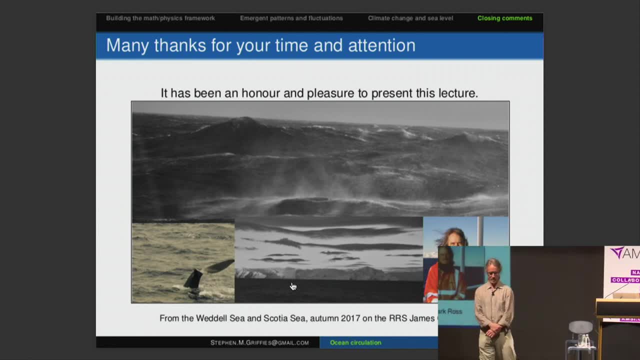 Yeah, So I teach in a geosciences department And I teach fluid mechanics in the geosciences department, And so the best- and I teach graduate geophysical fluid mechanics- The best students are the students that come through the engineering, math and physics. 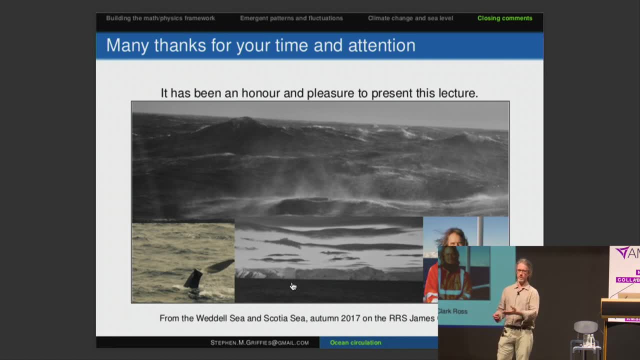 not from the geoscience undergraduates. So if you want to do the theoretical modeling work, this is the audience. This is one of the reasons I said yeah, I want to give this talk Because I want to turn on some of you all. 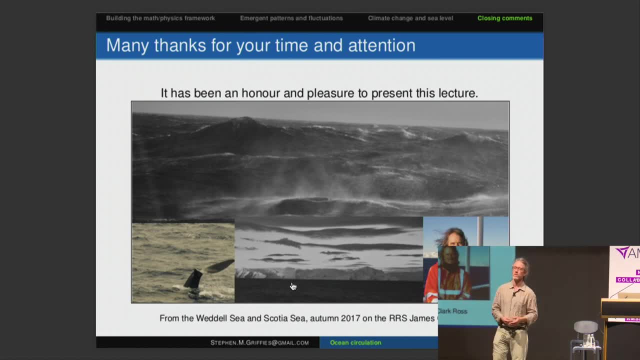 to the interesting fluid mechanics and mathematical physics in this field And so you can work in a geophysical department, geosciences department, and do interesting math physics. How do we get more of you in this field is really your question. I don't know. 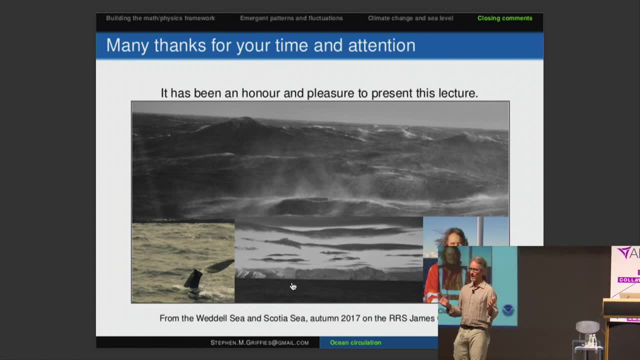 Maybe more of us out there have to say it's cool to know math. I mean it's. and there's also a gender bias, right, I think you know it's not. I mean, there's some of the best. 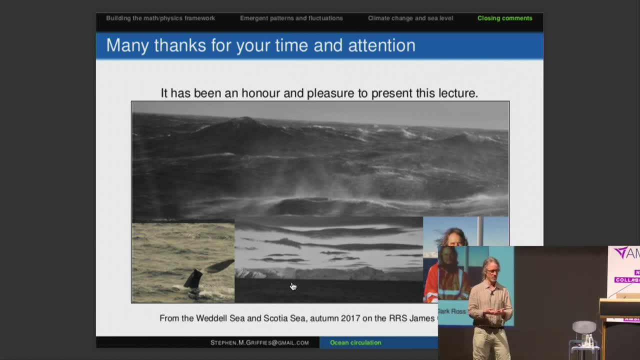 My son is 12 and some of his colleagues are smart girls, But at some level there's a falling away of that. Why is that? Why don't we have more? Why don't we have more Lisa Alexanders in our field? I think that's changing. 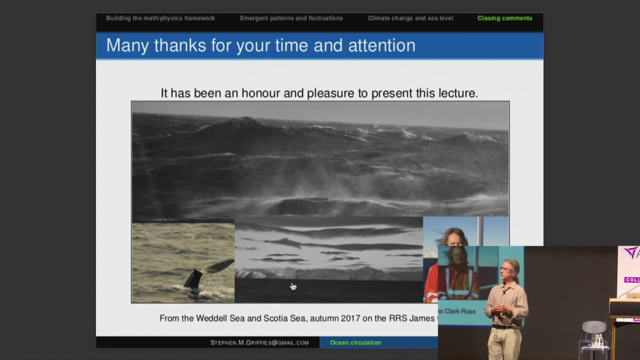 It's. we're doing good at that, But how do you get more math? The other thing that I have to. I don't have a good answer. The other thing that I want to emphasize is that this is still a quantitative field. 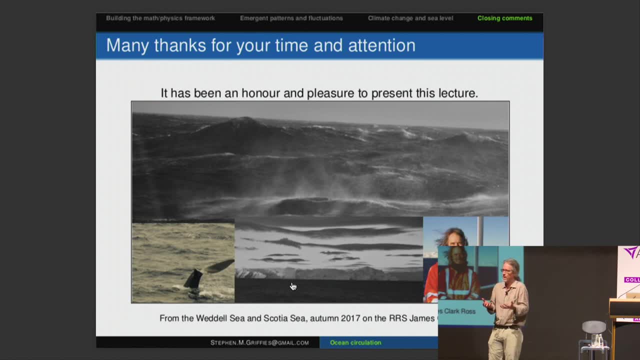 It's becoming more and more quantitative. We need more and more strong mathematical foundations for what we do. It's not something that you can just take off the shelf, yet It's not a turn, the key kind of problem. There's still lots of very difficult math questions. 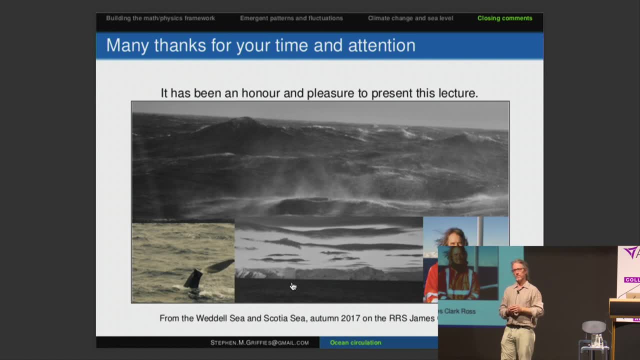 that are involved, And I think that's what's happening in the science and in the earth sciences. It's cool to know math. I don't know It's, it's, it's. there's lots of cool things in math. 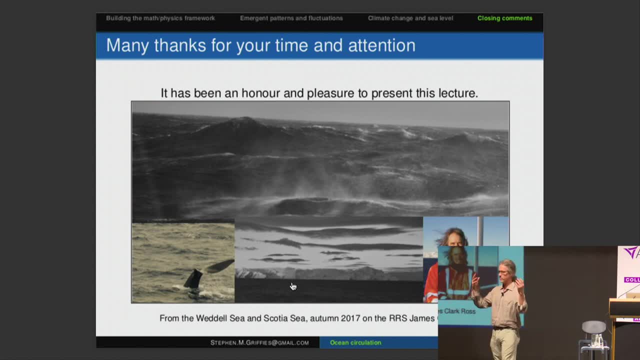 You know, I mean you could have somebody doing pure math, topological, algebraic topology, and give a cool talk. I looked at online at one of the earlier lectures and this was the glass bead game lecture And this guy was talking about all this stuff. 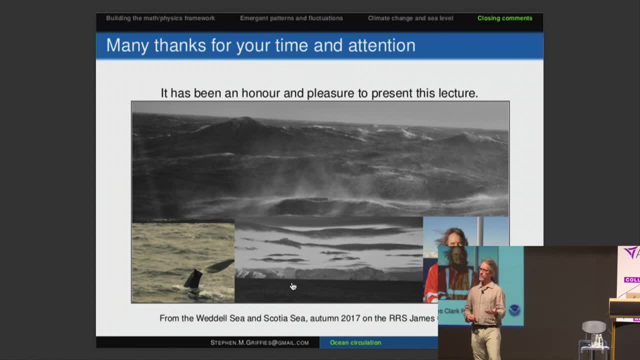 And the students in the audience was pure math. There's a. there's a professor in Princeton. He's an Indian guy, Won the Fields Medal. I don't know his name, He's. he's like: Yeah, He just gives the best talks.